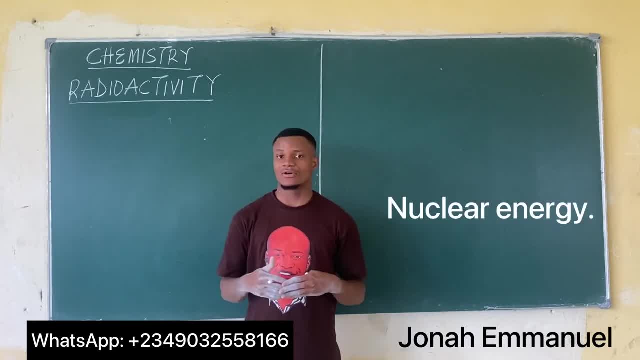 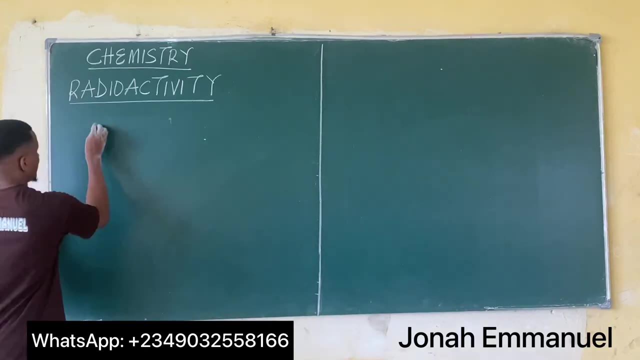 The energy given out during radioactivity is called nuclear energy, and of course it comes in the form of heat, So the energy given is a heat energy, also called nuclear energy. Alright, radioactivity was discovered in 1896 by a French physicist called Henri Becquerel. 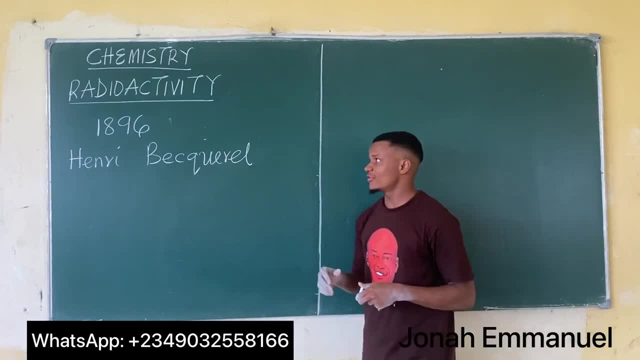 Henri Becquerel, a French physicist, discovered the idea of radioactivity in the year 1896, alright, and it's from this concept that things like atomic bombs are being made. The idea of radioactivity was used to counter John Johnson's theory. you know John Johnson's theory of atoms, which says that atoms can either be created or split, or destroyed. 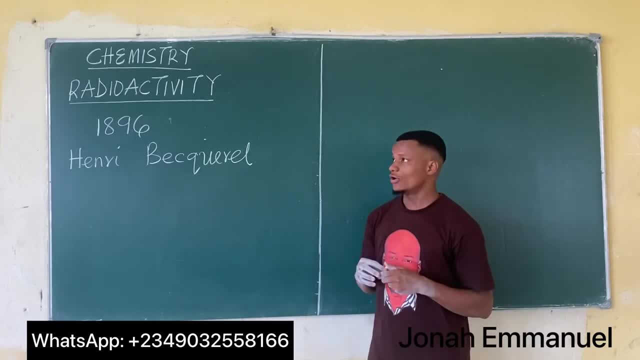 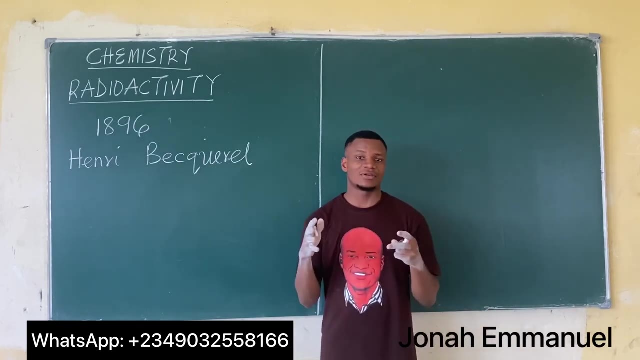 Of course, this concept or this discovery of radioactivity- Henri Becquerel in 1896, actually distorted that theory in the sense that with nuclear fission atoms can be broken down and with nuclear fission atoms can be created. 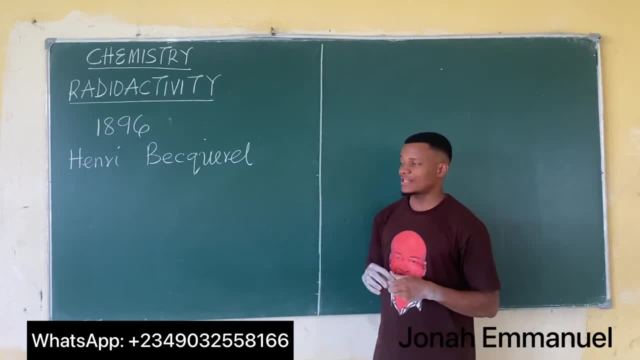 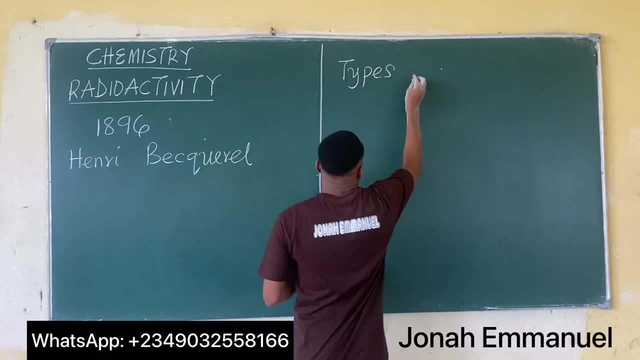 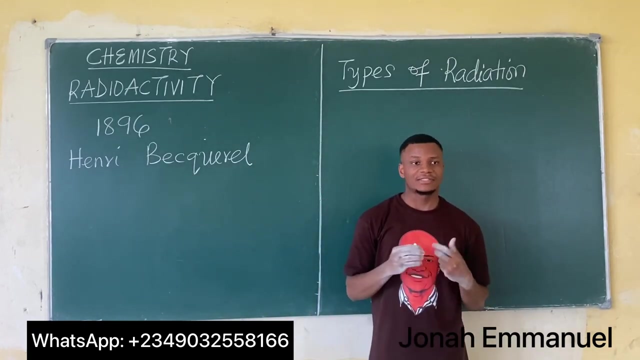 Alright, but we'll look at this much more later. Let's look at the types of radiation. types, Types of Radiation. So from our definition we said when the nucleoside atom undergoes radiation, that three particles, majorly, are being released. 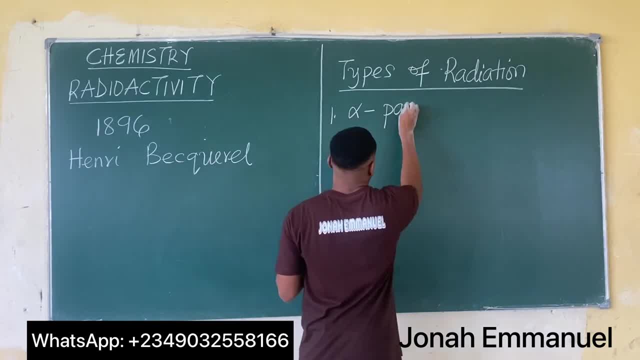 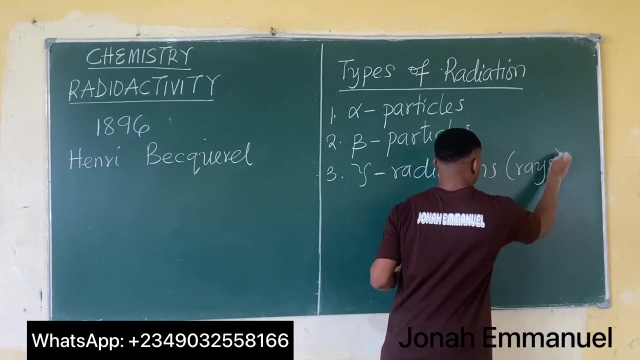 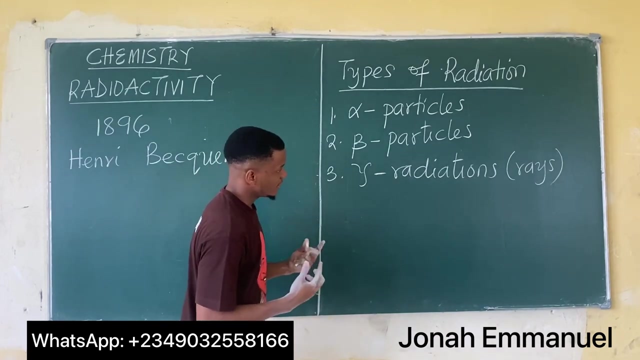 Number one, we said, is alpha particles. Number two, we said are beta particles. Number three, we said are gamma radiation particles. All right, so you have these three as three types of radiation from radioactive elements. By the way, elements that undergo radioactivity are called radioactive elements. 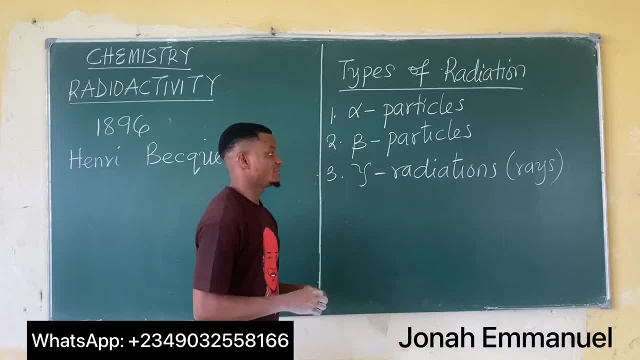 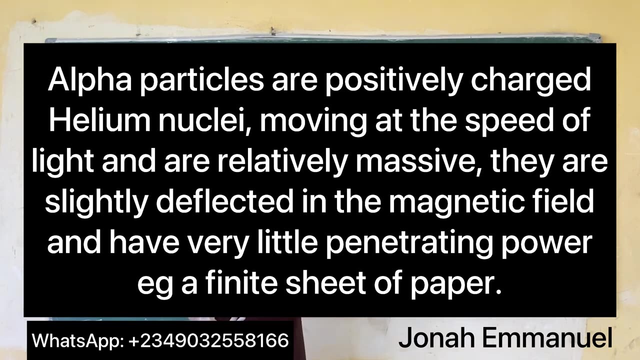 So when they undergo radioactivity, any of these three is being produced. We'll look at the characteristics of each of these three and then we'll proceed. Let's start with the first one there: alpha particles. Alpha particles are positively charged helium nuclei. 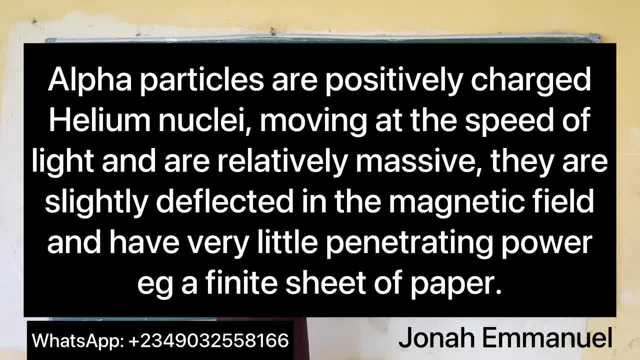 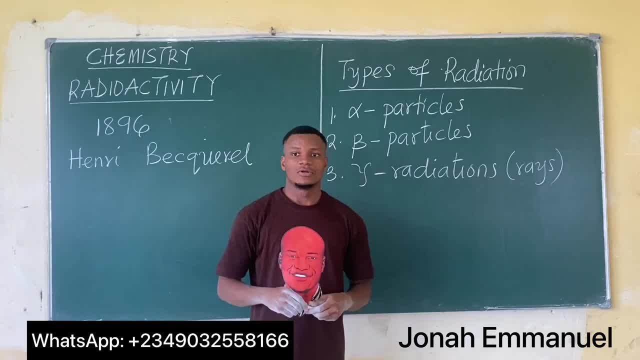 They move at the speed of light and are relatively massive. They are slightly deflected in the magnetic field and have very little penetrating power. Example: a tiny sheet of paper, All right. so that's the characteristic of alpha particles. Let's look at the second one, beta particles. 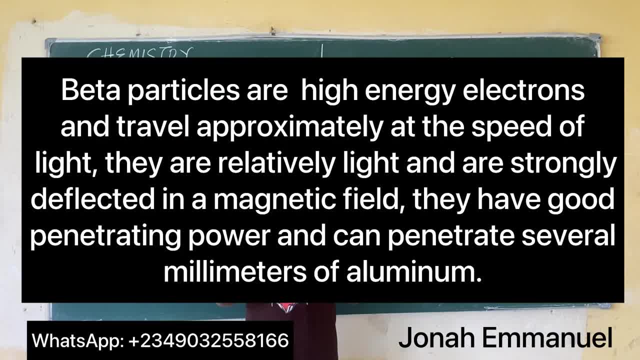 Beta particles are high-energy electrons and also travel approximately at the speed of light. They are relatively light and are strongly deflected in a magnetic field. They have good penetrating power and can penetrate several. So we'll start with gamma rays, gamma rays and we'll talk about the difference between them. 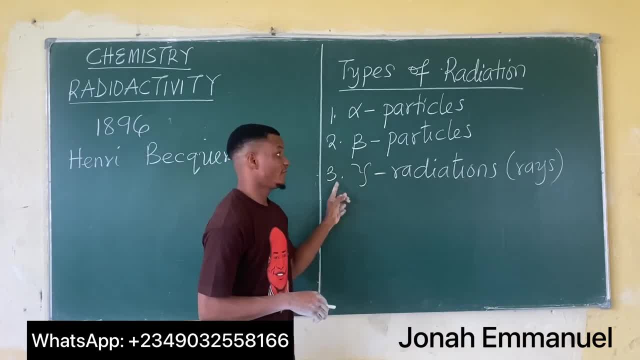 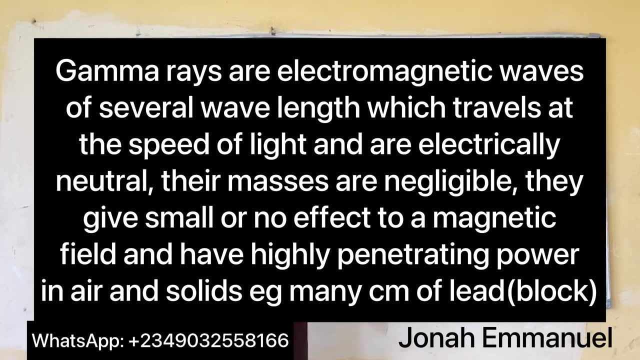 That's like the characteristics of beta particles. Finally, let's discuss gamma rays. For gamma rays, we said gamma rays are electromagnetic waves of very short wavelengths which travels at the speed of light and are electrically neutral. Their masses are negligible, They give small or no effect to a magnetic field and have 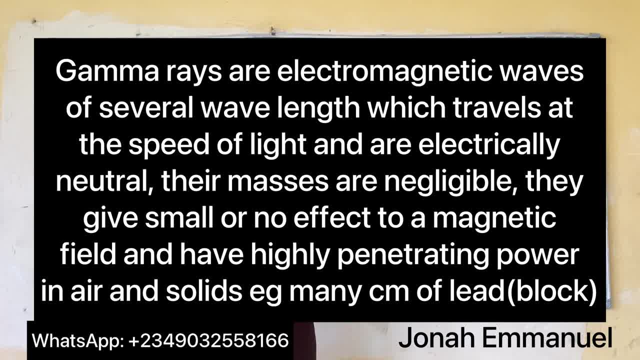 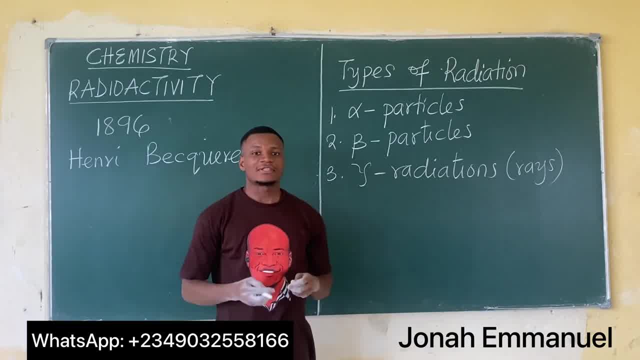 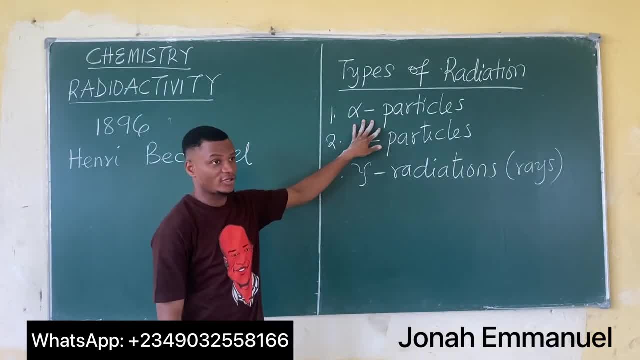 high benefiting power in air and in solids, example, many centimeters of lead or lead block. So, having considered these three the characteristics of each of the types of radiation, we said for alpha particles that they are helium-nucleos, for beta they are electrons. 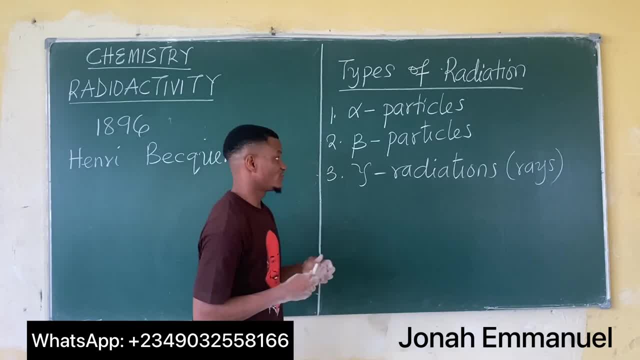 while gamma rays are simply electromagnetic waves. Also, note that alpha and beta are called particles because they are relatively massive, so they have a bit of mass, and so they are most referred to as particles, while gamma rays. the mass of a gamma ray is negligible, so we can see it, doesn't? 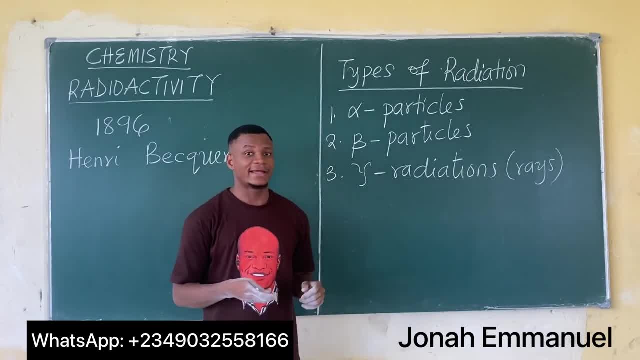 really have a mass, or the mass is too small and hence becomes negligible. and that's why this is not gamma particle, it is gamma radiation, because the mass is almost nothing. We said alpha and beta. of course they also travel at the speed of light, and we said for alpha particle: 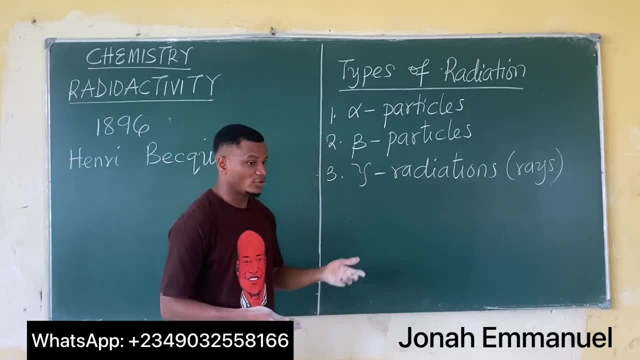 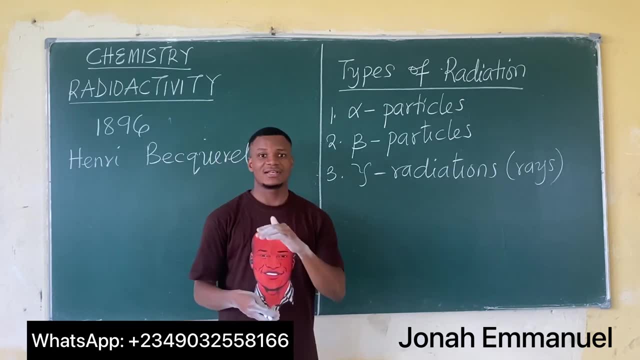 it is slightly deflected in the magnetic field. for beta particles it is largely deflected in a magnetic field. I would say, for gamma radiation it has either no deflection or it has very small or negligible deflection in a magnetic field. So we draw. 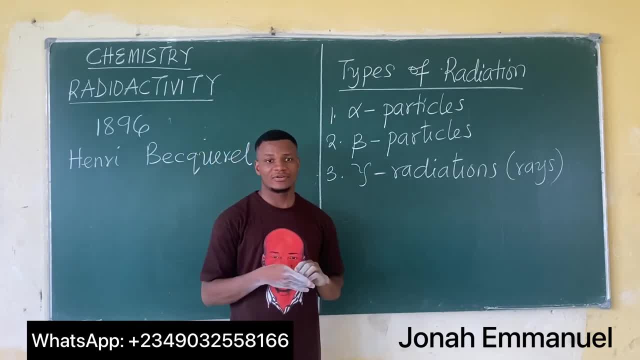 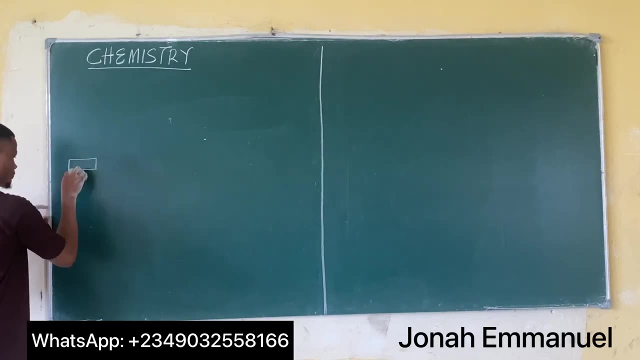 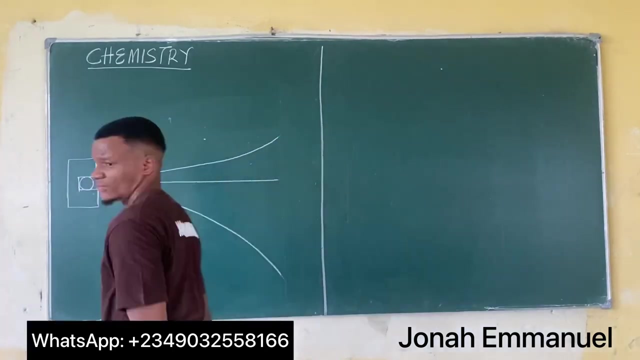 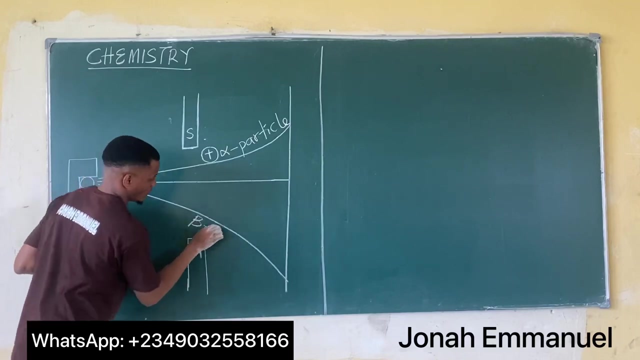 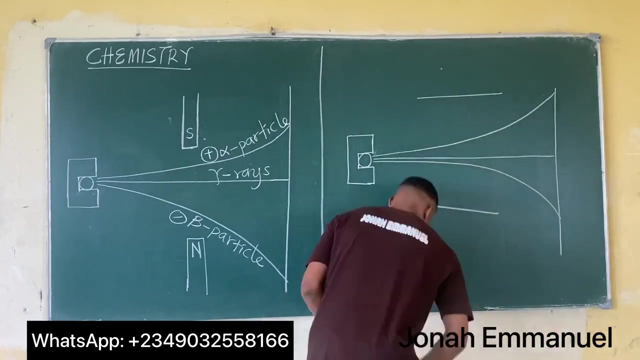 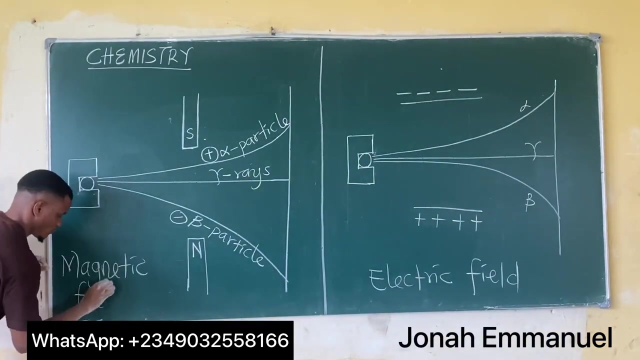 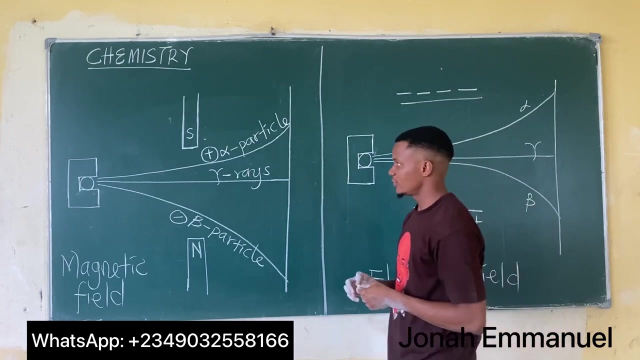 two diagrams, one for magnetic field, one for electric field. and then we look at the deflection of alpha, delta and gamma radiation in both electric field and magnetic field. Alright, so here's a diagram to show the deflection of the three types of radiation in both magnetic field and electric field. 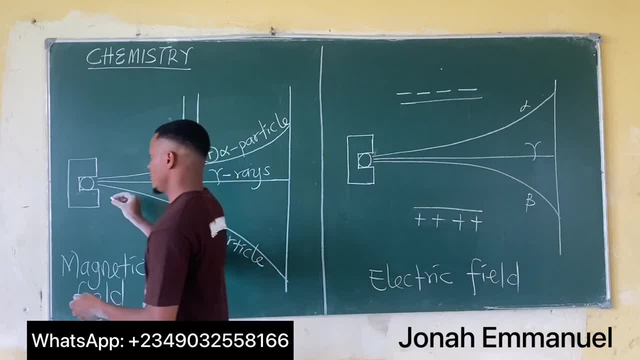 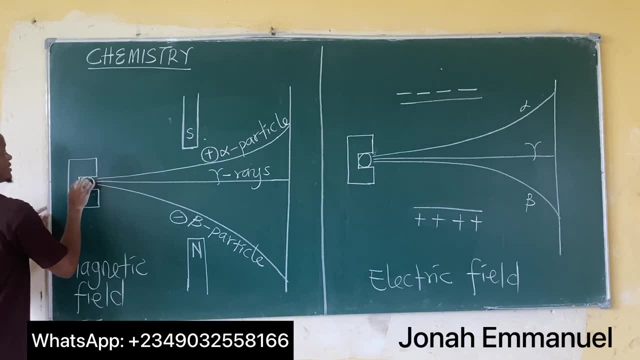 Now let's analyze this. first For magnetic field. now, what you have here is your radiative elements. So what you have here, this one is the magnetic field you have here, this one here is the reductive element. This is the reductive element. What? 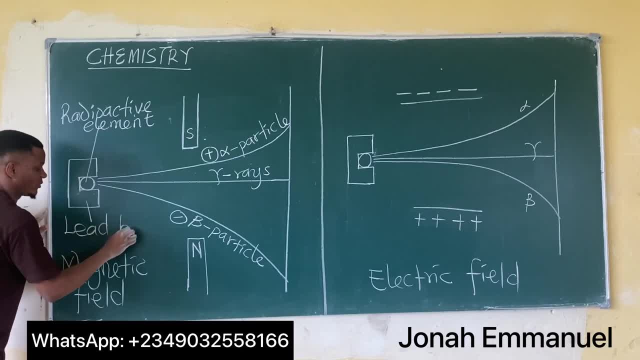 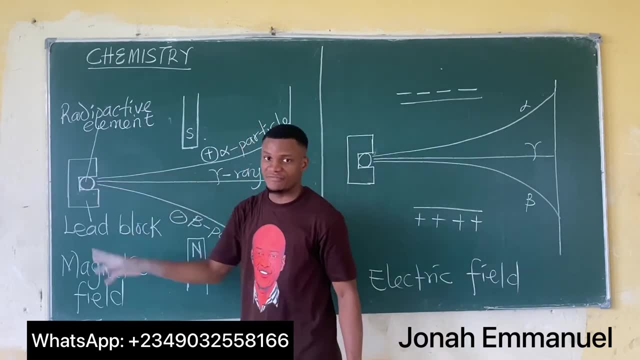 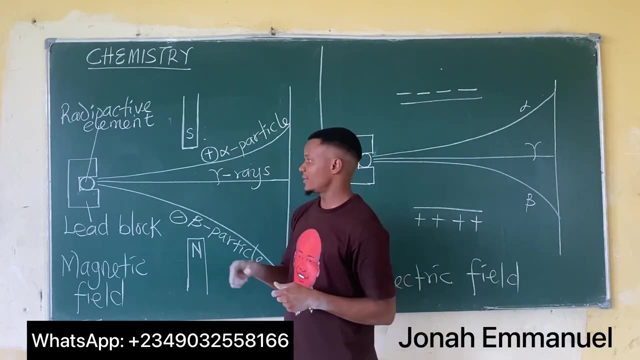 you have here is the lead block. You have the lead block And the lead block is used to ensure that the radiation does not spread to the environment. Of course, we said the kind of radiation that has the greatest effect is the gamma rays, So we use the lead blocks. 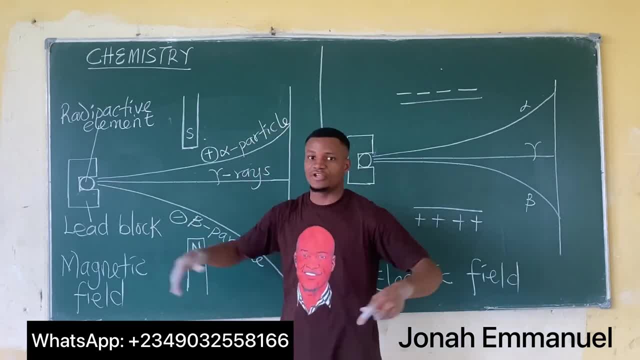 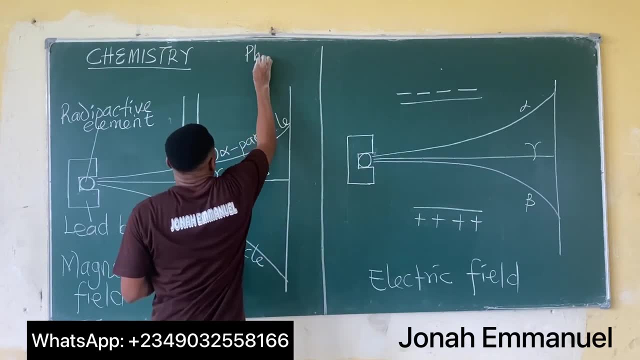 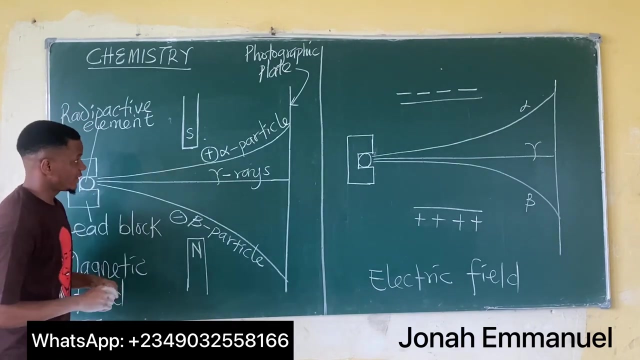 to make sure that the reductive element does not spread that radiation to the environment. All we have here is the photographic plates. This is the photographic plates. All you have here is called the photographic plates, All right, so you have this. For the magnetic field, you observe that the alpha particle 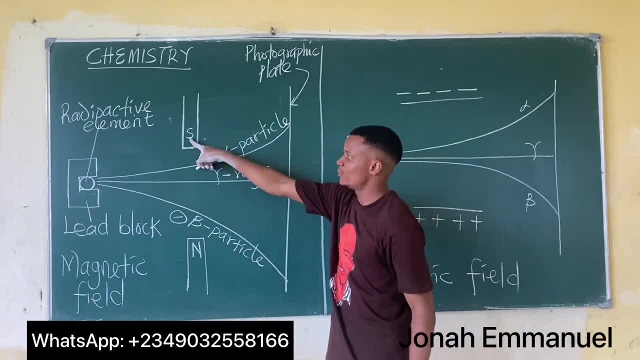 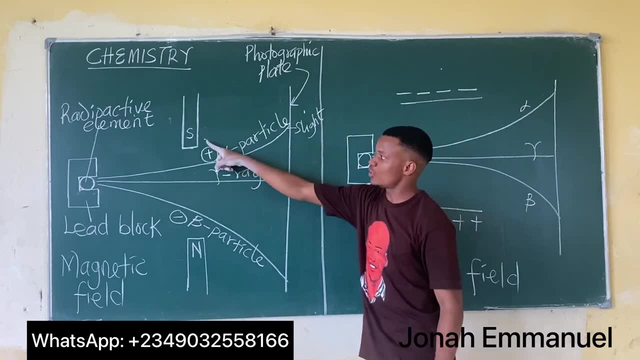 will be deflected, as you can see, towards the south pole, but it will be a slight deflection. So I have slight deflection towards the south pole in the magnetic field, But look at the gamma rays. It is not deflected. So it just goes like this, Or it is slightly like the 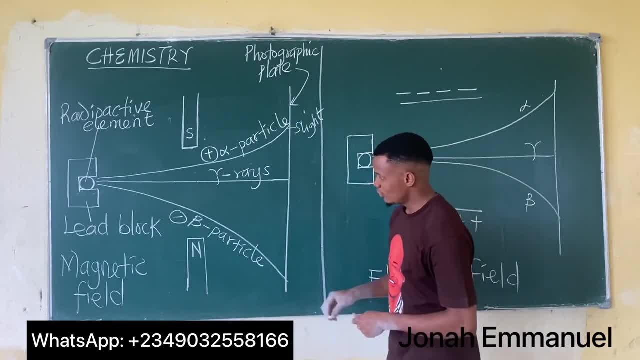 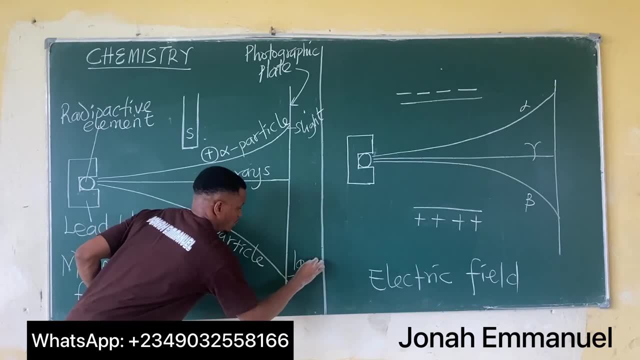 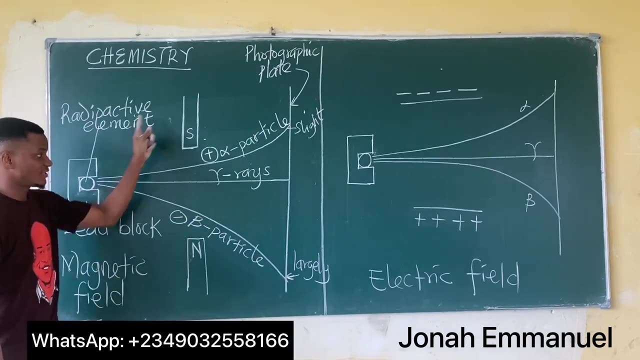 deflection is almost nothing, All right. So this is what is called the alpha particle. It is largely deflected. This is largely. this is largely deflected toward the north pole of the magnet. All right, so this is deflection of the three types of radiation in the magnetic field. 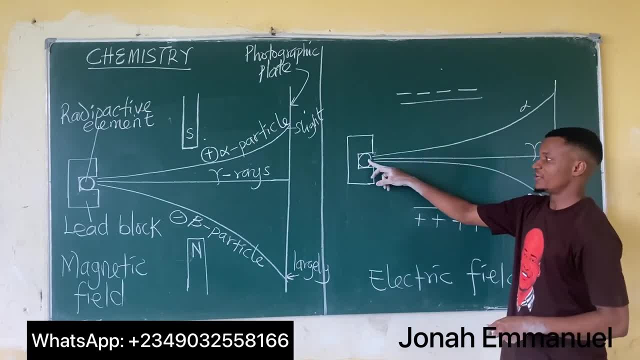 Now if we come about to the electric field, of course this is still the reductive element, this is still the lead block, this is still the photographic plates. Observe that the alpha particles may not be very stable in the Walkman diagramич. 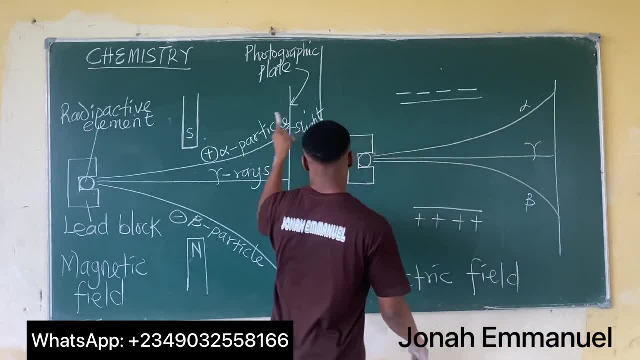 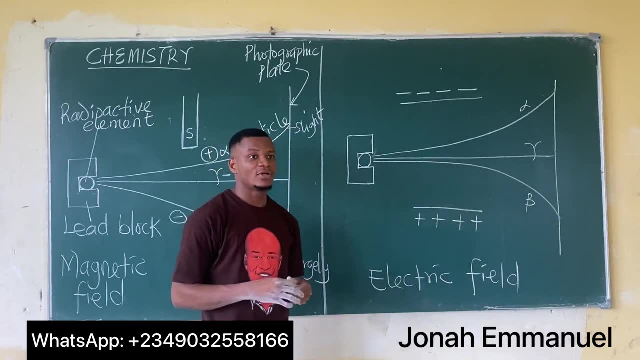 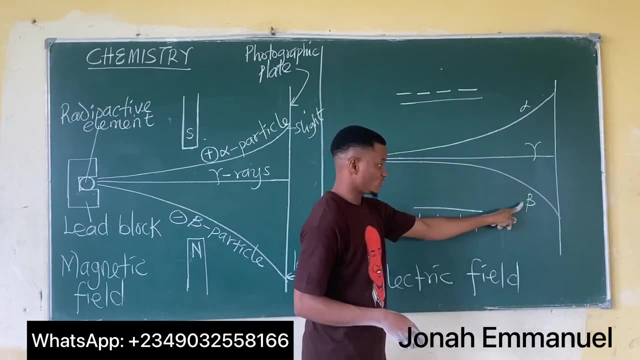 47 itself wall08無 sär. the alpha particle being positively charged will go towards the negative charge, of course, in obedience or in accordance to the first norm of electrostatic, which is light charges attract, all right also. the beta particle will also, which is an electron, being negatively charged will move. 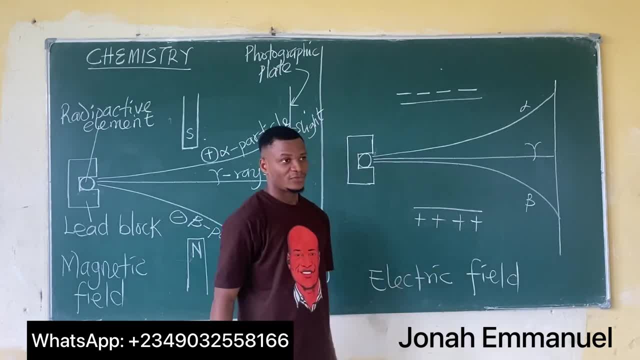 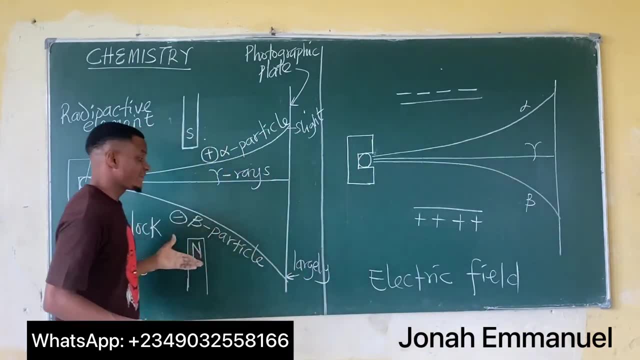 towards the positive region of the electric field. now observe that when it comes to electric field, the deflection are almost alike. all right, but in magnetic field the deflection of the beta particle is large, right, that's it. right. this light is reflected in magnetic field, right, while for 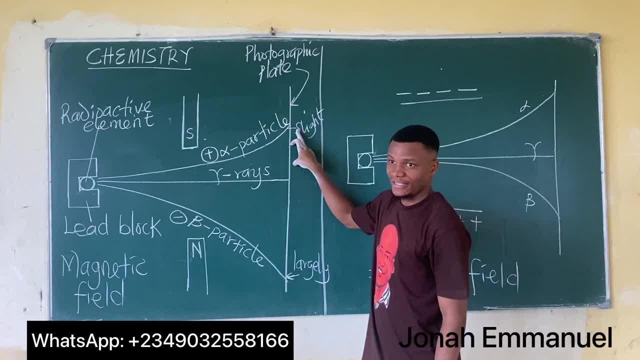 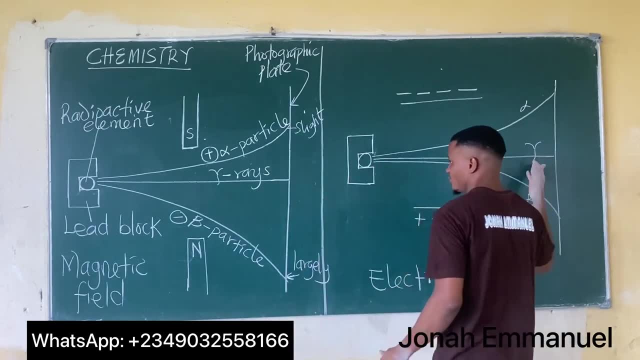 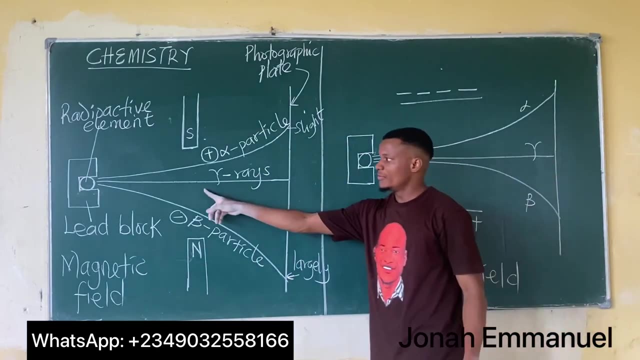 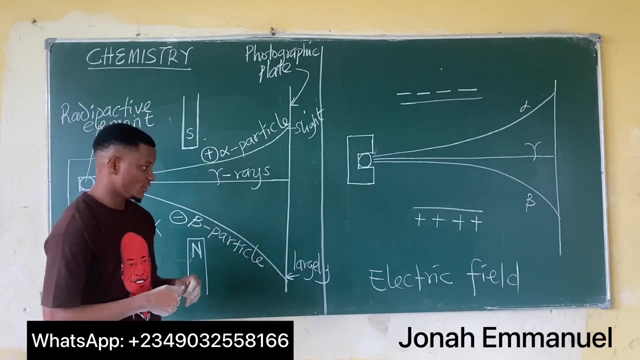 magnetic field alpha particle is slightly deflected, but when it comes to electric field, the deflections are almost like the same thing for gamma rays. whether it's in magnetic field or it is in electric field, observe that there is no meaningful deflection. so this is deflection of radiation in both electric field and magnetic. 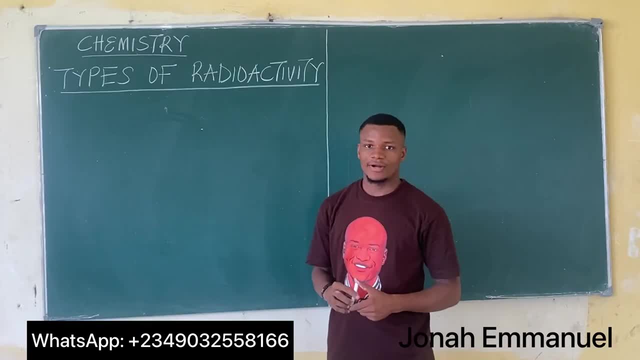 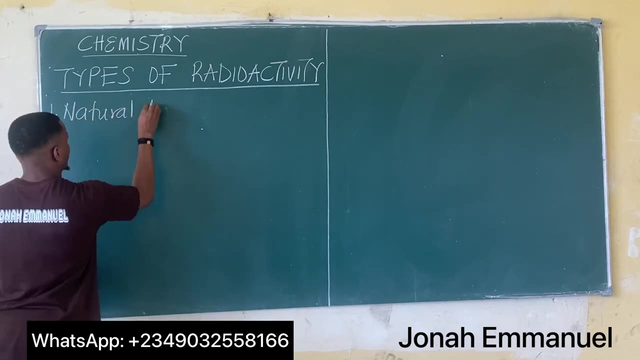 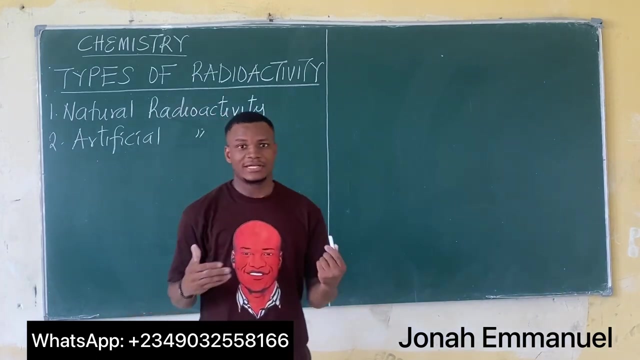 field. all right, let's proceed. all right, so let's look at the types of radioactivity now. generally, there are two types of radioactivity. number one, natural radioactivity. number two, artificial radioactivity. so these are the two types of radioactivity by definition: natural radioactivity. 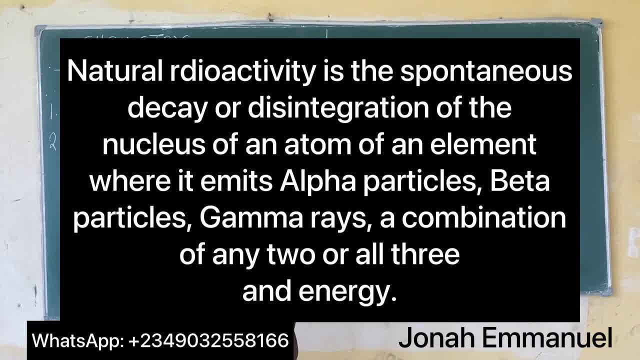 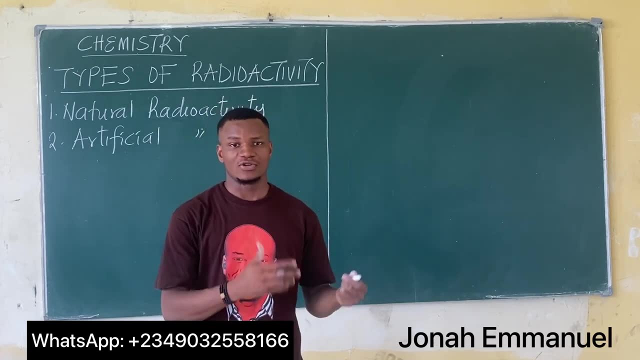 is simply the spontaneous disintegration or decay of the nucleus of an atom, where alpha particle, beta particle, gamma rays, a combination of any two or all three, is being released with the release of heat energy. now, the heat energy released during radiation is called nuclear energy. now, when it comes to 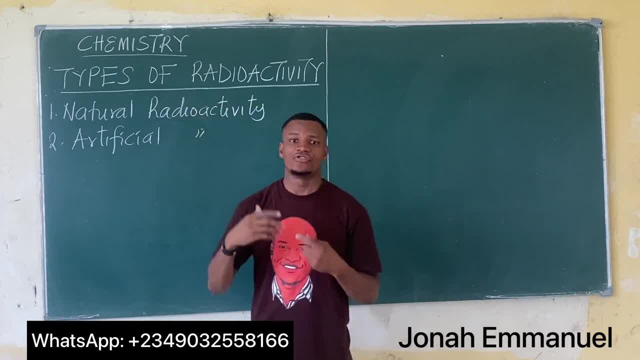 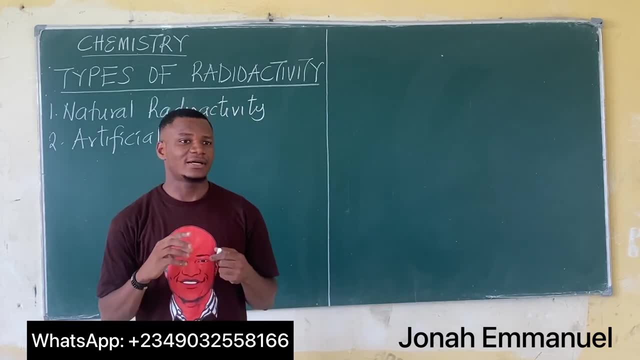 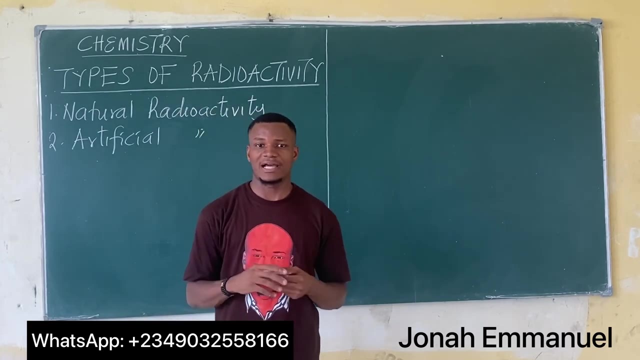 a definition for both natural relativity and reactivity. in general we said it is the spontaneous decay of disintegration. now let's analyze the third decay. we'll talk about the second decay. in radioactivity there are usually two types of decay. the first one is called alpha. 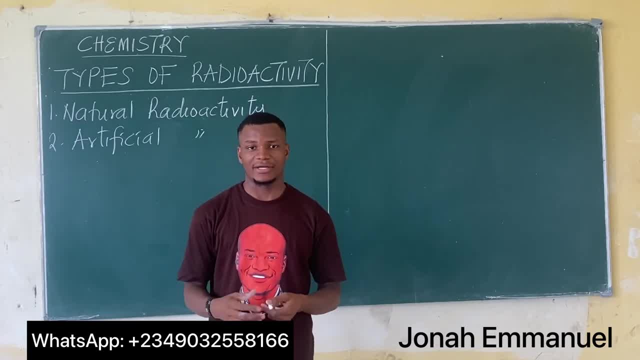 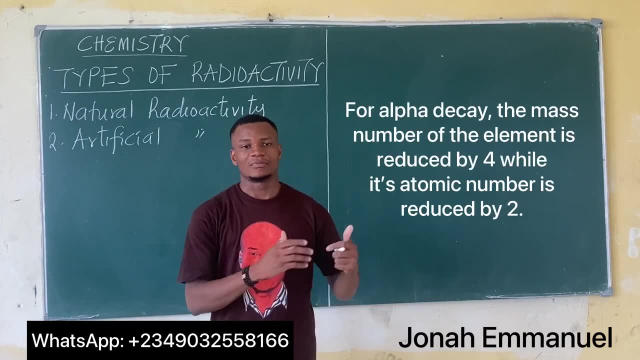 decay, and the second one is called a better decay. all right, during alpha decay you have a particular element, decay of being that a particular element is being broken down to form a new element, in which the mass number of the new element is being reduced by four and the atomic number of the new element is being reduced by two. basically, while for a better decay, 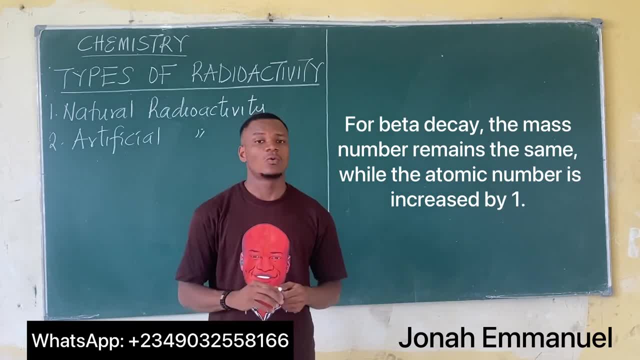 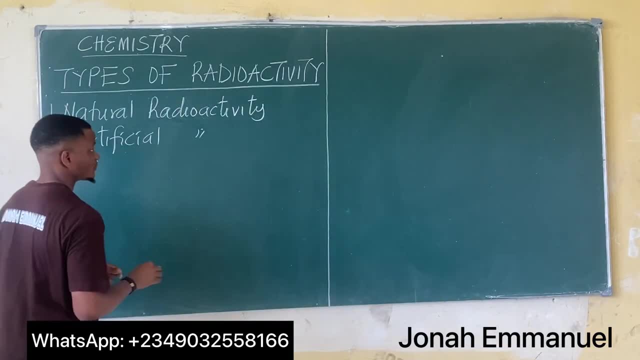 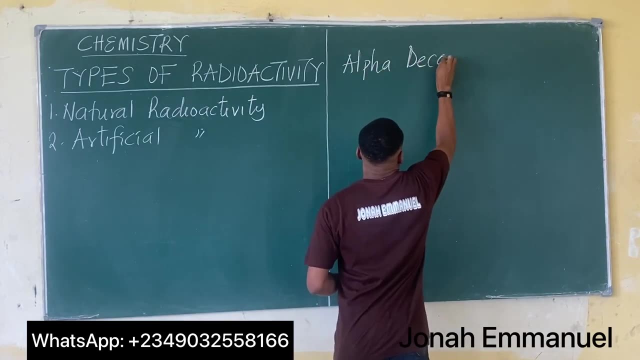 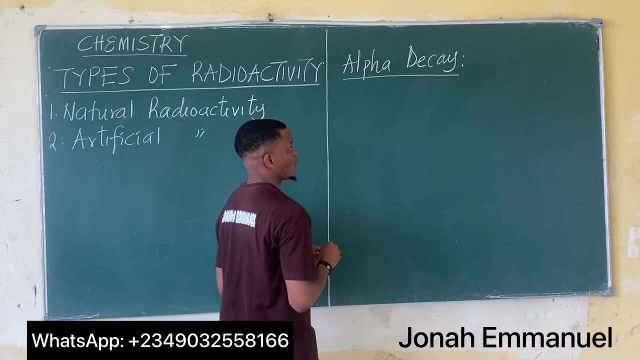 the mass number of the new element remains the same, while the atomic number of a new element is being increased by one. so this is the chemical equation for an alpha decay. generally when it comes to decay, decay for alpha decay. the general equation for an alpha decay is given by: let's have an element x having atomic number z. 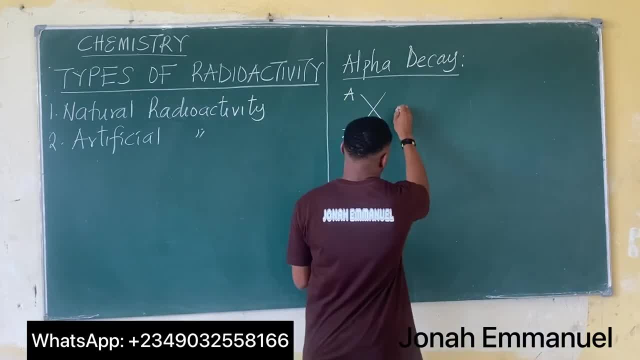 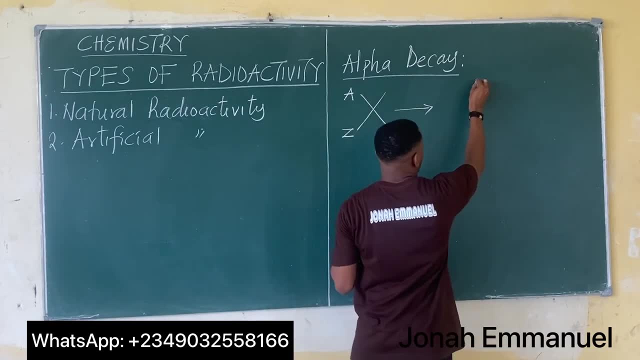 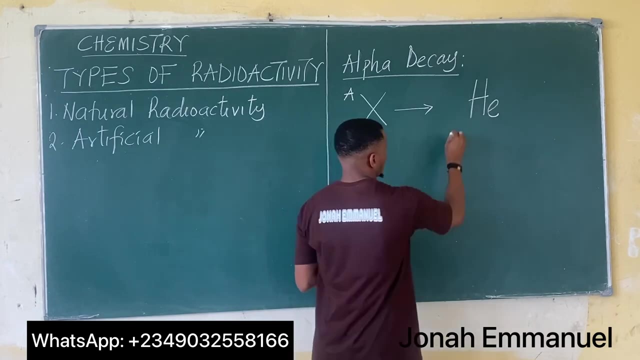 and mass number a. i have this. if this element under owes alpha decay, of course, since it's an alpha decay, that means an alpha particle will be produced, and when we discuss alpha particles we say they are helium and new light. this is uh two here. so this is the new might symbol for the. 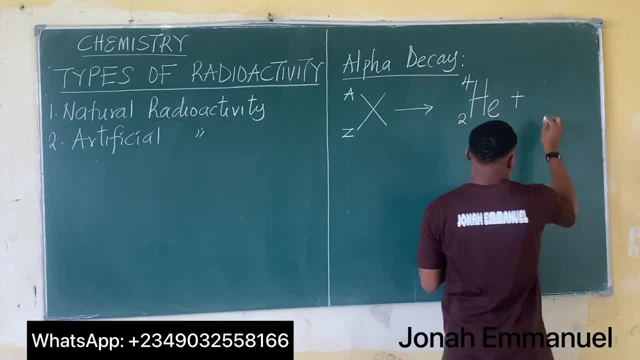 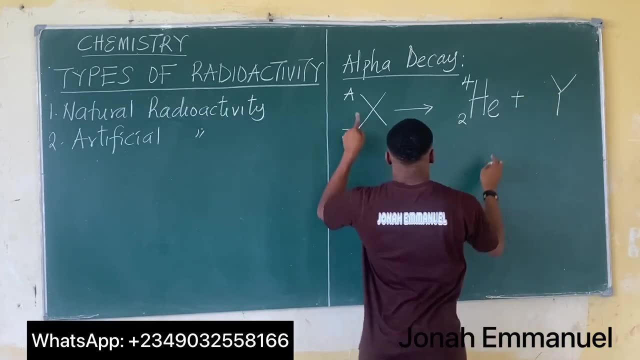 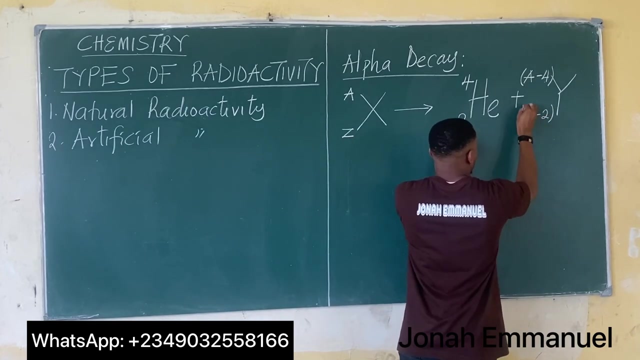 helium plus, you have a new element in form. let's call the new element y for y. here we say, the new mass number becomes what i have here, a minus what i have here 4. so you have this y for the atomic number i have here, c, to become c minus what i have here two. all right, so this. 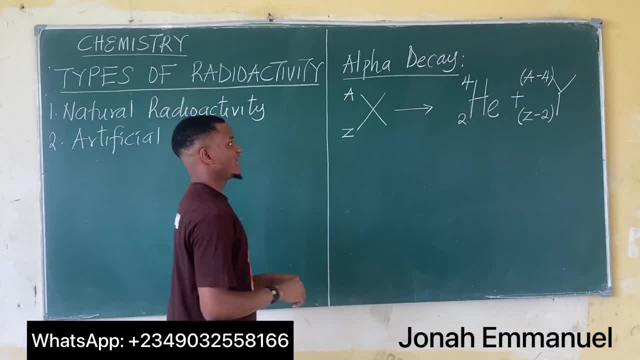 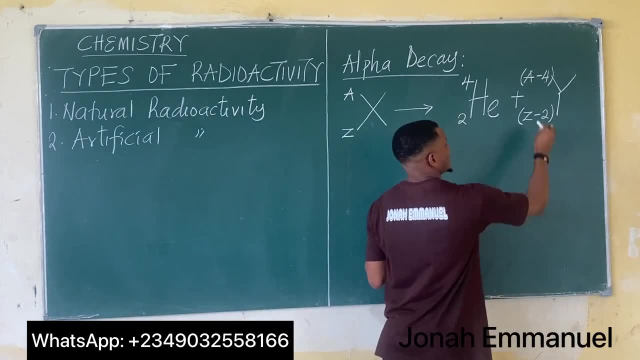 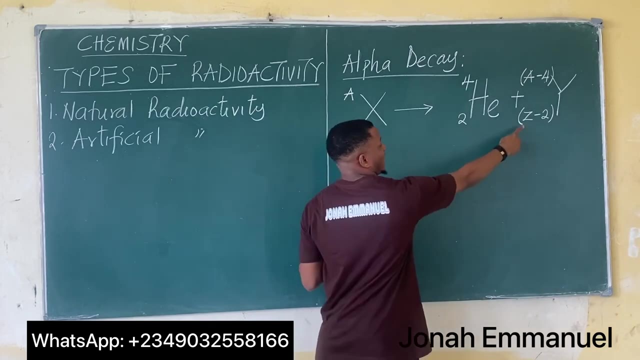 is like the general equation for an alpha decay. and for an alpha decay we said an element would disintegrate to form a new element, such that the mass number of the new element would differ from this one by four, and also the atomic number of the new element would. 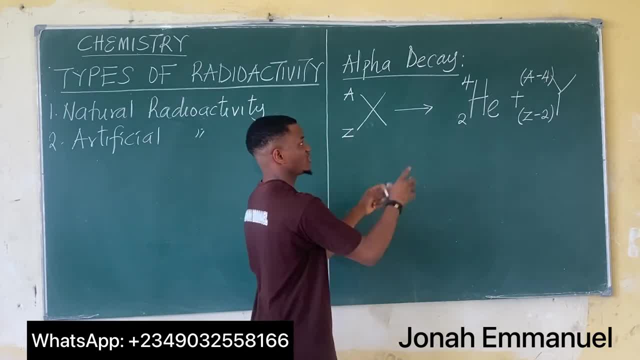 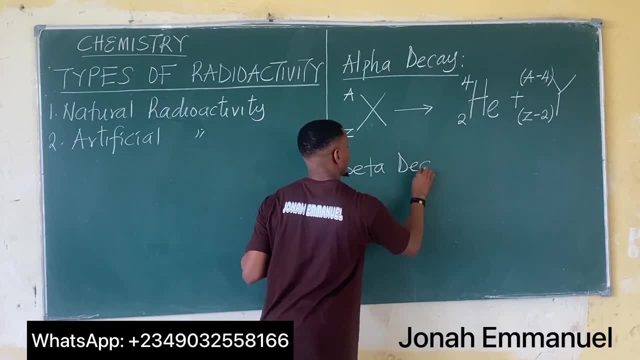 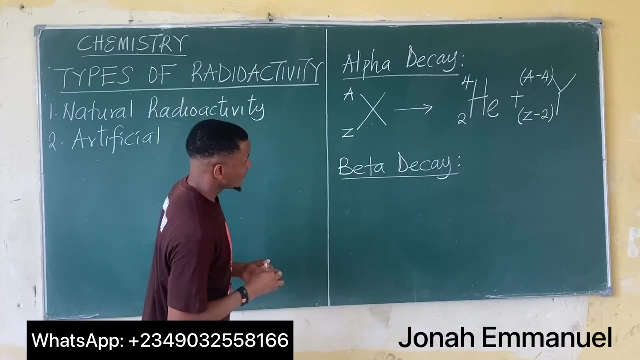 differ from, uh, this one here by two. all right, this is joined to general one. if you look at better decay, second one is better decay for better decay. the general equation would be this: so i have an element x having atomic number z and mass number a. this is undergoing better decay of. 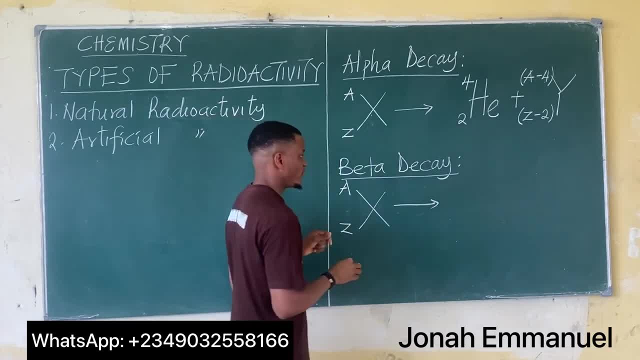 course we said for better. we said they are electrons. for electrons we have that every number is minus, is one and the mass number is zero. all right, for this it becomes plus. a new element is formed, y, such that now, when it comes to getting a new atomic number from a new element, we said it was- 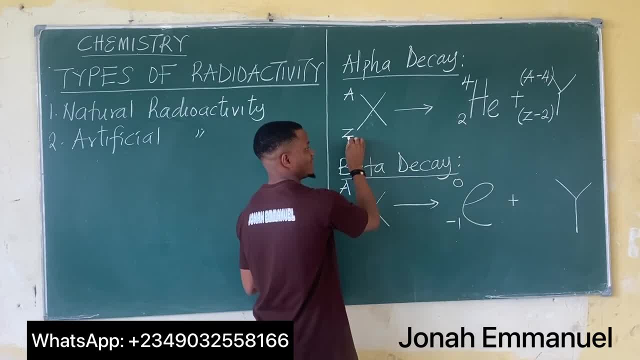 this one here minus this, so it becomes z minus two. with that same concept for this becomes z. this one here minus what i have here minus one becomes z minus what hybrids, it becomes Z minus 1.. And that's equal to Z minus minus Jc plus 1.. 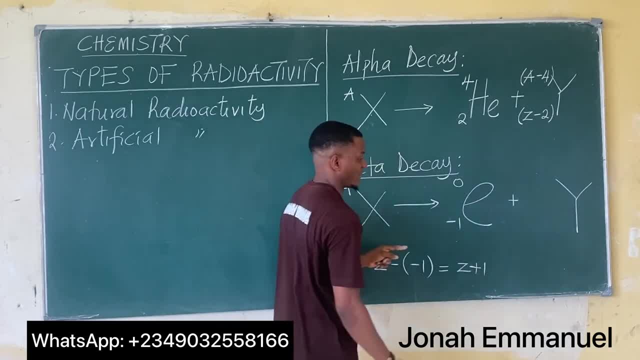 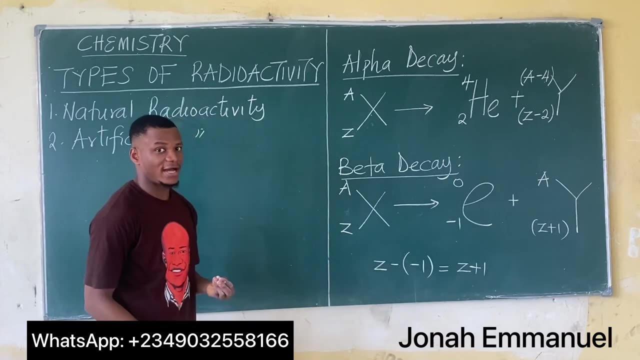 Having Z plus 1 as the new atomic number. So it becomes Z plus 1.. Yeah, Same thing here. This one becomes A minus 0, which is obviously A Alright. So this becomes the major difference between an alpha decay and 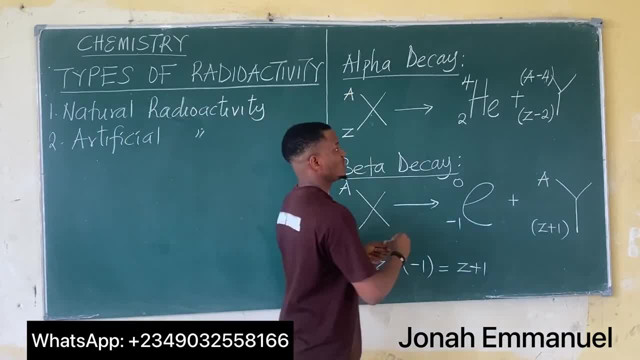 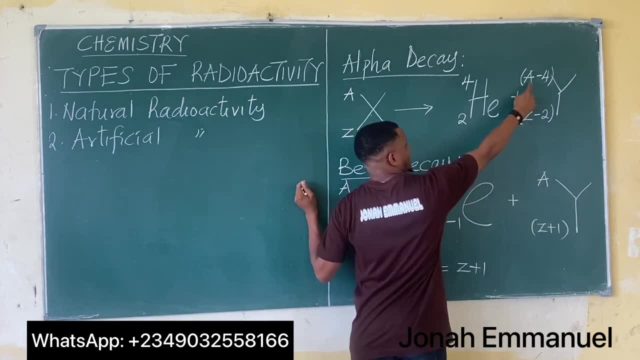 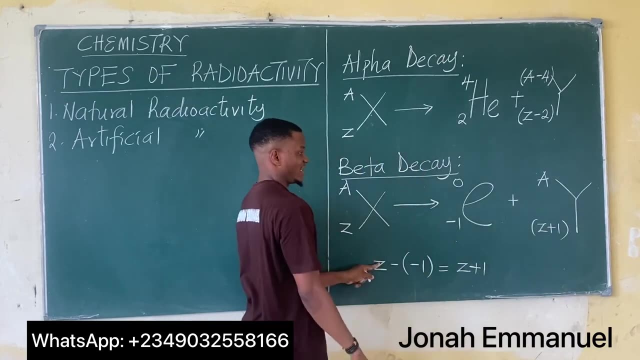 a beta decay. For an alpha decay, the new element formed is such that its atomic number is being reduced by 2, and its mass number is being reduced by 4.. While for beta decay, a new element is being formed such that the atomic number 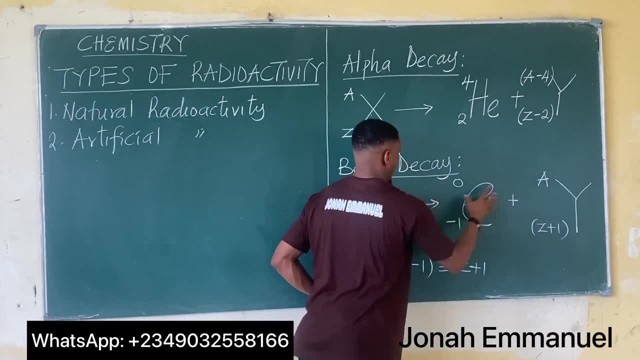 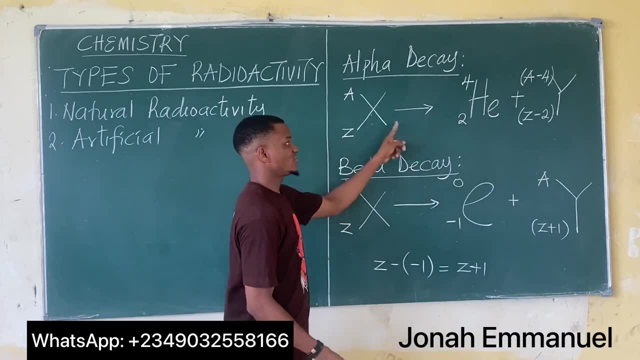 is being increased by 1, while the mass number remains the same. This is, in its basic state, okay, That if it emits just one beta particle and it emits just one alpha particle, I will have the same result. So this is like: 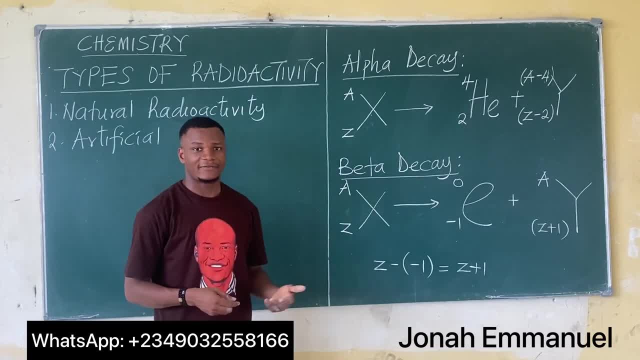 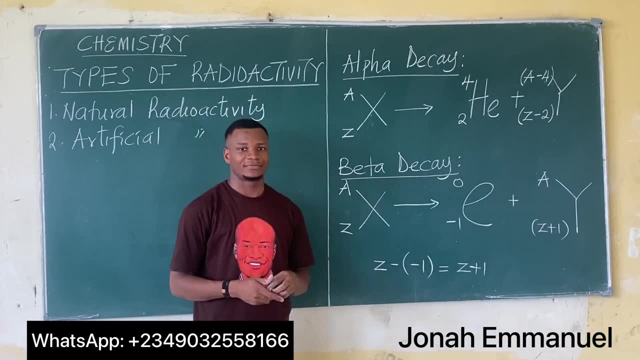 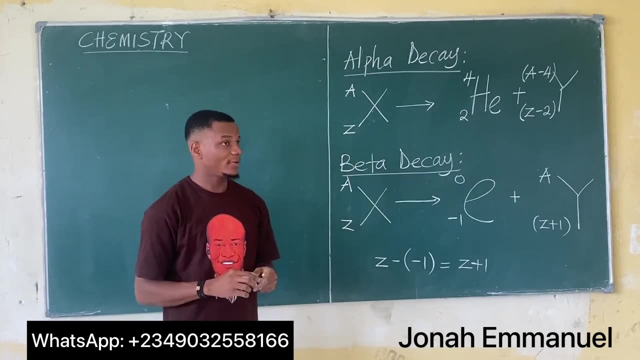 the simple idea behind alpha and beta decay. We'll take some examples to explain the concept of alpha and beta decay. Alright, so an example of an alpha decay is when radium-226 decays to form radium-222, as given by the patient below. 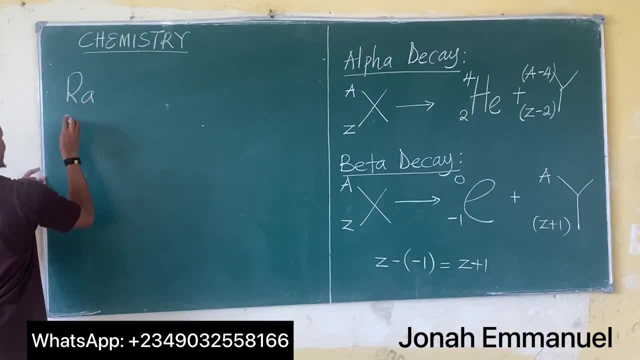 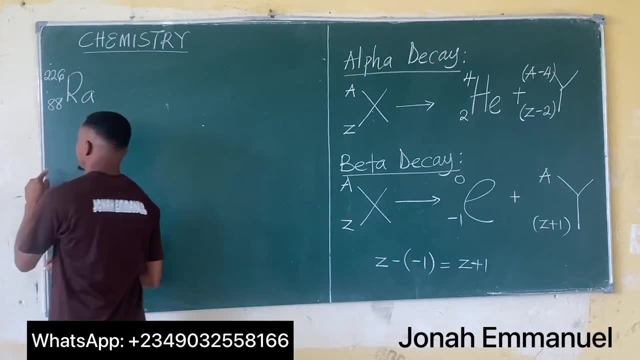 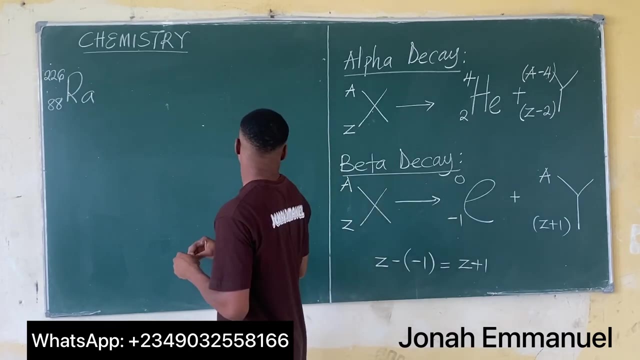 So I'm having radium RA having an atomic number of 88, and mass number of 226. So this element is called radium. It's the radioactive element. If this element undergoes alpha decay, it will produce helium nucleus, of course. 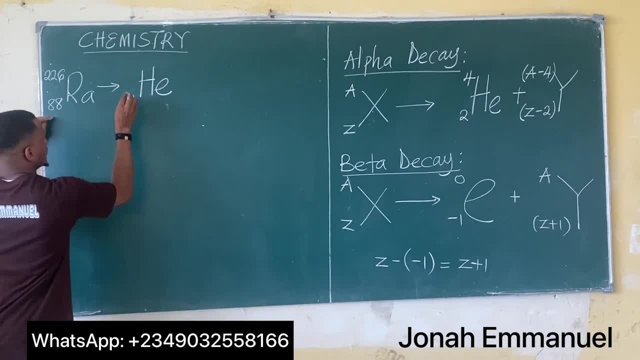 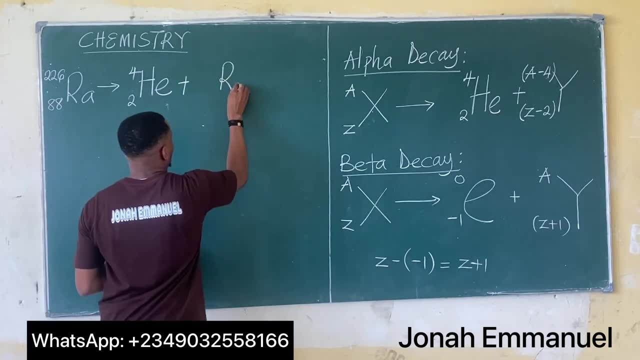 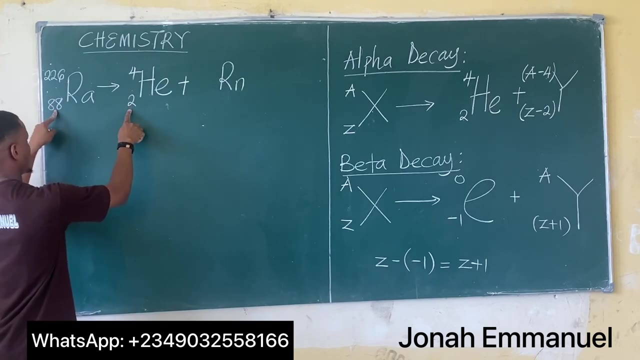 HD, such that here it becomes 2 and 4, plus the new element form which is called radon. So I have this here. For radon they have decided, the mass number becomes this: one minus this, So it becomes 88 minus 2.. 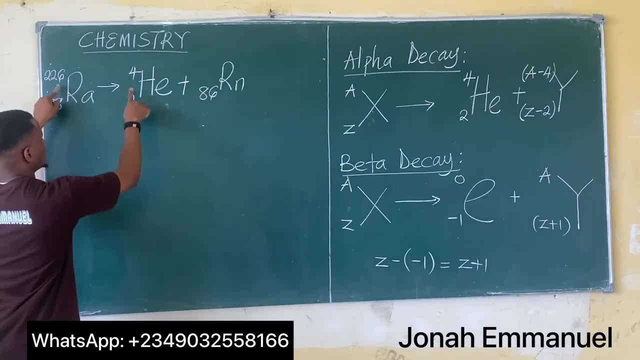 That gives you 86.. While for this one it becomes 226 minus 4.. That gives you 222.. Alright, So I have a cell that's called radium, while I have a cell that's called radium, While I have a cell that's called radium. 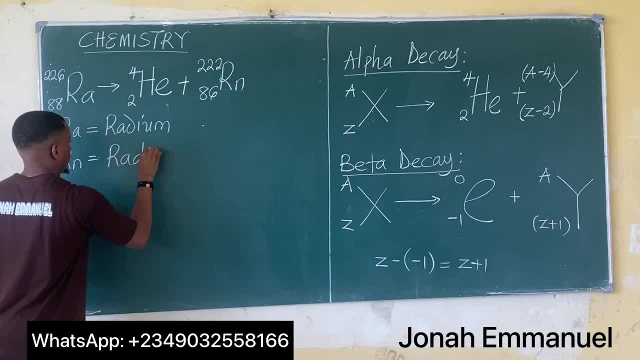 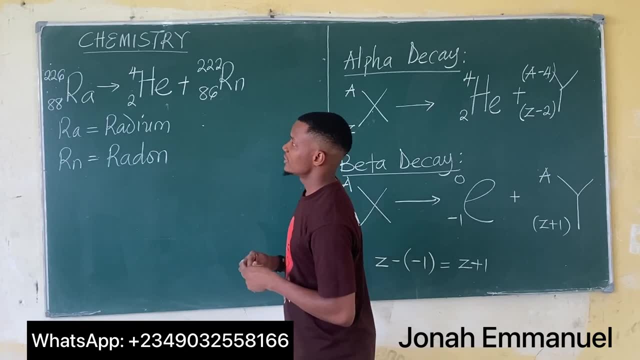 While I have a cell that's called radon. Alright, So these are like two elements under the activity. Now, of course, we said it is continuous disintegration or decay, such that for this one, since it's an alpha decay, alpha particle is being released. 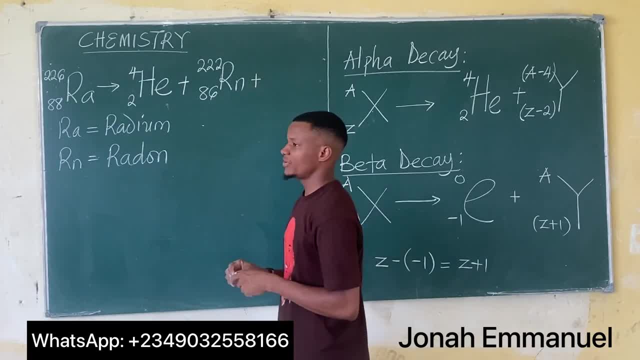 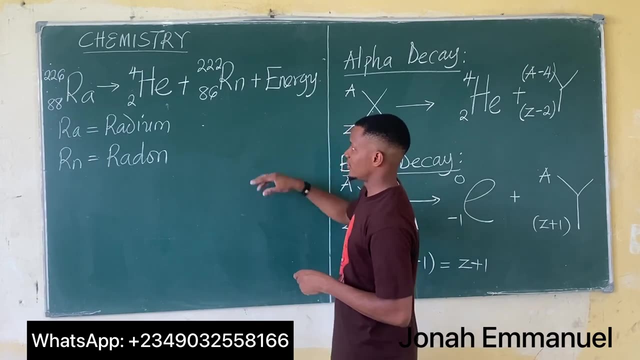 And we said: at the end you have an energy being released. Of course we said it's heat energy. It becomes plus energy. Alright, So whenever it comes to writing radioactive decays, at the very end there should be energy there. 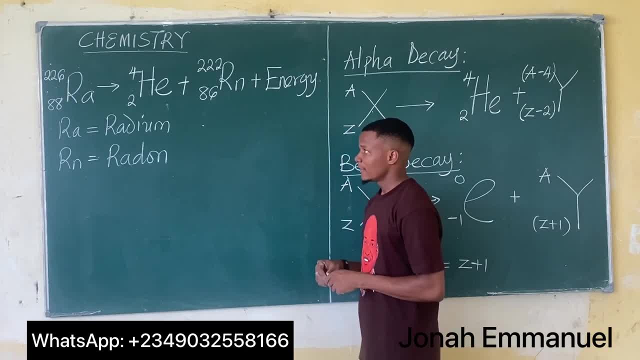 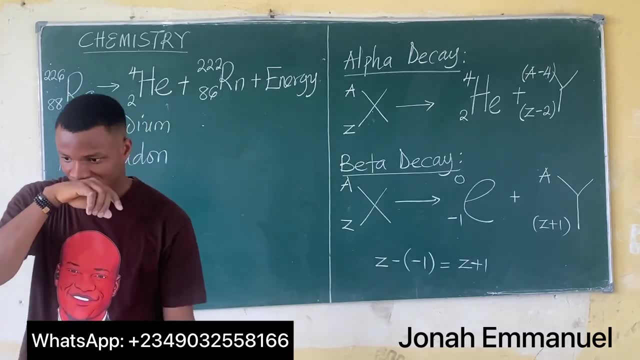 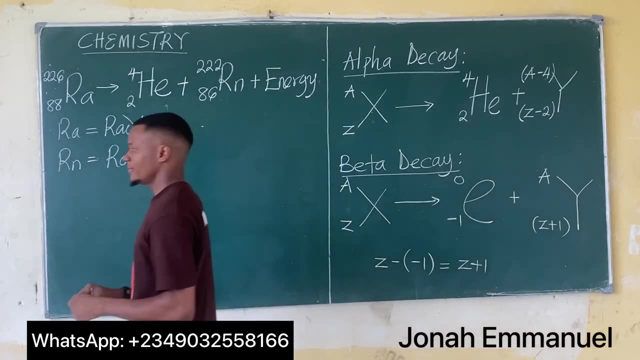 So I have this. So this is an example of an alpha decay. Let's take an example to explain beta decay Also, let's get for beta decay. Let's take an example of beta decay Now. one example of beta decay is that. 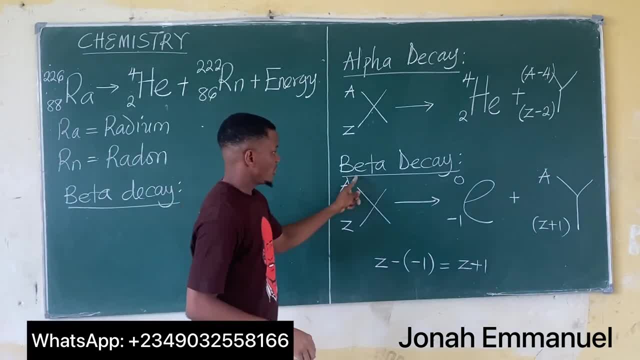 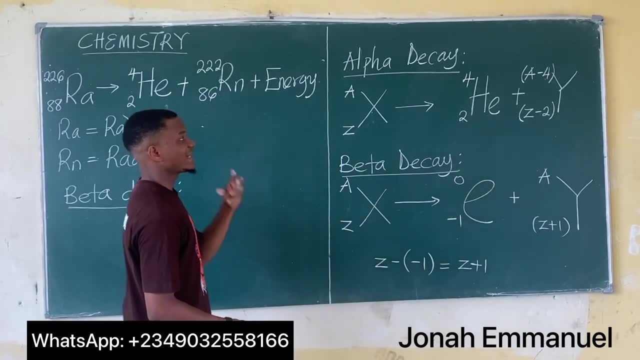 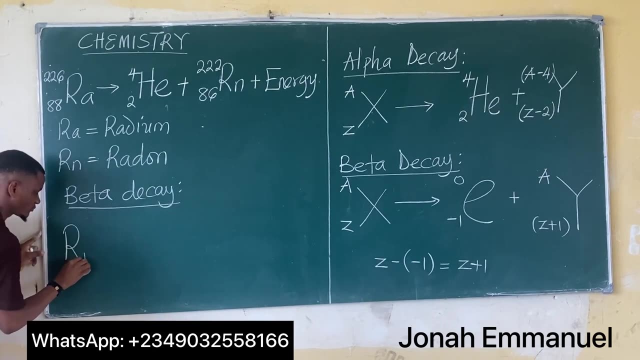 radon emits two or undergoes beta decay to emit two particles, or two beta particles to produce an isotope of radium. Alright, So I have radon, that's Rn, atomic number 86, as we see here, and mass number 222.. This is because 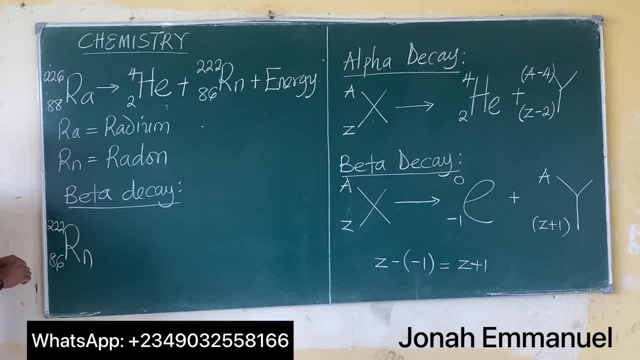 it becomes 222.. Okay, It would emit two of beta particles, that's electron minus one and zero to produce. now the new element becomes 86.. So we say 86 minus two times this. that becomes two times minus one, that becomes equal to 86. 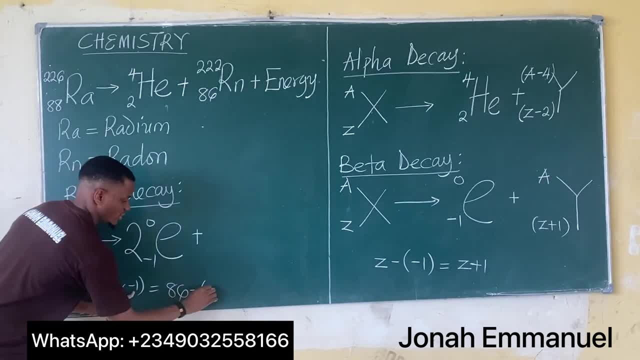 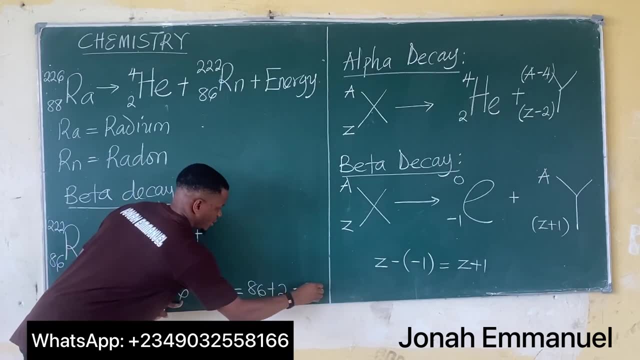 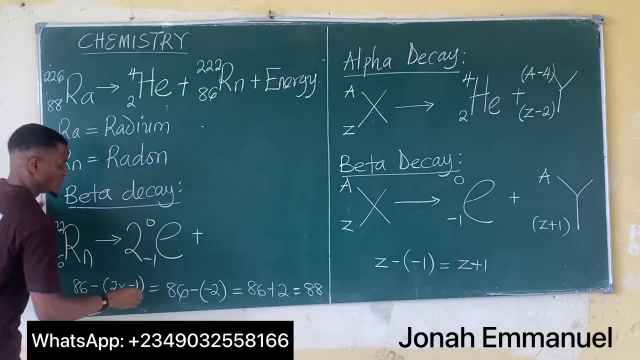 minus two times minus one is minus two, and that's equal to 86 plus two and that's equal to 88.. So the element that has atomic number 88, of course, as you can see here, is radium. That means I'm having Rp. 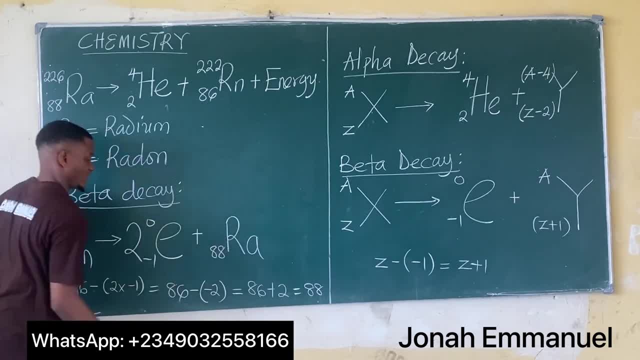 here radium having atomic number 88. So I have this For the mass number. it becomes this one here. That becomes that becomes 222 um 222 minus. of course. this was two times minus one. This now becomes two times zero, That's. 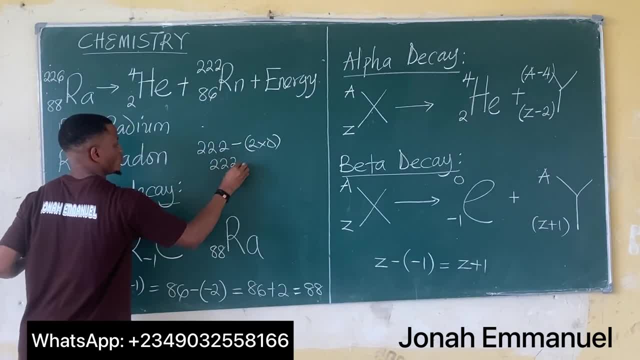 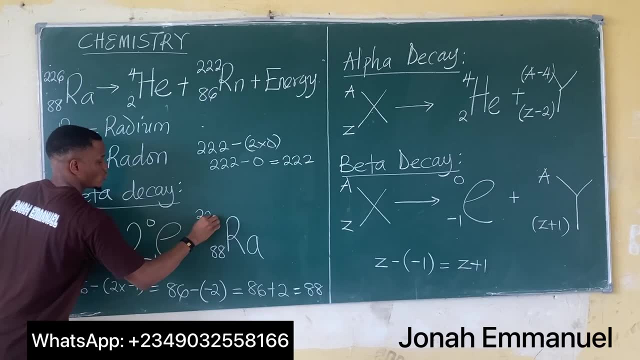 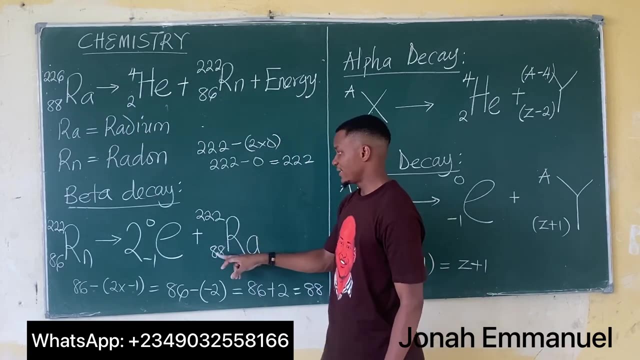 two times zero, I'm having 222 minus two times zero is zero. That gives you 222.. So the mass number here becomes 222.. So observe this and this: they are both radium, having the same atomic number- 88 and 88, but different. 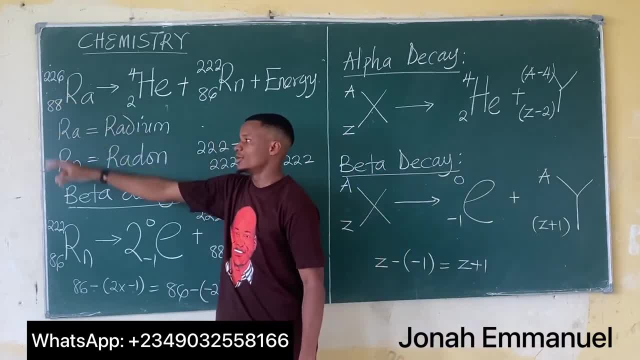 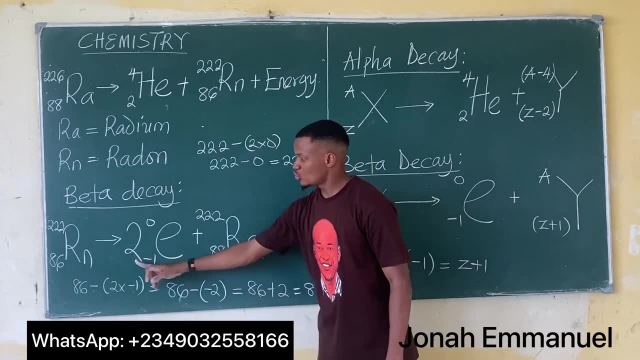 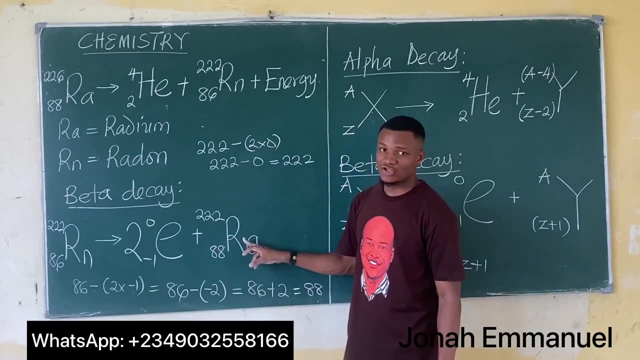 mass number 222 and 226. So we can say: um radon undergoes beta decay to emit two particles of, or to emit two beta particles to produce an isotope of what Radium. So we can say this one here is an isotope. 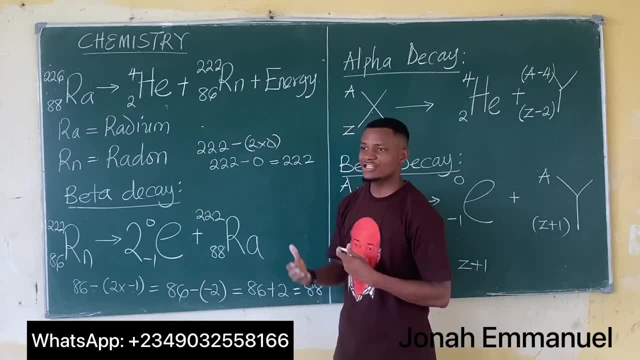 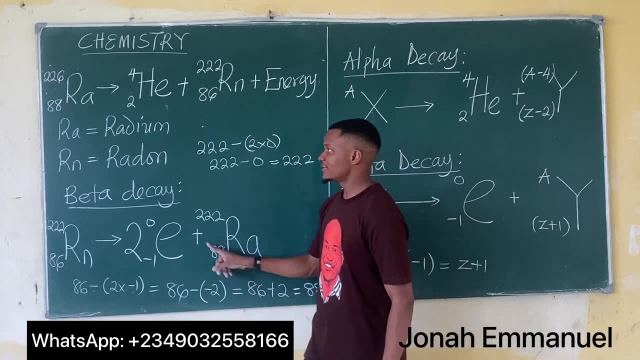 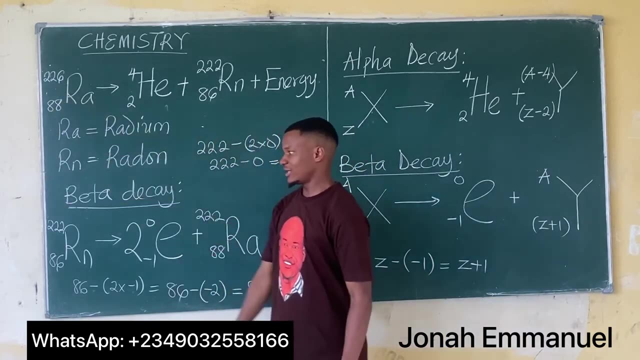 of radium. Now, don't forget that in the concept of isotopy we said an element has, or isotopes refers to elements that have the same atomic number, 88, but different mass number: 222 and 226.. So they are different mass number. So we can. 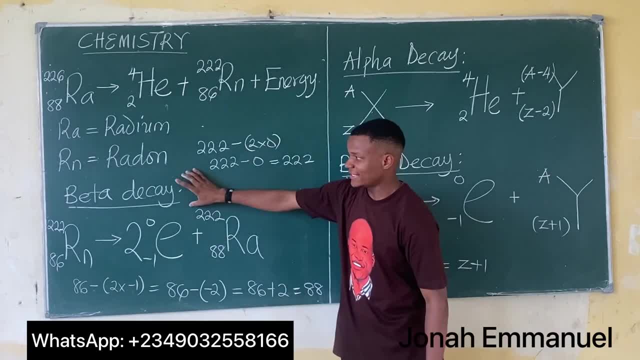 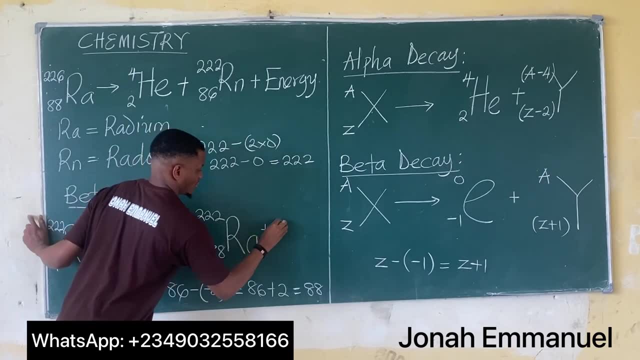 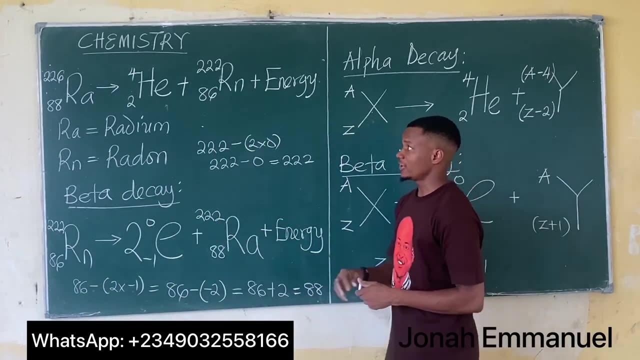 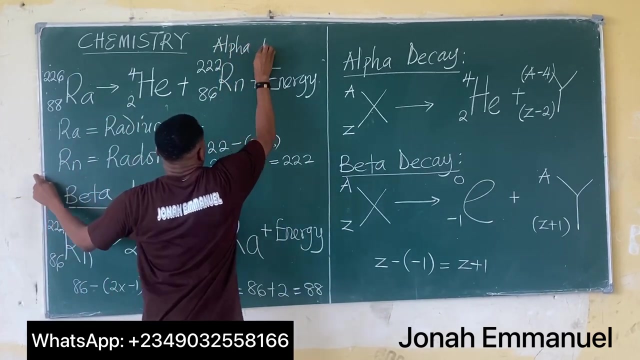 say, radon undergoes beta decay to produce an isotope of radium, Of course, plus very important energy, plus energy, Alright. so this is how the concept of alpha decay, which is this? perhaps I should explain this here. this is how alpha decay and beta decay works. 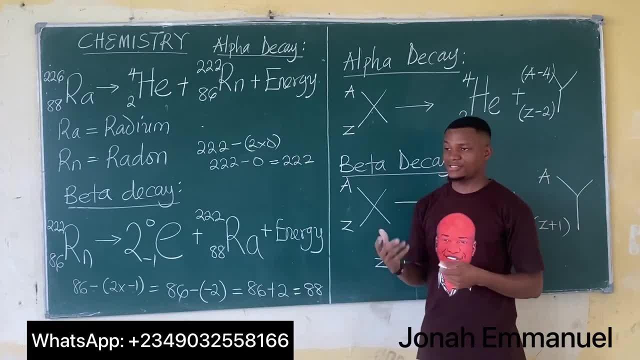 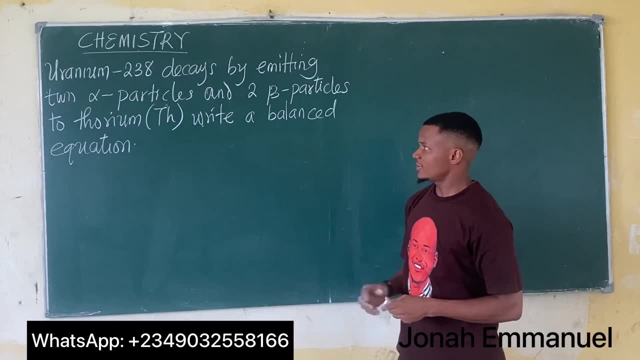 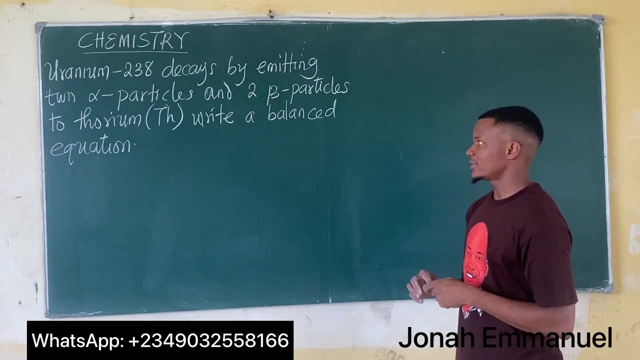 We will take more examples on alpha and beta decay and explain this point much better. Alright, so let's take a simple example to first understand the concept of alpha beta decay. So this question says Uranium 238 decays by emitting two alpha particles and two beta particles. 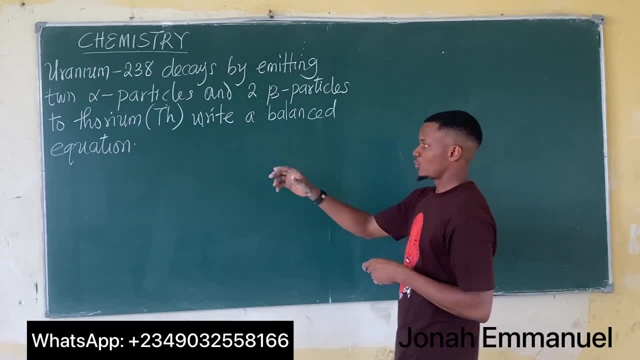 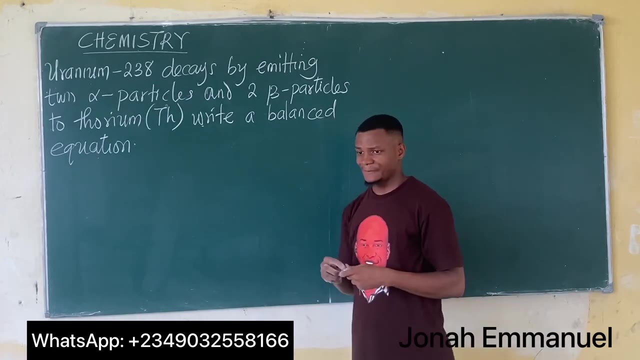 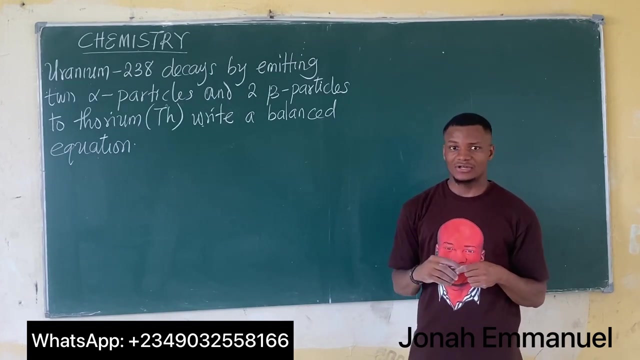 to thorium. So thorium is actually an element whose symbol is TH. It says: write a balanced equation. So we will try to write a balanced equation for this particular decay Now, before then for me to notice. this Decay, or this integration, is actually a decomposition reaction. 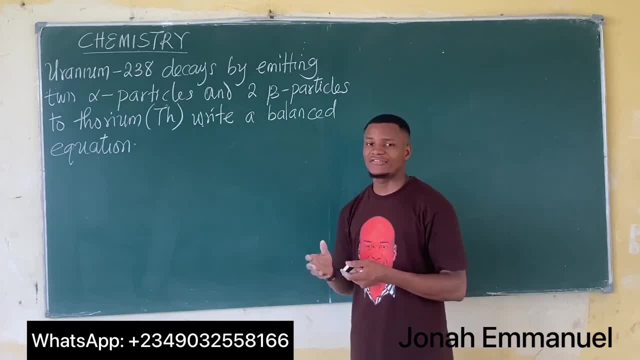 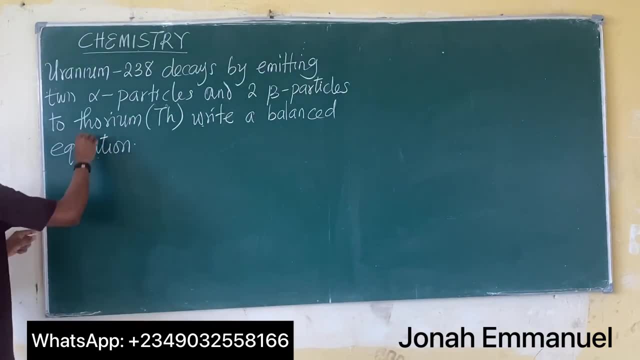 which means for a decomposition reaction is a kind of reaction where we have more products than reactants. So for this, first of all, let's get your uranium. So let's get this done, please. So for uranium, the chemical symbol is U, The atomic number, of course, is 92. 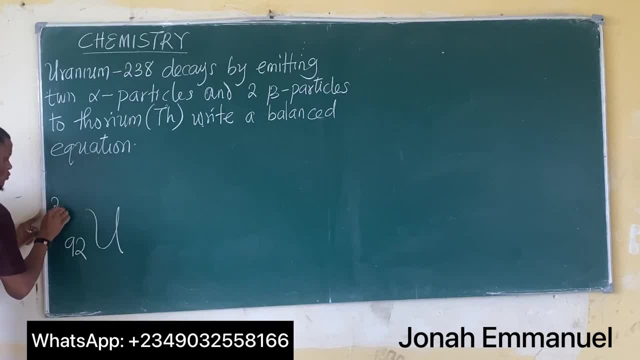 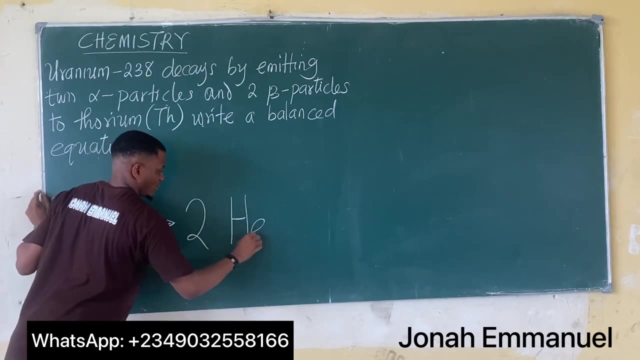 while the mass number is what you have here, So 2, 3, 8. So here this undergoes a decay to give two alpha particles, So it becomes two times alpha particles. you said they are helium, So it becomes helium. only two here, and of course four. 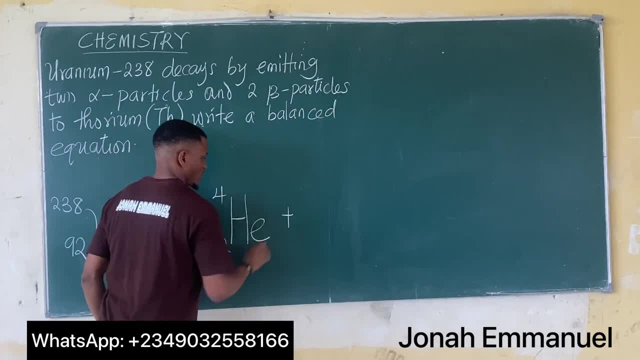 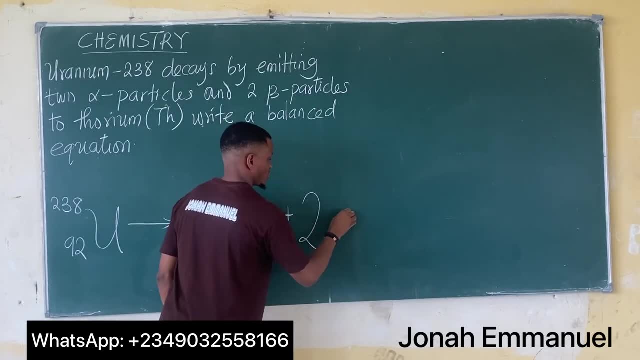 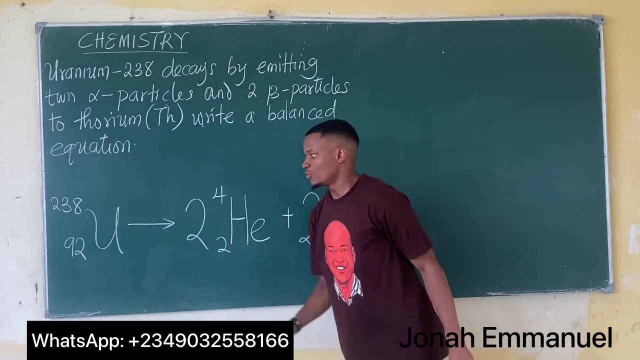 and also two beta particles. So it becomes plus two of beta particles. That should give you beta particles. you said they are electrons, So it becomes electrons. This is minus one, this is zero. So I am having uranium with atomic number 92 undergoing a decay to emit two alpha particles. 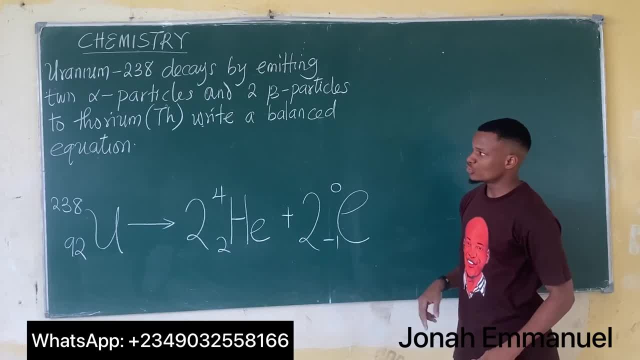 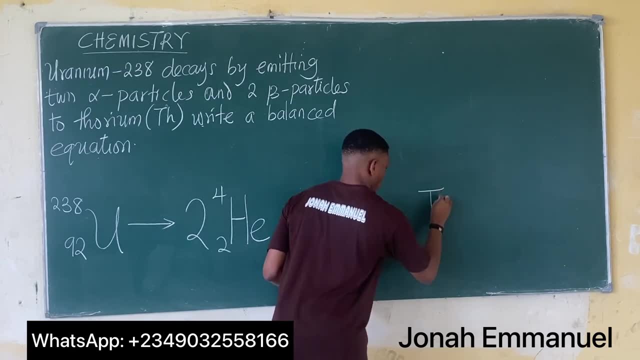 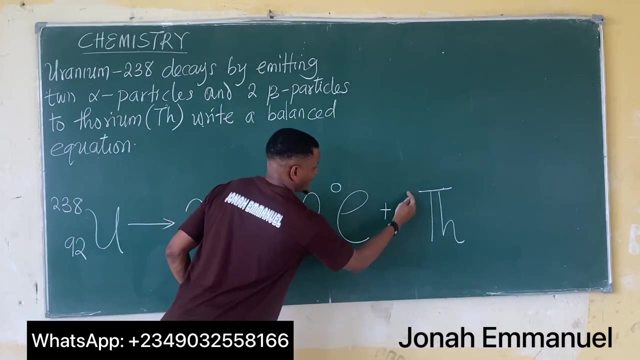 and two beta particles to form thorium 3H, So it becomes plus. Thorium should be TH, So I am having TH. Alright, Our task now would be to find the atomic number and the mass number of thorium. here Now, of course, plus obviously we have our energy. 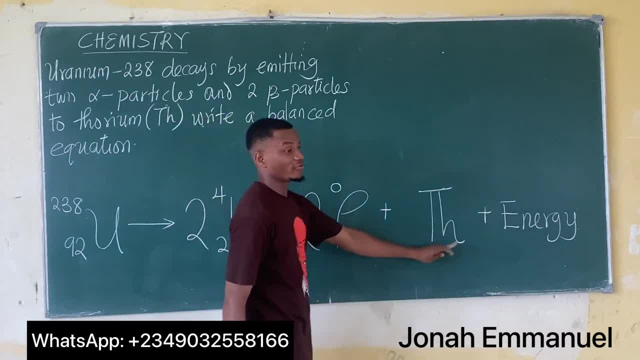 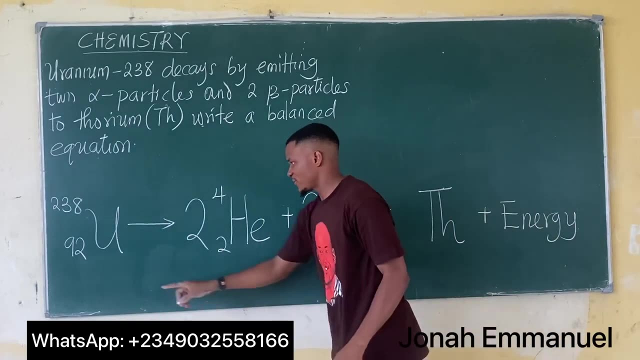 We have energy here. I have said the kind of energy released during the activity is called the nuclear energy or perhaps heat energy. So let's get the atomic number and the mass number of thorium that will be released. So let's get. So this becomes 92. 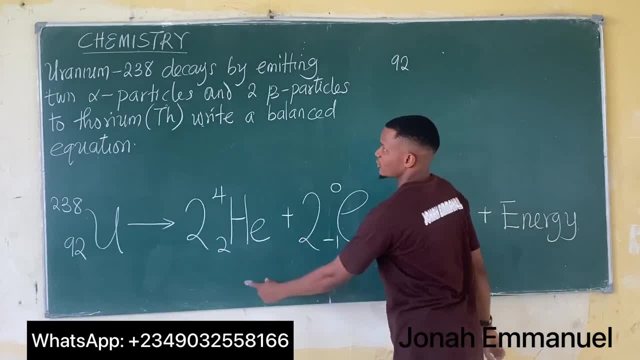 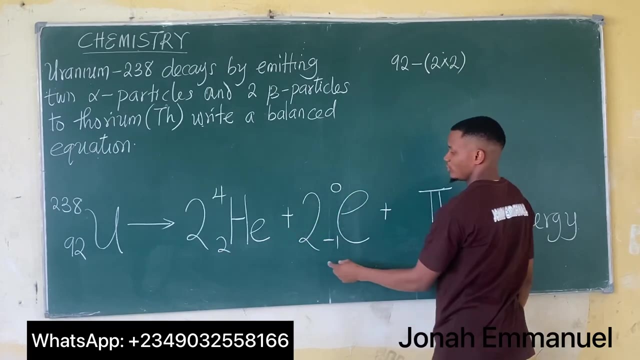 So I am having 92 For this, since this is under decay, or this integration becomes a subtraction, So it becomes minus. Let's look at alpha decay. I am having 2 times what I have here- that 2. So I am done with this one. here Come to the beta decay. 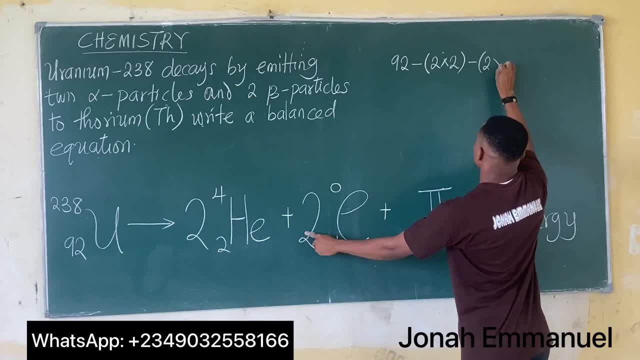 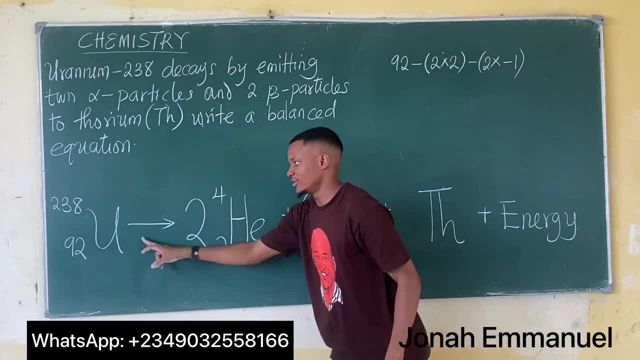 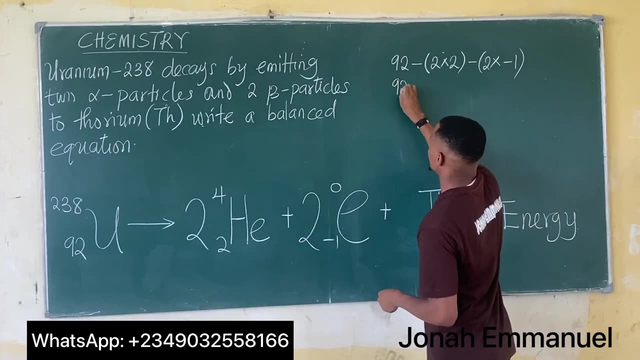 It becomes also minus what I have here, 2 times what I have here minus 1, and that's all Alright. so it becomes 92 minus 2 times 2, also minus 2 times minus 1. If I work out this much, give me 92. 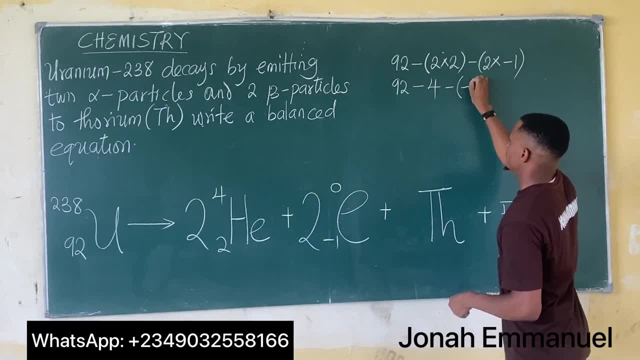 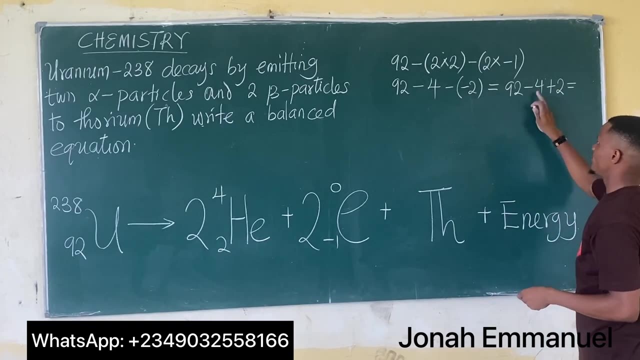 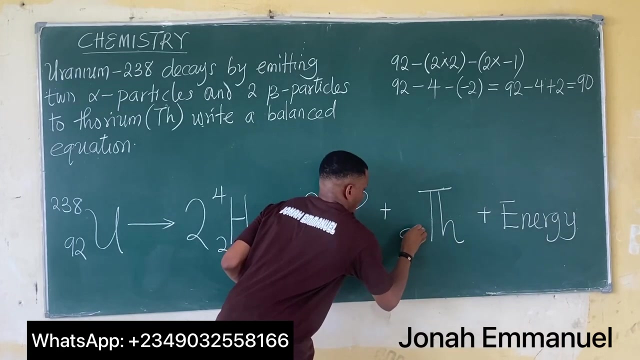 this gives you 4. This gives you minus 2. So I have this. This is equal to. I have 92 minus 4. minus minus is plus 2. So 92 minus 4 gives 88.. 88 plus 2 gives 90. I'm having here as 90. So hence for thorium the atomic number becomes 90. So I have 90 as the atomic number. 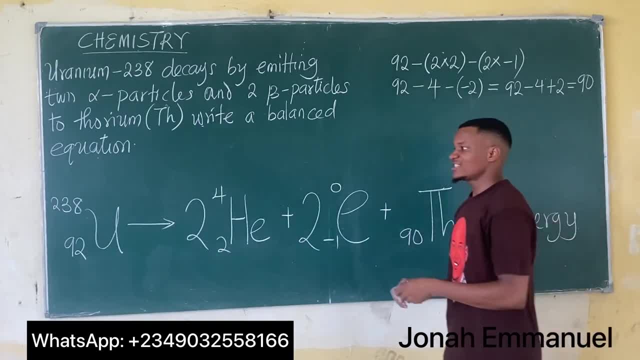 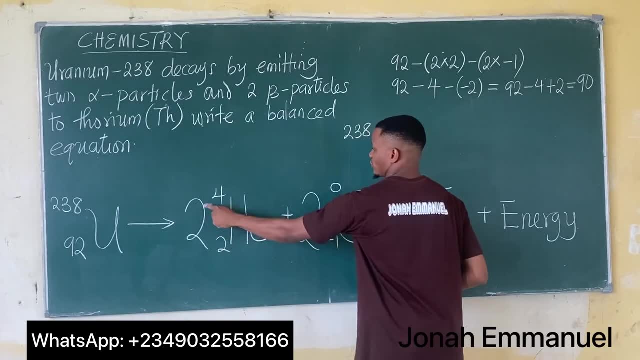 We'll do the same thing to get the mass number. So for the mass number, I have this as 2, 3, 8.. So I'm having 2, 3, 8 minus 2 times 4.. So 2 times 4, minus, this times this, 2 times 0.. 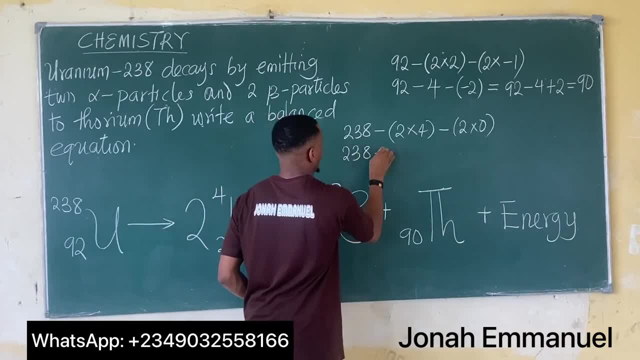 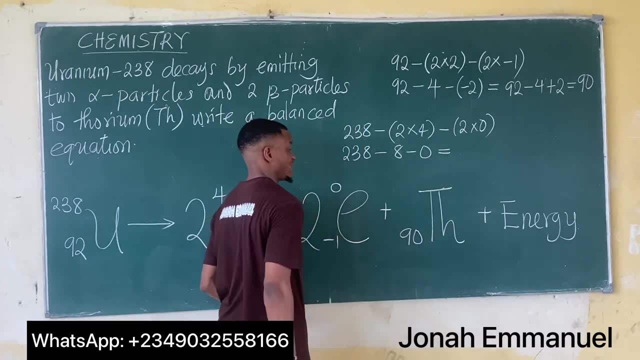 So I'm having here as 2, 3, 8 minus 2 times 4 is 8 minus 2 times 0 is 0. So I'm having 2, 3, 8 minus 8.. That's 2 times 0. 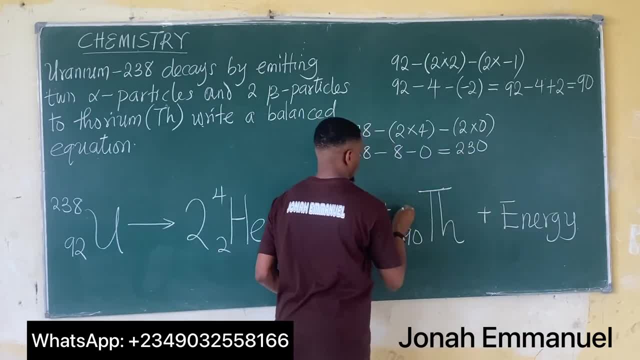 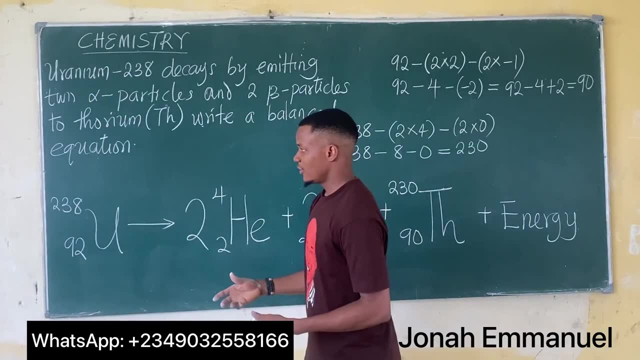 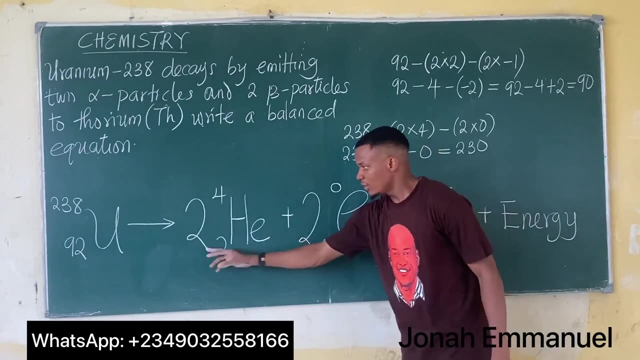 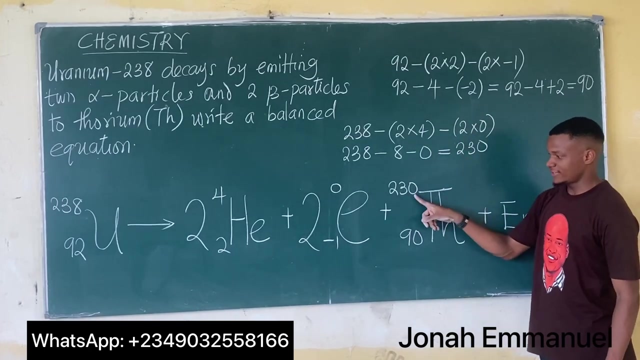 230 minus 0, that's 230.. So this gives you 230.. So this now becomes the equation of the decay, where uranium 2,, 3, 8, undergoes decay by emitting 2 alpha particles and 2 beta particles to produce thorium-230 having an atomic number of 90.. 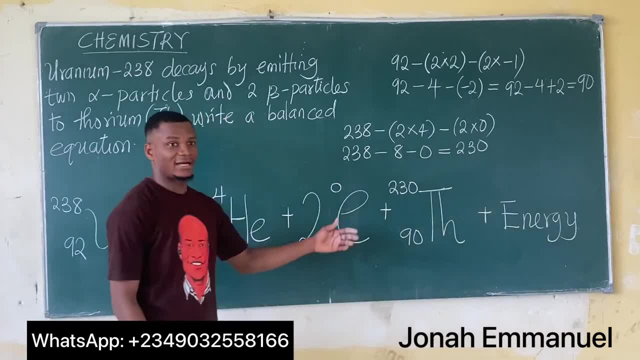 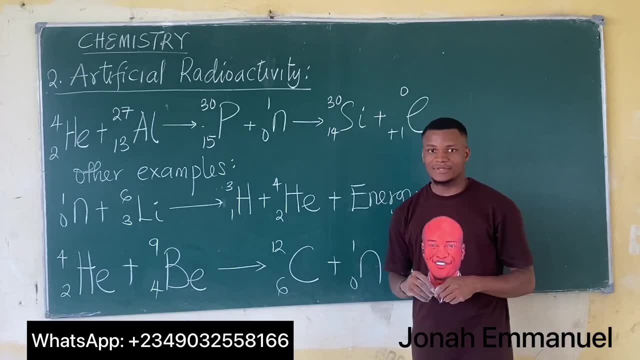 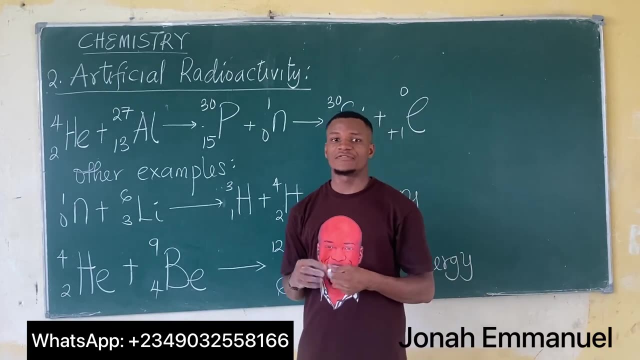 So of course we do this, We release off energy. So this is how this is done, All right, So we earlier discussed that there are two types of radioactivity: natural radioactivity and artificial radioactivity. We discussed the concept of natural radioactivity, citing instances using alpha decay and beta decay. 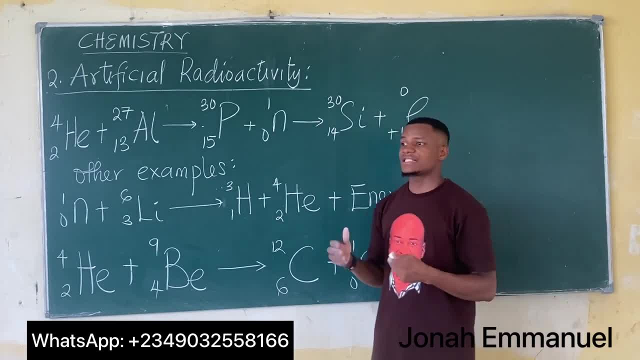 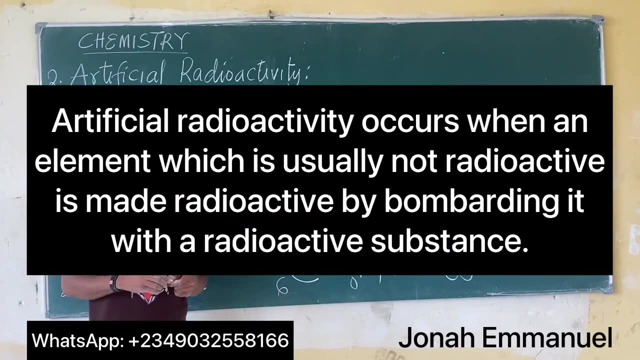 Now, when it comes to artificial radioactivity. in artificial radioactivity it is simply, we can say: artificial radioactivity occurs when an element which is usually not radioactive is being made radioactive by bombarding it with a radioactive substance. that is artificial radioactivity. 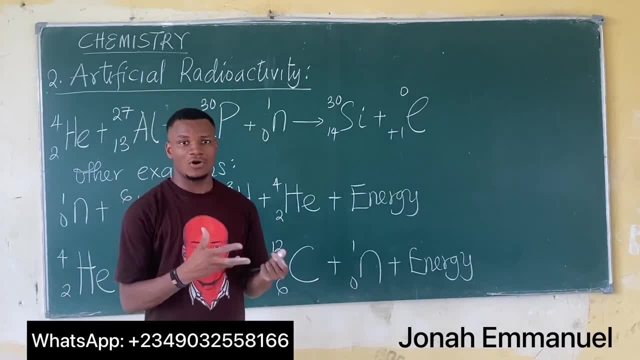 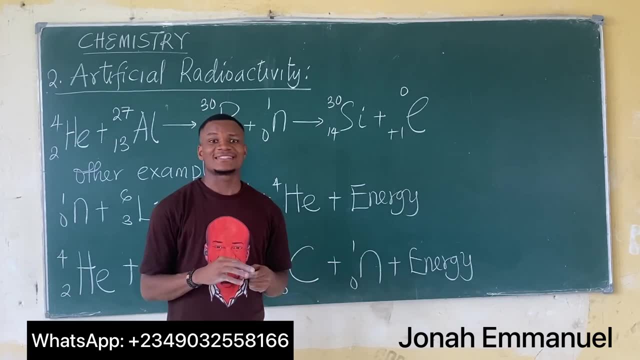 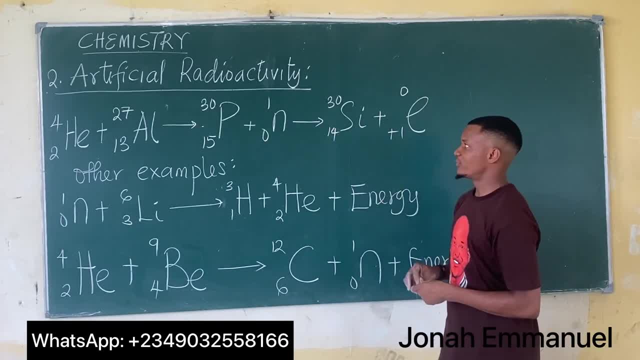 So, by definition, artificial radioactivity occurs when an element or a particle which is usually not radioactive is made radioactive by bombarding it with a radioactive substance. that is artificial radioactivity. electron which, on further decay, produced silicon-14 or silicon-30, having 14 as its atomic number. 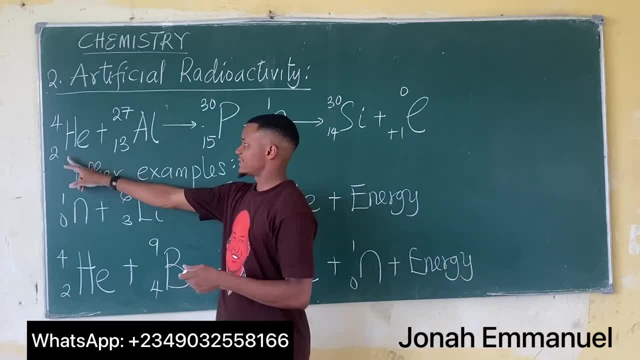 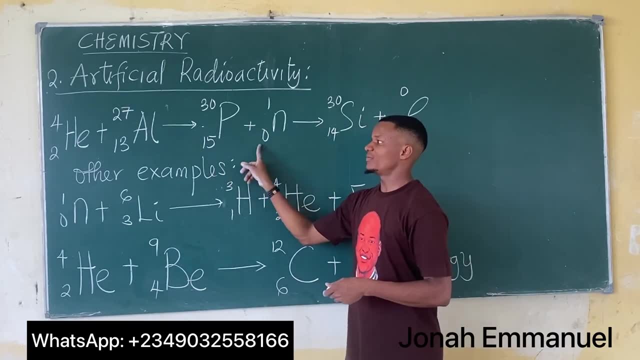 Now, if you look at this one here, for this for the left hand side, for this one here, total atomic number is 15.. Here, 15 point plus zero, Total atomic number is 15.. Here the same thing. Now see the trick here. alright, So in this case now, the electron now becomes: 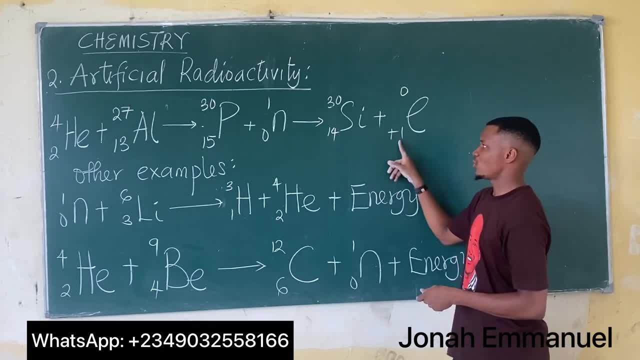 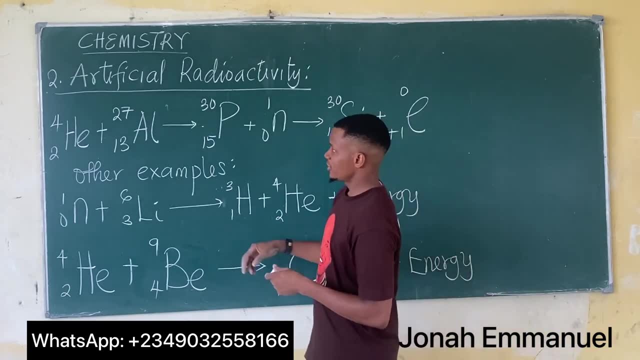 a plus one, such that I'll have 14 plus one, giving you a balanced 15 as your atomic number For this one. here I have this as 31,. alright, So this is called. this is 31.. The mass number: 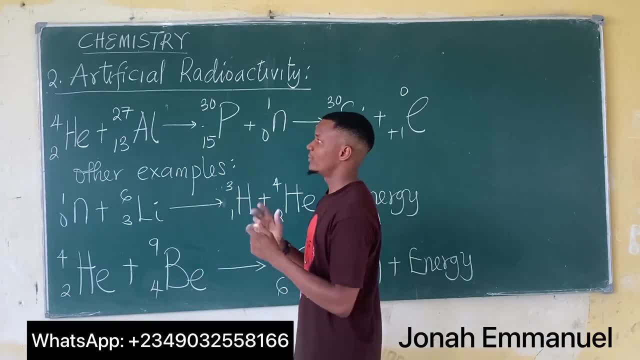 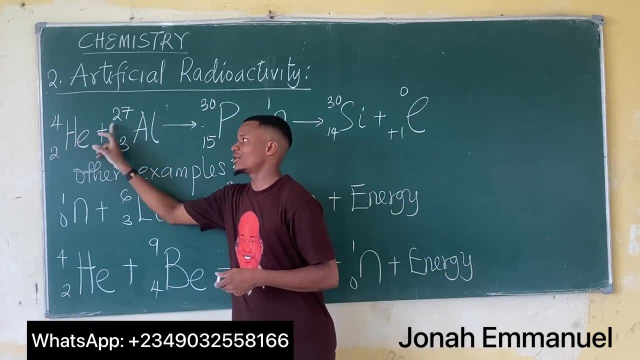 combined 14 to the 7 gives you 31. combined. Same thing here: 30 plus 1, that gives you 31.. So for these two mass number: here total mass number is 31.. Here total mass number. 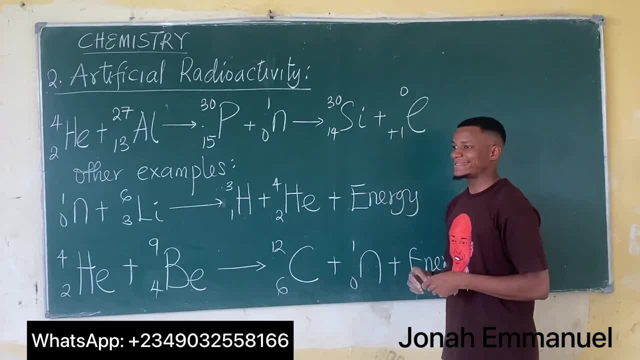 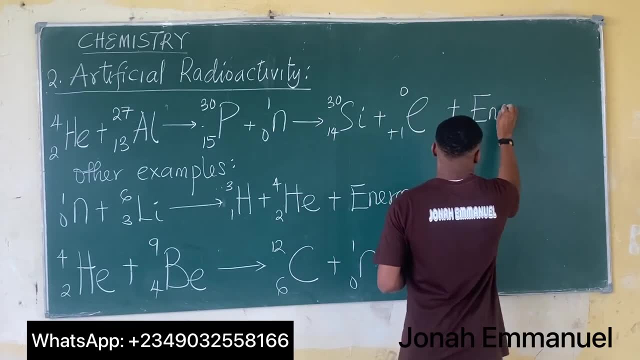 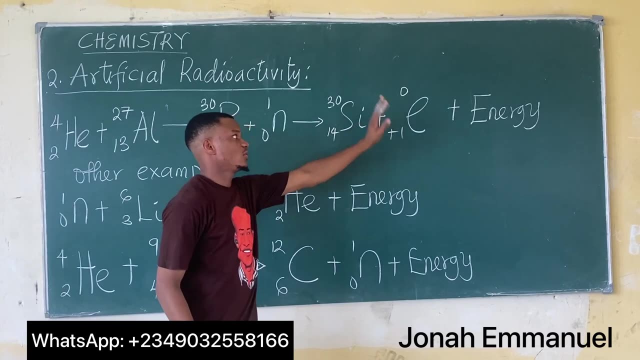 is 30. So we can see some bit of energy right is being lost. It's being lost in this process. So you can see here: energy is being lost at this point here. alright, So the mass number is gone, Alright. so some other examples of artificial relativity in: 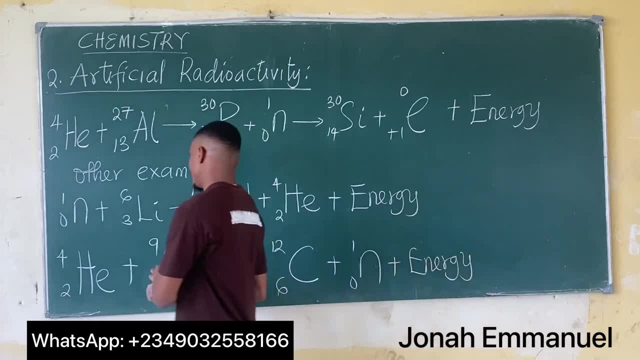 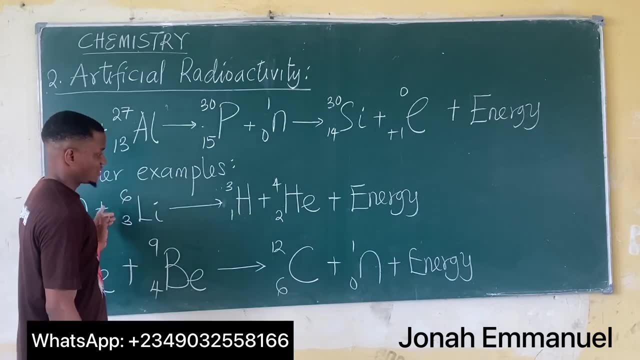 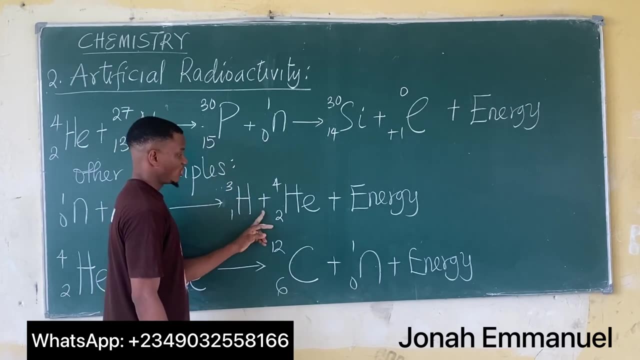 place what you see here For this one. here I'm bombarding lithium. alright, Lithium is a lithium atom with a neutron, such that it's now decaying into you. have tritium here. Tritium is an isotope of hydrogen being combined with helium. That's alpha particle plus energy. 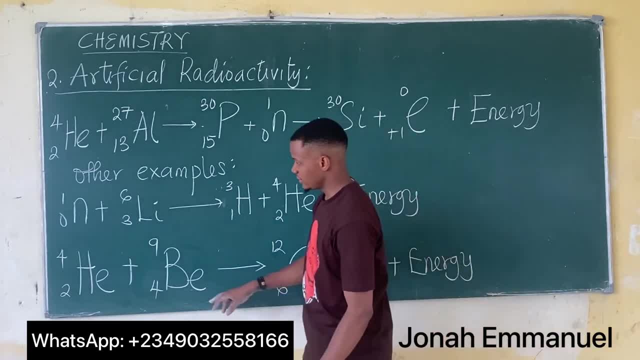 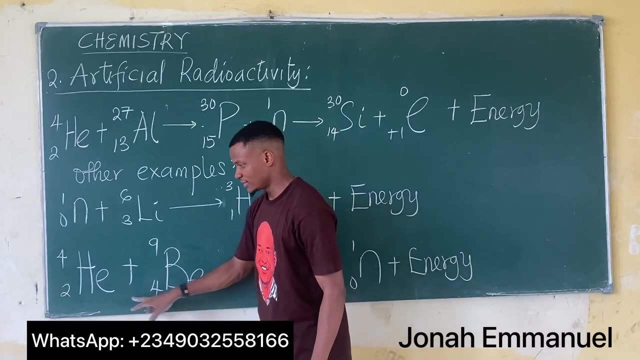 Same thing here For this one. here I'm bombarding for this one. here the element that is not radioactive is lithium. here Same thing here for this one: the element that is not radioactive is beryllium. But I will now go back. I will now combine beryllium with my alpha particle, which is helium. 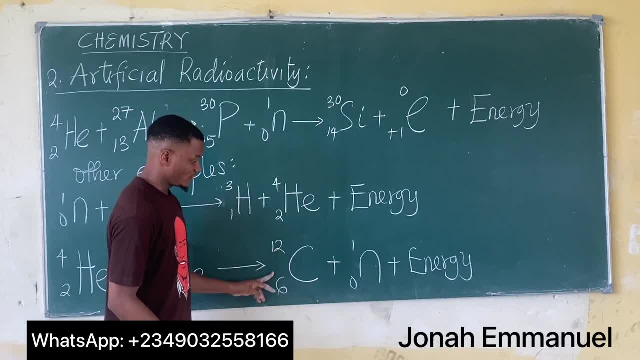 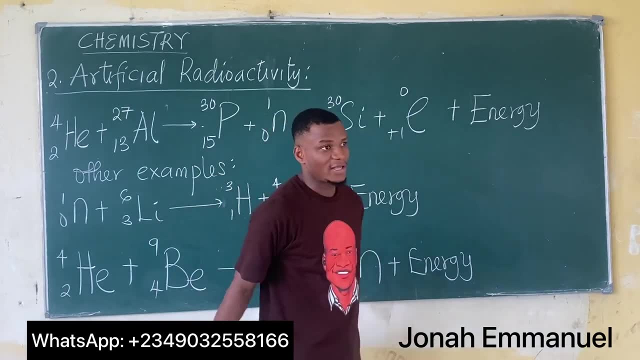 It will now produce carbon, alright, carbon-12, with neutron and, of course, plus energy, Alright. so these are examples of artificial radioactivity. That's a case where non-radioactive elements, such as aluminium, such as lithium, such as beryllium, is now being made into. 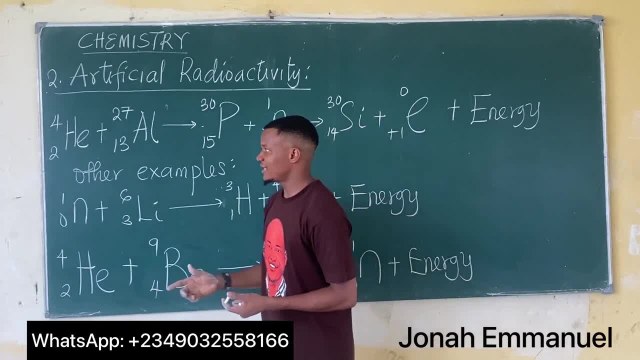 radioactive by combining them or bombarding them with radioactive particles. okay, Helium, neutron, of course, helium. So this explains the concept of radioactivity. Now, next up, we'll look at what is called radioactive isotopes or radioisotopes. 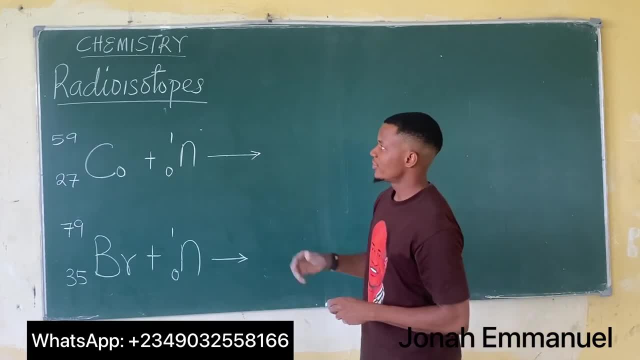 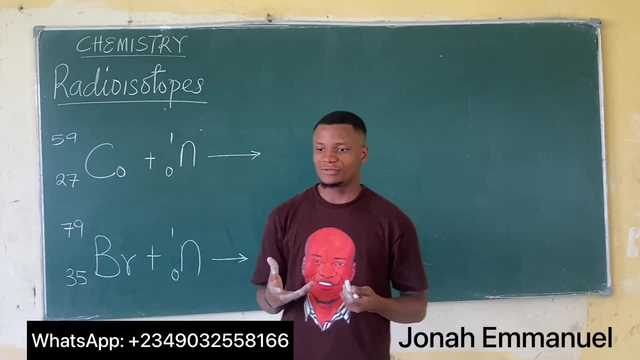 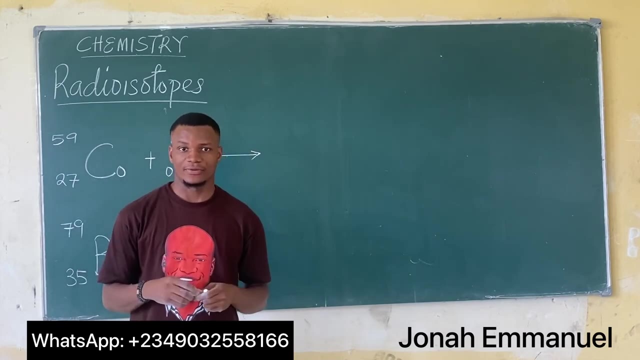 Alright, so let's look at the concept of radioisotopes. Radioisotopes are simply isotopes of elements that are formed by bombarding certain elements with a neutron, a proton or a deuterium. alright, So when it comes to radioisotopes, they are simply isotopes that are formed artificially. 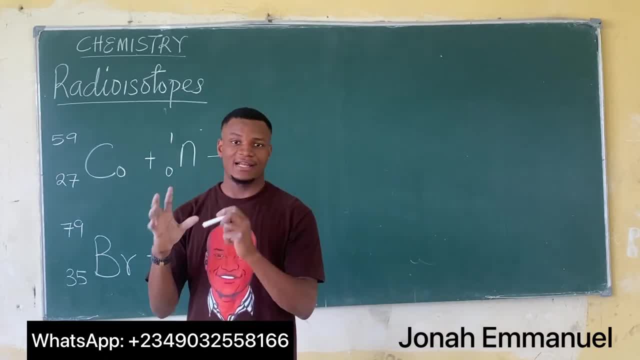 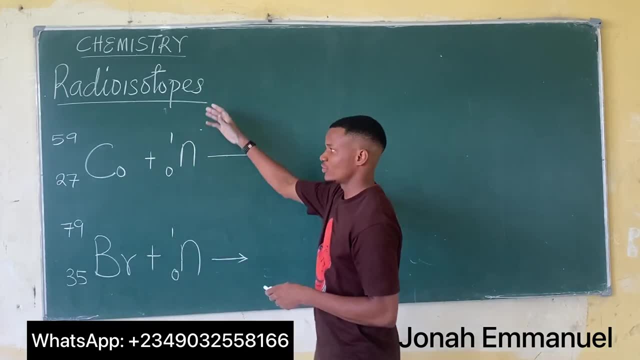 by bombarding a particular element with either a proton, a neutron or a deuterium. That's the simple idea of radioisotopes. Now, for instance, we have these two things: We have cobalt here, we have bromine. Now, if I bombard cobalt-59 with a neutron, 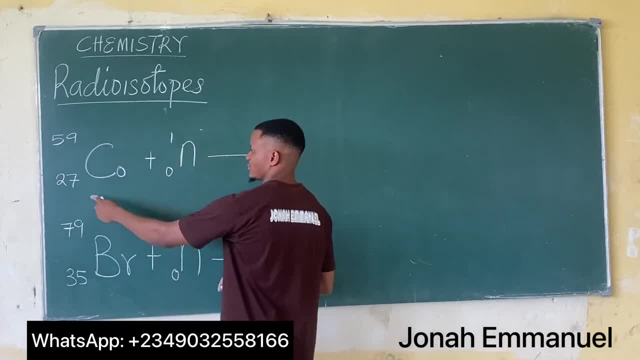 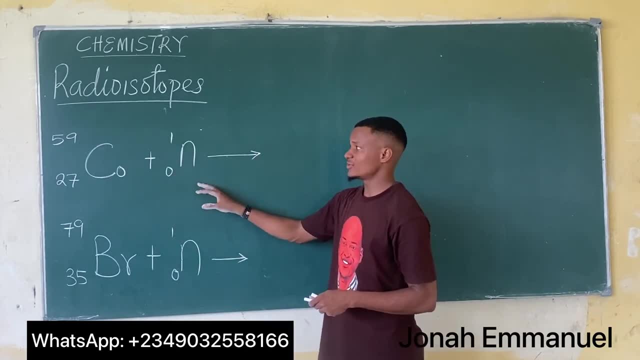 from here. if these two are combined, of course, looking at atomic number, it comes to the 7 plus 0. Now, in this case I'm not subtracting because this is not a decay In this case. now you can see that there is a combination there, So I'm going to add up all of them. 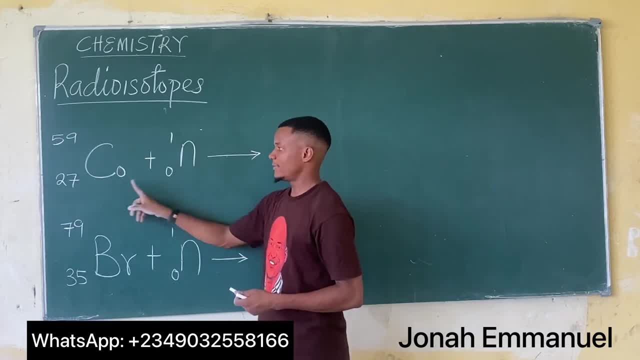 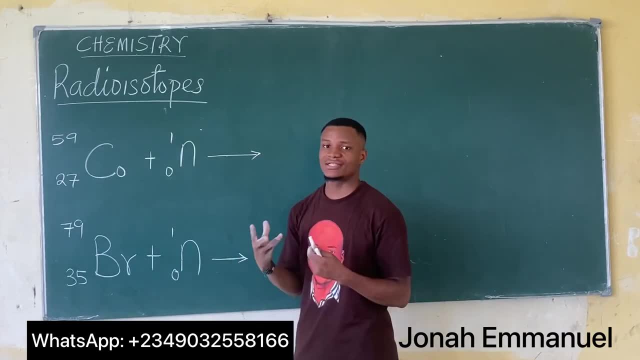 So I'm going to add up all of them. So I'm going to add up all of them. I'm going to add up the atomic number and not subtract. So if I add up the atomic number, it becomes 27 plus 0, which is 27.. 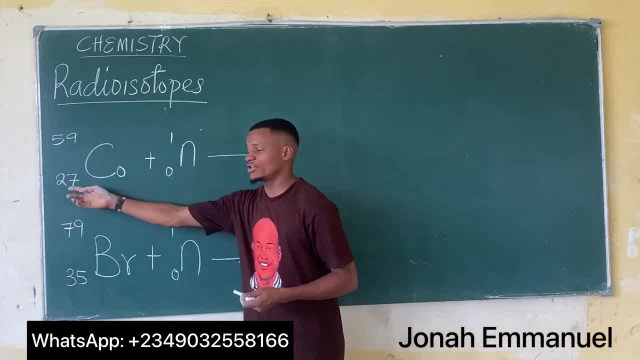 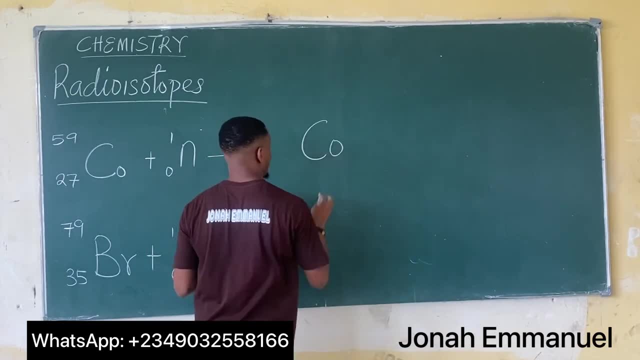 So a new element of atomic number 27 is formed, which of course is the same element, That's cobalt. So I'm having cobalt here with atomic number 27.. Also for the mass number. I'll simply sum up this and this: 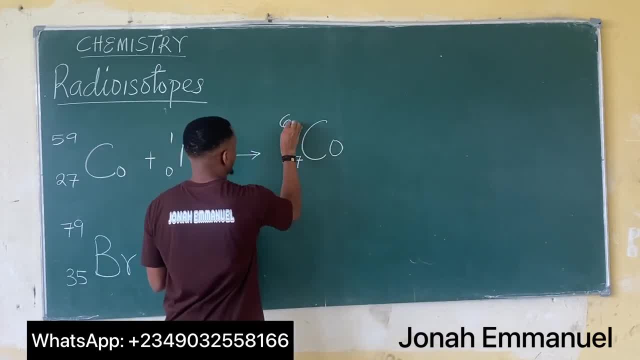 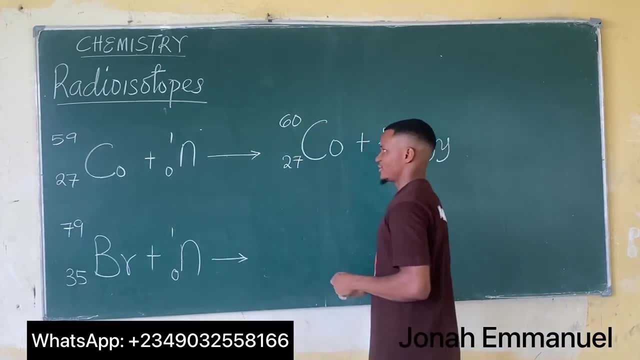 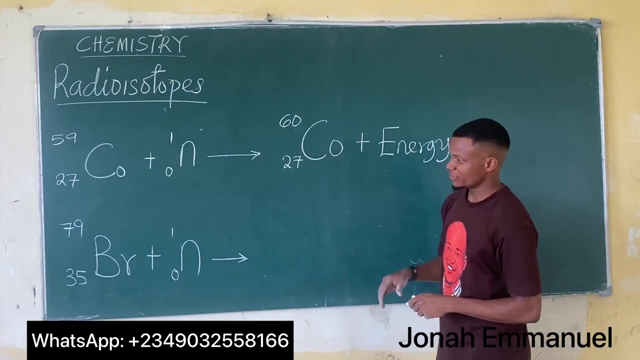 So it becomes 59 plus 1. That's 60. So I'm having cobalt 60. And of course, with the release of energy, With the release of energy, So this becomes a radioisotope, That's an isotope of cobalt, It's a radioisotope. 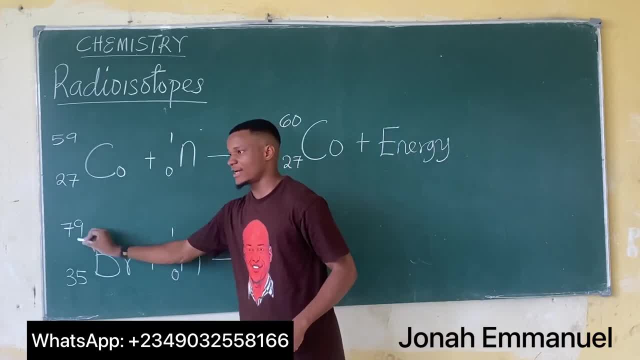 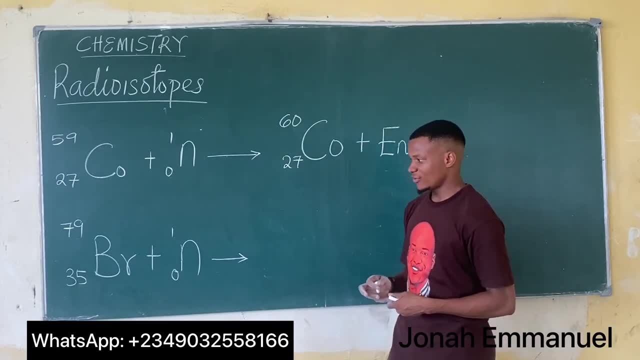 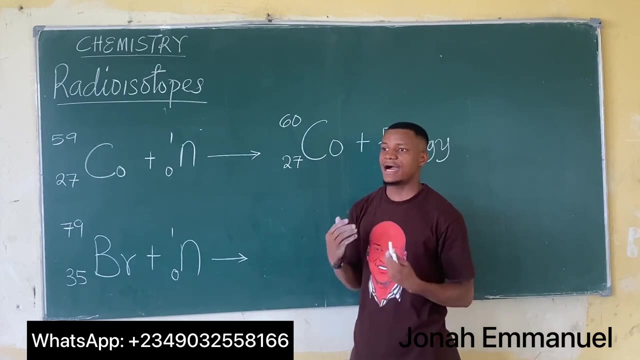 And for this one here I'm having bromine- bromine-79, combining with a neutron. So if I combine this, of course, for the atomic number it becomes 35 plus 0, which is state 35. So an element of atomic number 35 is being formed. 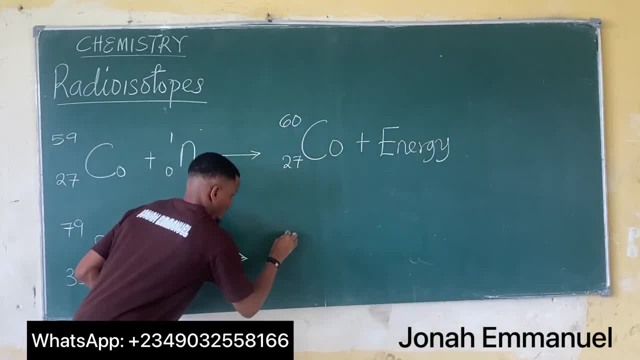 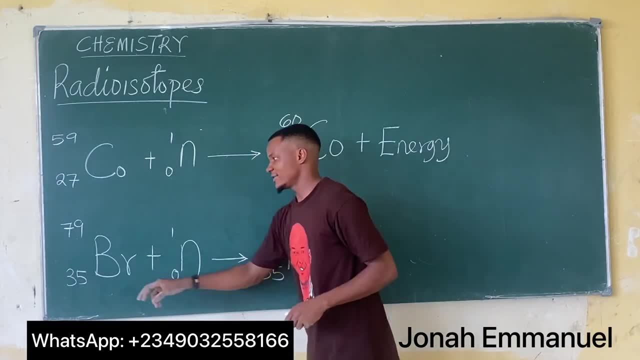 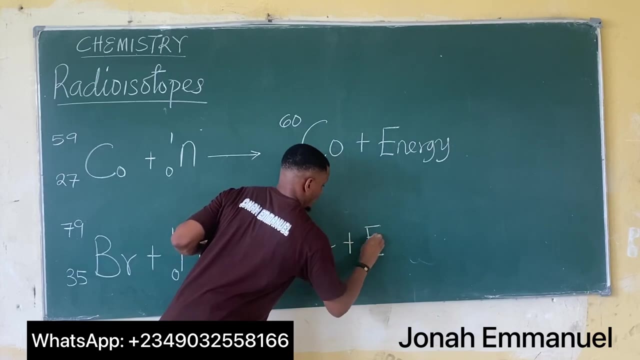 which of course is still bromine. So I have bromine here, So bromine with atomic number 35. For the mass number combined is 79 plus 1. That gives you 80. And of course, plus the release of energy. 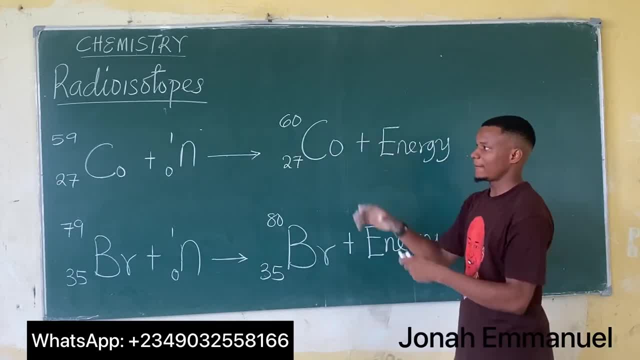 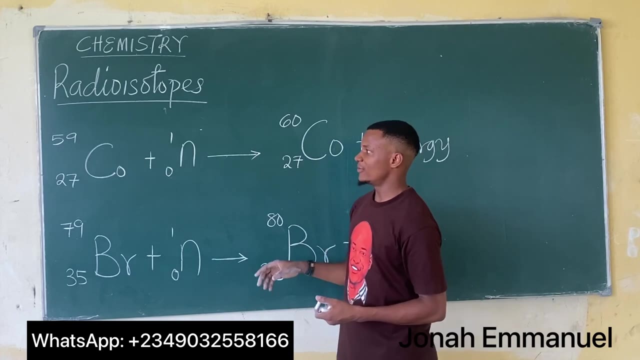 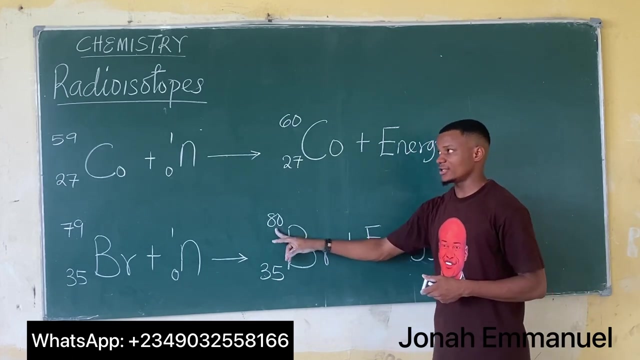 Now energy is being released. So these are equations that show the concept of radioisotopes. So cobalt-60 is a radioisotope of cobalt-59, because it was got by combining cobalt-59 with a neutron. Also in the same sense, bromine-80 is a radioisotope of bromine. 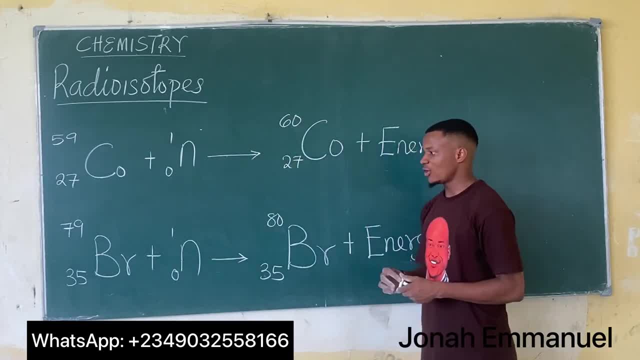 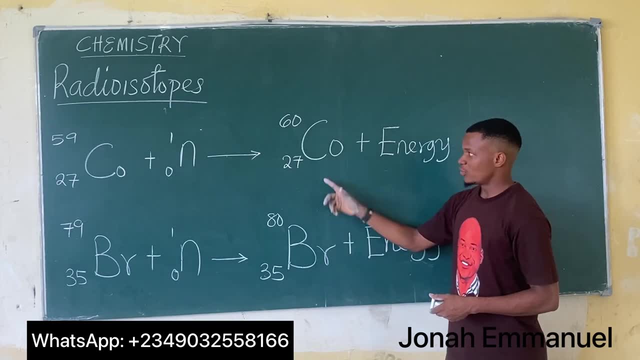 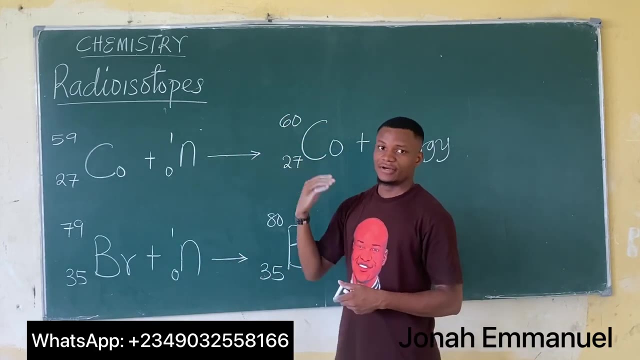 or, for example, bromine-79, because it is got by combining bromine-79 by neutron. So you can see, cobalt-60 and bromine-80 are both radioisotopes of cobalt and bromine respectively. 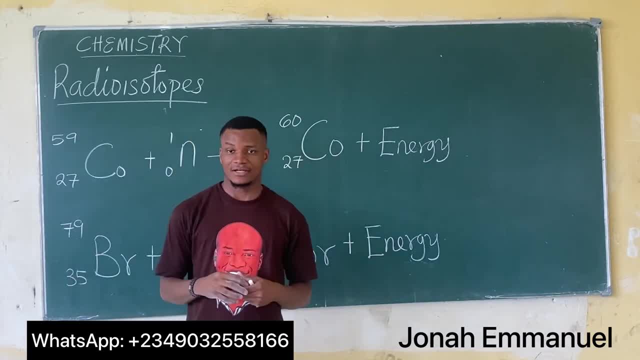 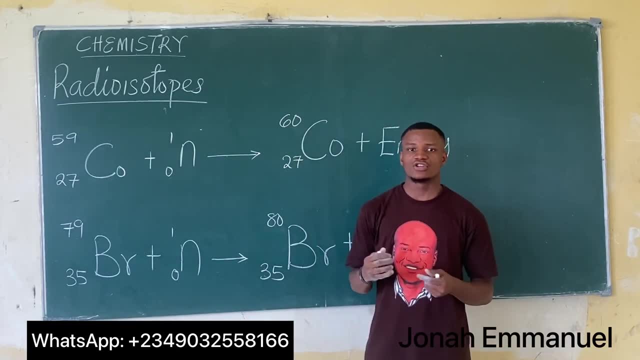 So this is just a simple concept of radioisotopes. This is just a simple concept of radioisotopes. Next up, look at nuclear energy and the concept of nuclear fission and nuclear fusion. Alright, so let's look at the next concept there, called nuclear energy. 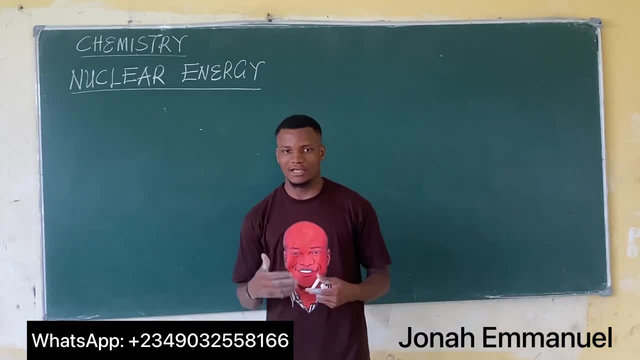 Now most likely what you look at. if you refer back to our equations on alpha decay, beta decay and etc. you observe that at the end of each radioactive equation or radioactivity equation, you observe that there's something called plus energy. 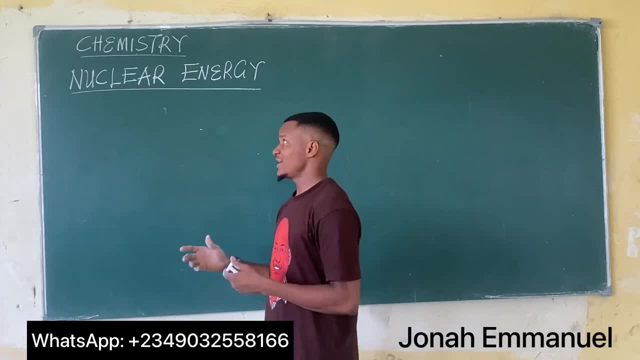 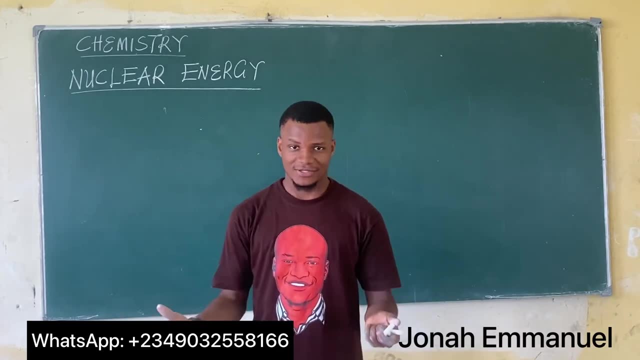 There's always a plus energy there. So what's that plus energy? That's energy that is called a nuclear energy. What's a nuclear energy? A nuclear energy is simply the energy that is released or given off during a radioactive process. 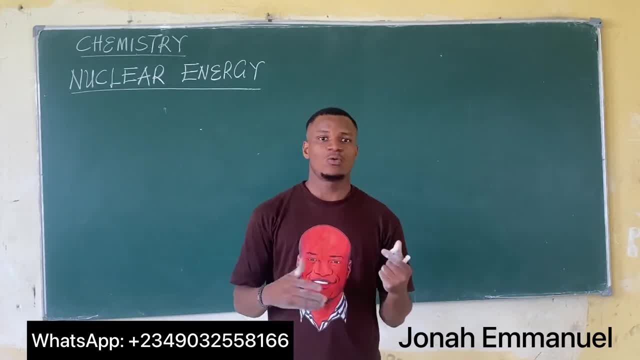 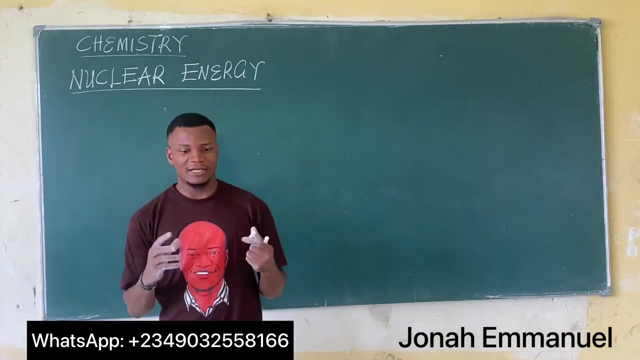 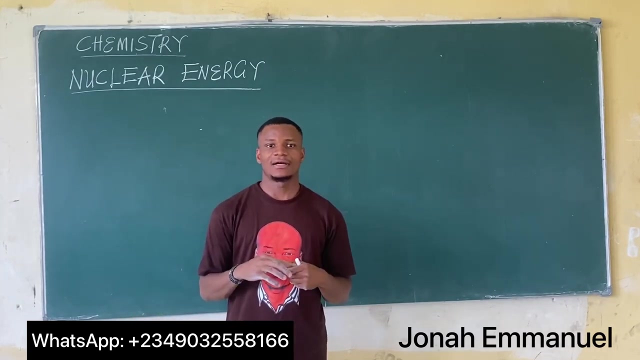 or during radioactivity. So when there is a radioactive process or when radioactivity takes place there, energy is being given off. That energy there is called a nuclear energy We talked about. I just mentioned the concept of radioactive process. Basically there are two basic radioactive processes. 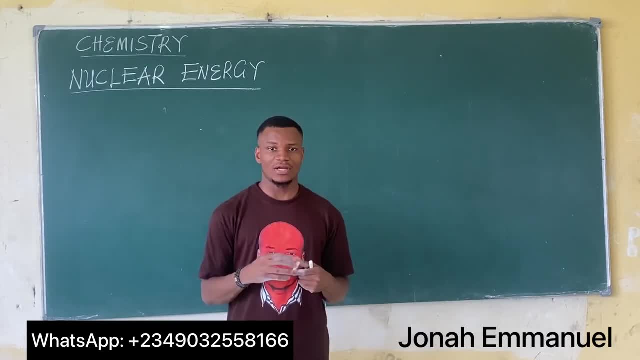 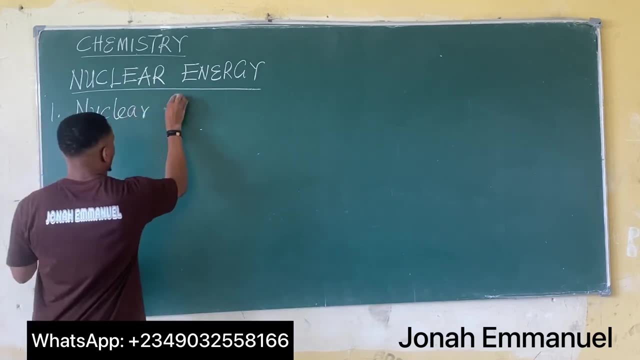 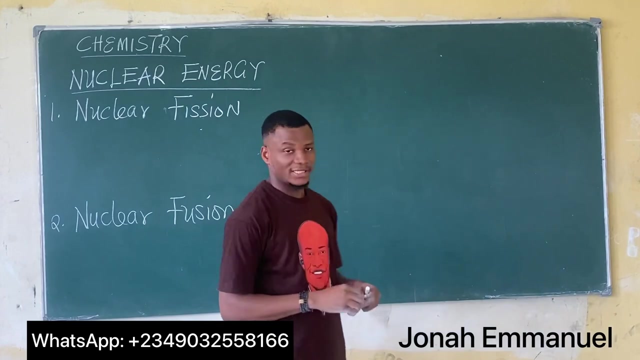 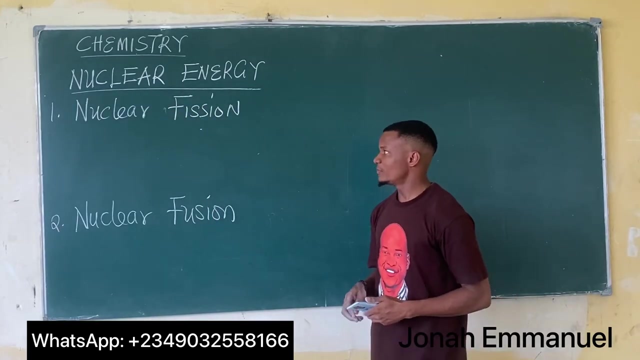 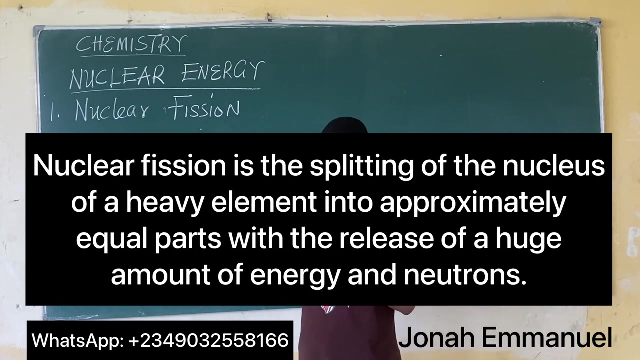 which includes nuclear fission and nuclear fusion, The two big ones. all right, So nuclear fission and nuclear fusion are two basic radioactive processes. All right. So by definition, nuclear fission is simply the splitting up of the nucleus of a heavy element. 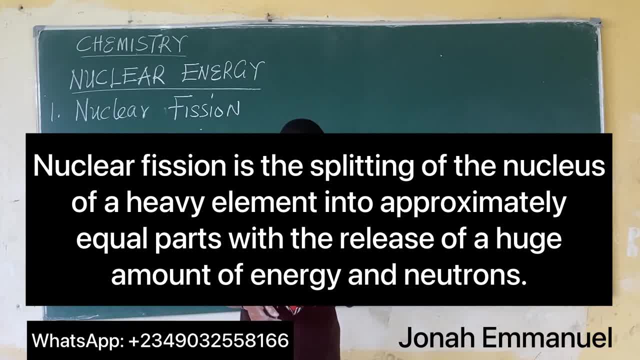 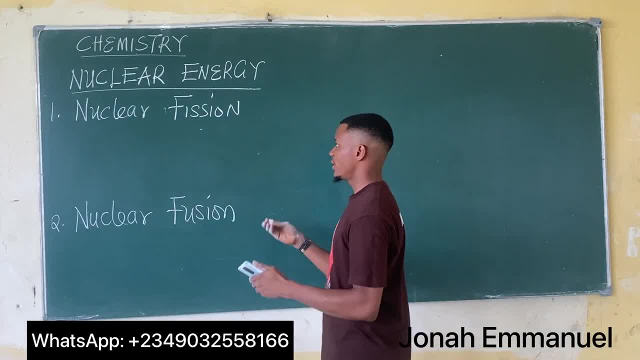 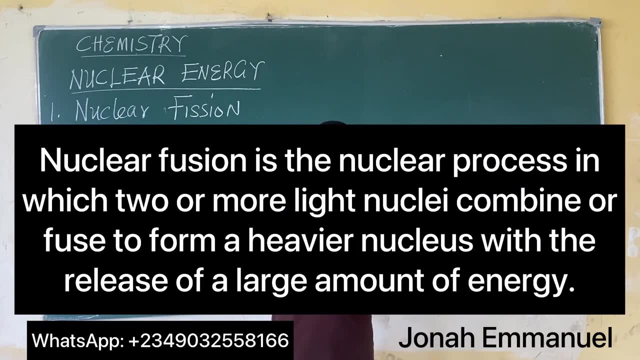 into approximately equal parts, with the release of a huge amount of energy and neutrons. So that's the definition for nuclear fission. Let's look at nuclear fusion. By definition, nuclear fusion is simply the nuclear process in which two or more light nuclei 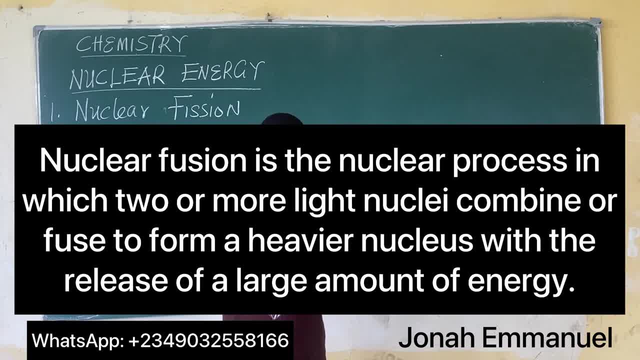 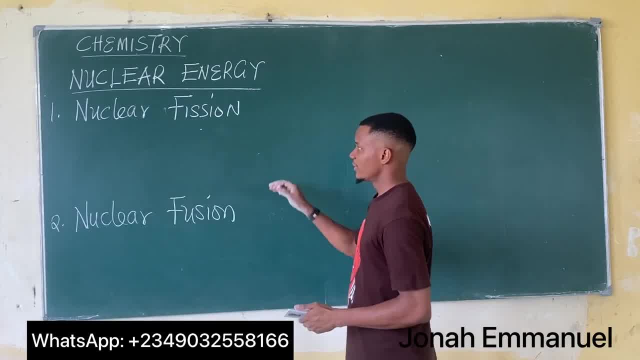 combine or fuse to form a heavier nucleus with the release of large amounts of energy. All right, So look at some, very just look at. we use one nuclear or radioactive equation to explain two of them. All right, Okay. So this is one example each. 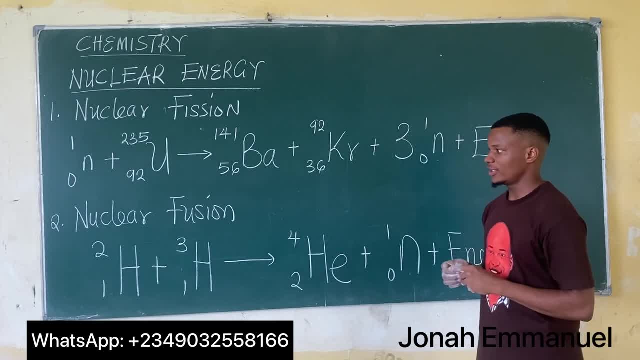 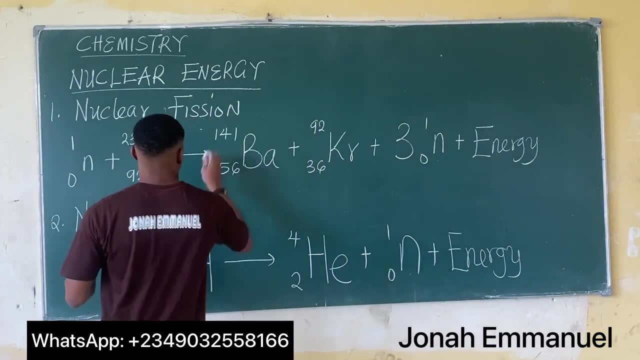 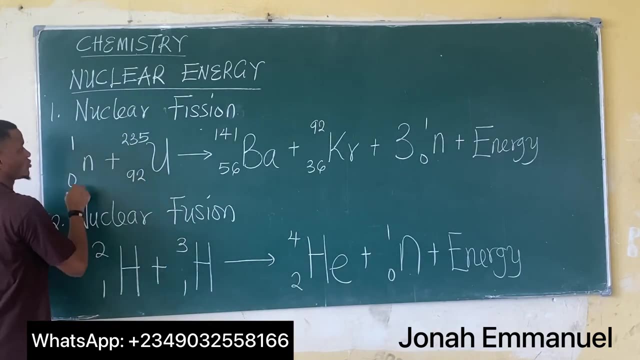 for nuclear fission and nuclear fusion- All right. Nuclear fusion, nuclear fission- All right, Let's start with this. This is smaller, Okay, All right, Let's start with this, For here I have a neutron being bombarded by. 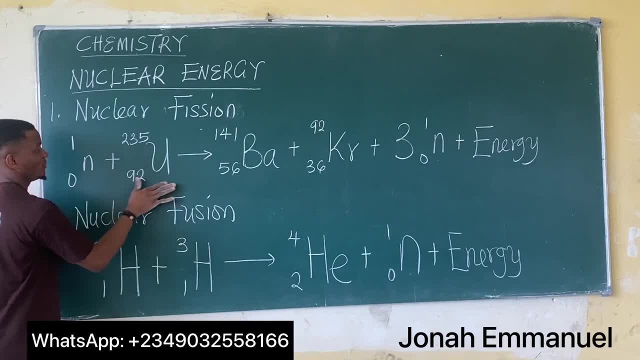 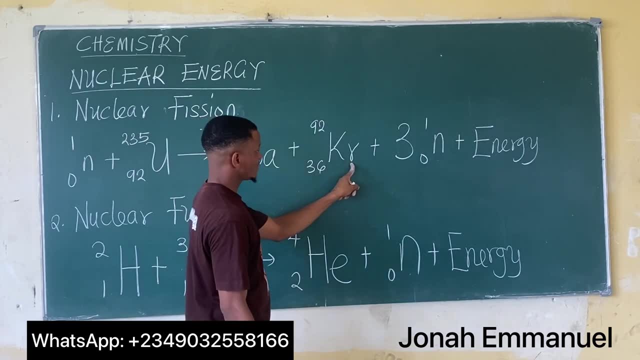 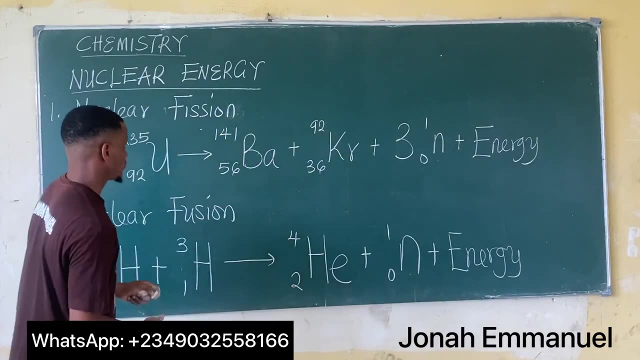 or bombarded with uranium to produce barium, barium 141,, barium 141,, krypton 92, and three neutrons, of course, release of energy. So this is an example, an example of a nuclear fission. 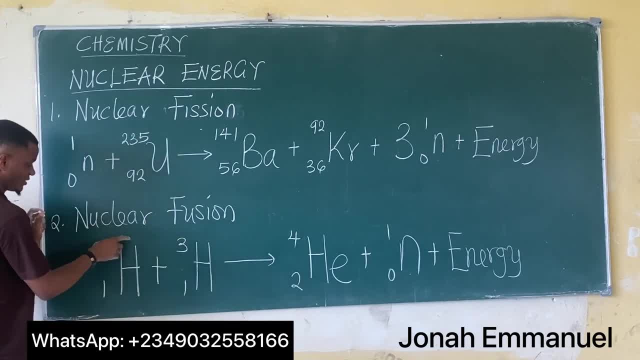 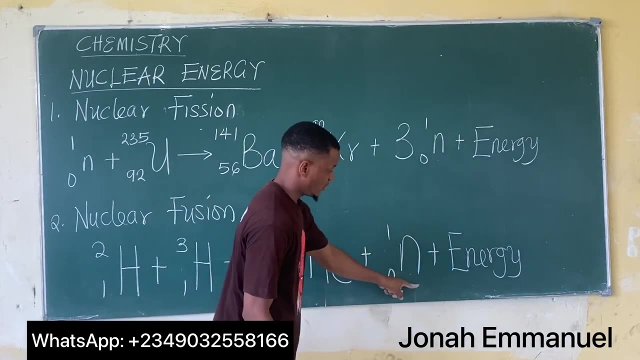 All right For the nuclear fission I have. this is deuterium, That's an isotope of hydrogen, being combined or being bombarded or being combined with tritium to produce the helium molecule with, of course, your neutron. 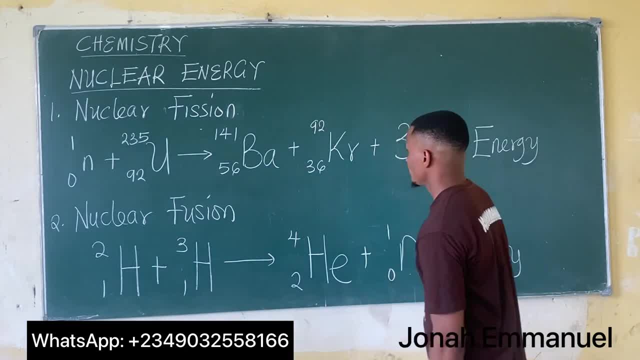 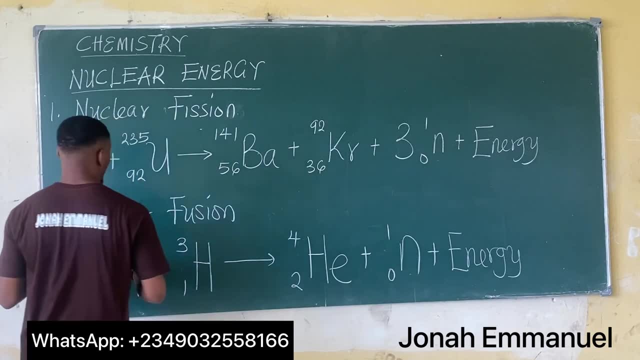 of course, with the release of energy. Now, if I try to, if I try to look at the atomic number and mass number involved for the left-hand side of the equation, for other nuclear fission, for the left-hand side of the equation, 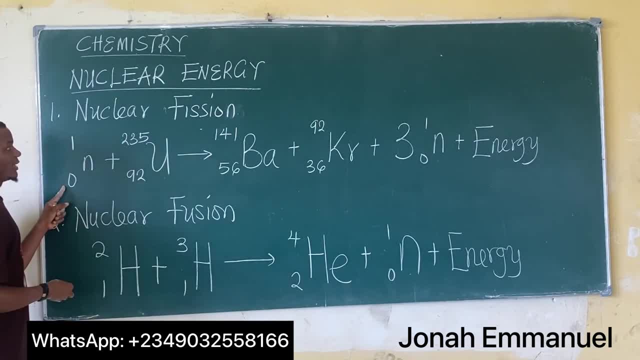 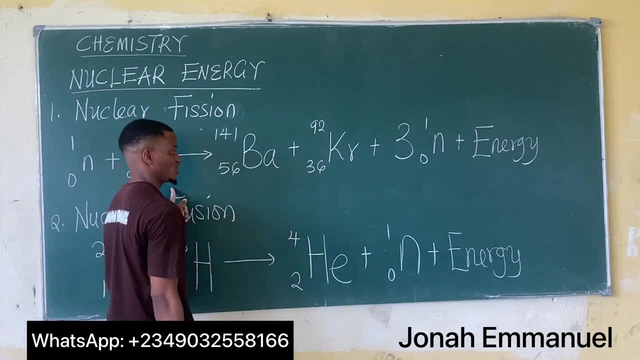 if I try to sum up the atomic numbers, I have 0.92,, which is 92.. For my right-hand side of the equation, I have 56 plus 36,, which is about 92, plus 3 times 0,. 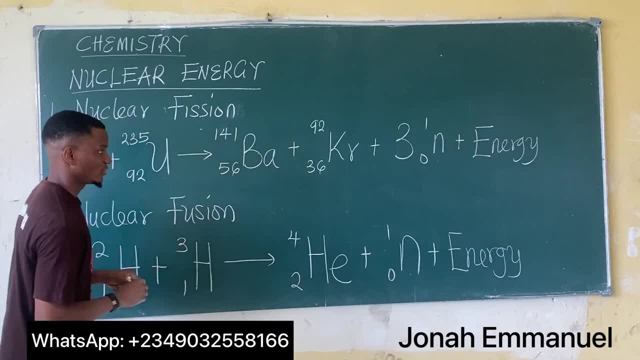 which is 92.. So this is a balanced reaction or equation, because I have in the left-hand side of the equation I have 92 total atomic number. On the right-hand side I have 92 total atomic number If I look at the mass number. 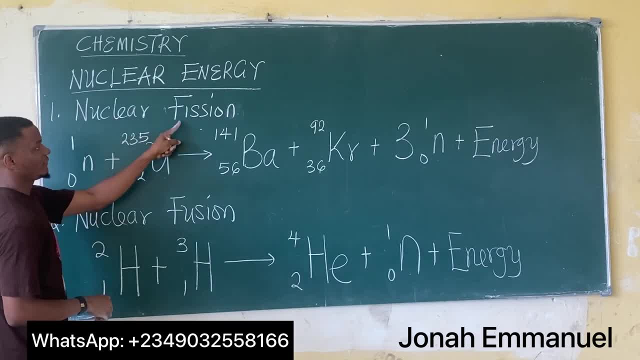 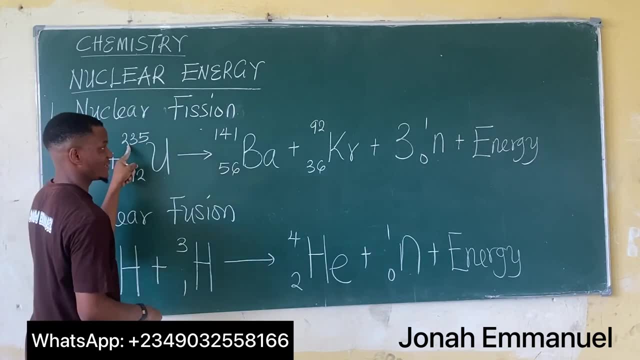 for the left-hand side of the equation, other nuclear fission. for the left-hand side of the equation I have 1 plus 235, which is 236 in total. If I look at this, this becomes 141 plus 92,. 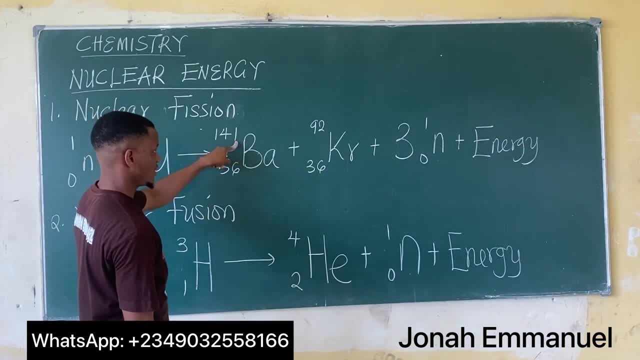 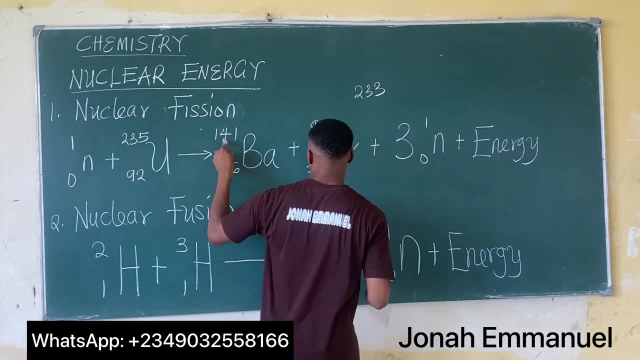 that's about 233, right, 233 plus 3 times 1,, so it's 233.. If I combine 141 plus 92, also combine these two 3 times 1,, that's 3.. That gives you 237.. 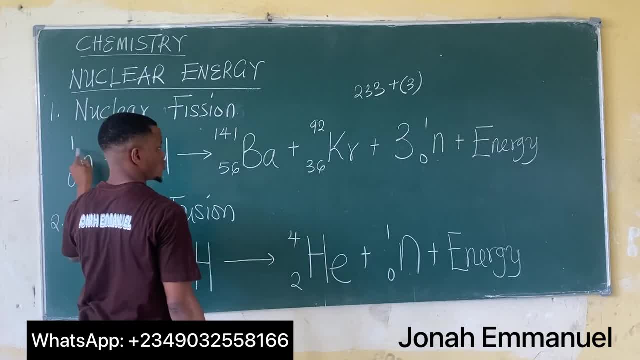 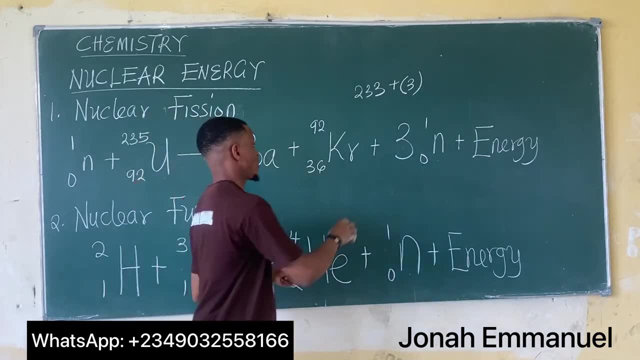 That gives you 236.. So I have here in total 236 as the total mass number Here. so I also have 236 as the total mass number. So this is a complete, or this is a balanced equation of nuclear fission. 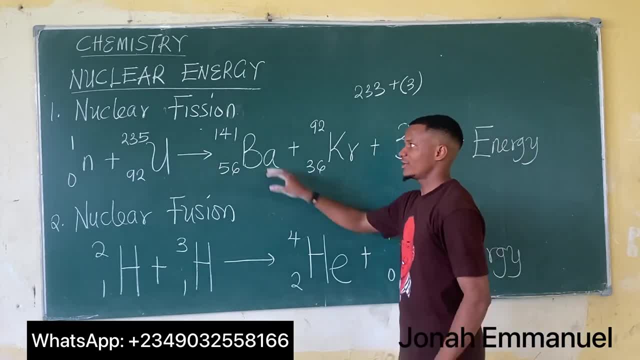 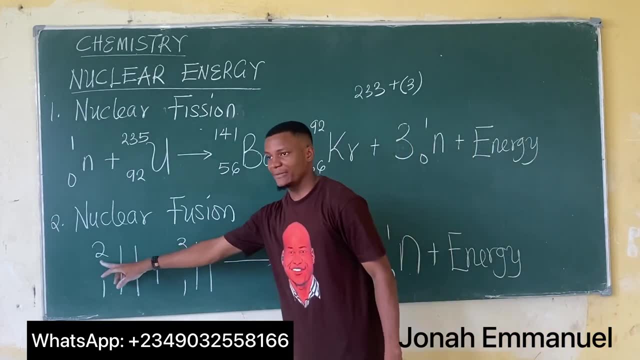 If you look at nuclear fusion here, right, nuclear fission and nuclear fusion. if I look at the nuclear fusion reaction here, this is 2, in terms of mass number, this is 2 plus 3.. So totally on my left hand side. 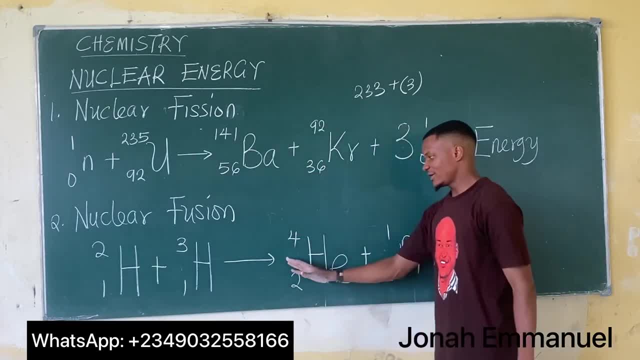 I have 5 as the total mass number. If I look at the right hand side of the equation, I have 4 plus 1, that's 5 as the total mass number. Also, if I consider atomic number, I'm having 1 plus 1,. 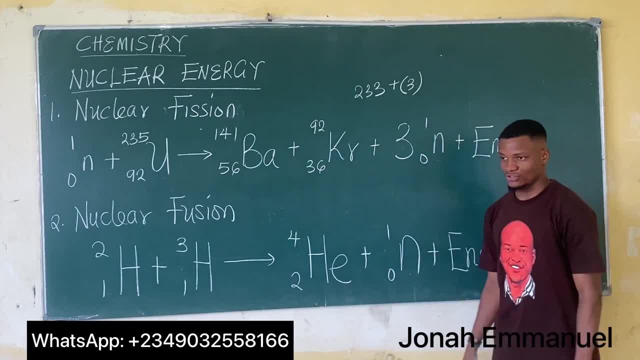 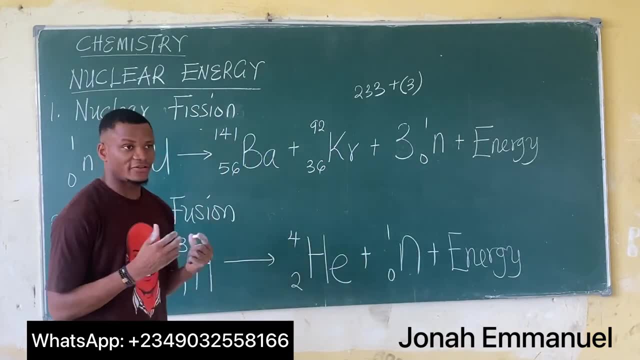 which is 2.. From here, 2 plus 0,, which is 2.. So it becomes a balanced radioactive equation. Now how do you easily know the difference between a nuclear fission and a nuclear fusion? What's the difference between them? 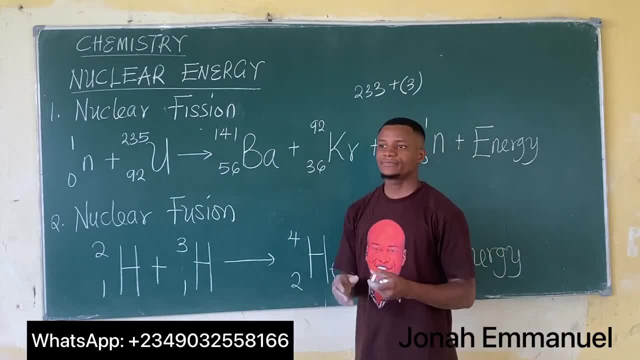 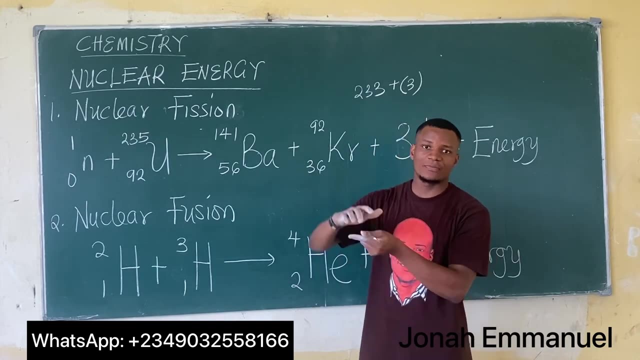 The idea is simple: For a nuclear fission, I have a bigger element that's been split into smaller ones, Alright- While for a nuclear fission, I have smaller elements being combined to form a bigger one. That's the idea, Alright. 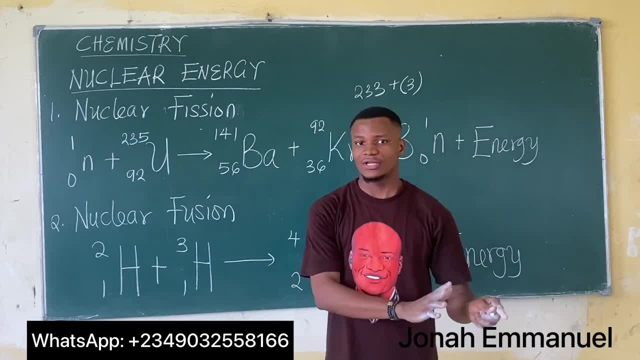 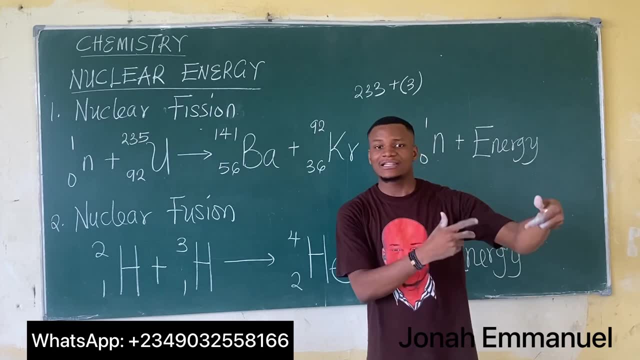 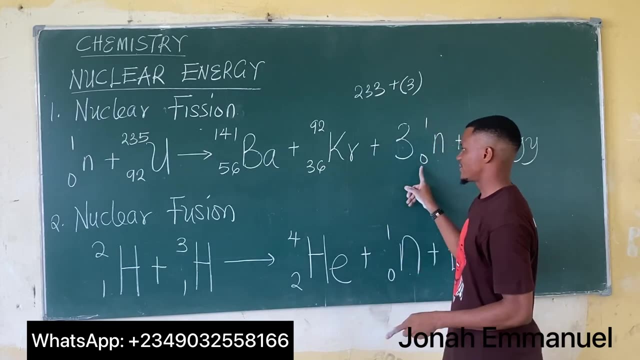 So this is how you can easily differentiate between nuclear fission and nuclear fusion. For nuclear fission, you have a bigger element with a higher mass number and a higher atomic number being split into several other elements with smaller atomic numbers. You can see here: 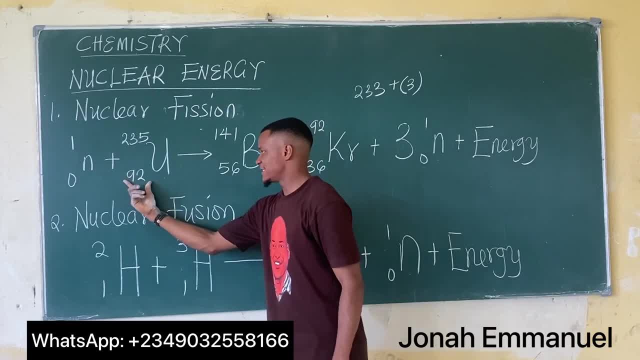 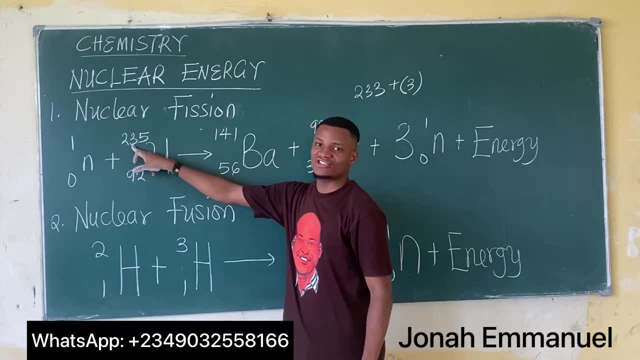 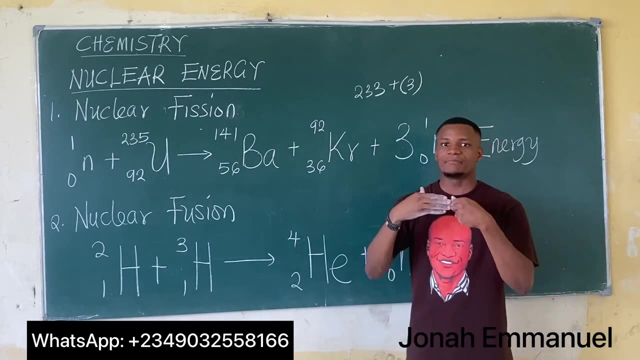 Smaller atomic number. So the larger atomic number is being split into other, the smaller atomic number. Same thing with mass: The element with the larger mass number is being split into other elements with smaller mass numbers. So it becomes a fission. Alright, 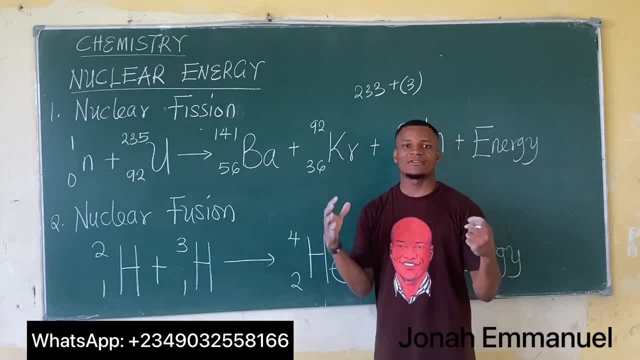 A breaking off. Alright, That's it. While for fusion, when something is being fused, it means it is being combined, So I have elements or isotopes with smaller mass number and smaller atomic numbers being combined to larger ones, As in this case. 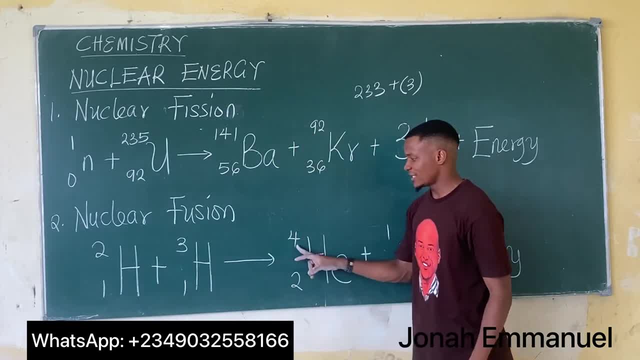 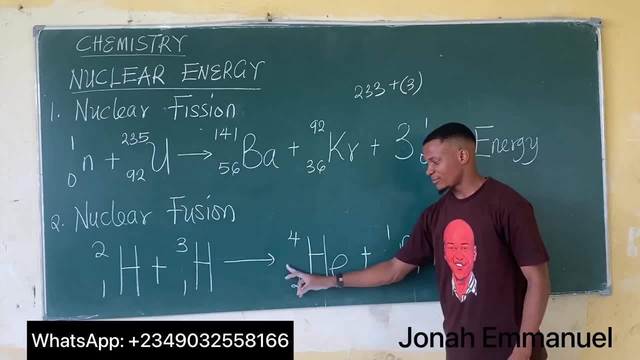 you can see the smaller ones- two and three- being combined to form the larger one, which is four, And also you can see the smaller atomic numbers which are being combined to form the larger atomic number, that's two. So how do I know? 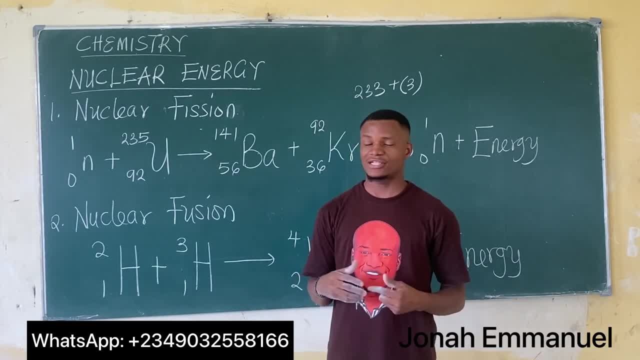 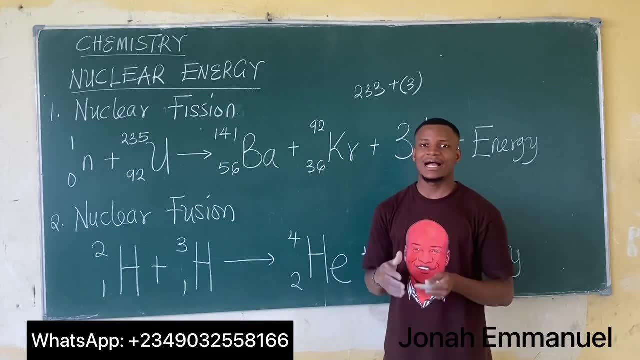 if it's a nuclear fission or a nuclear fusion reaction. Fusion reaction- Very simple. Look at the reaction very well. Where do I have the element with the larger atomic number and mass number? If it's at the reactant part, that's here. 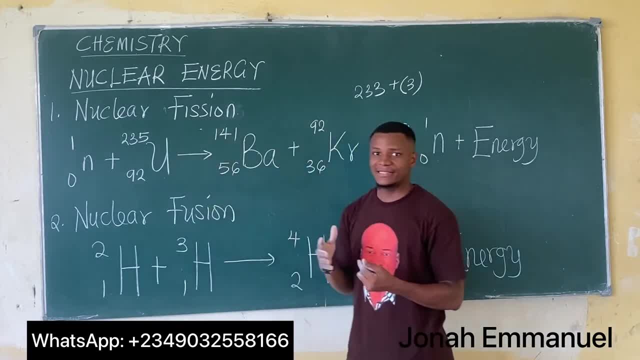 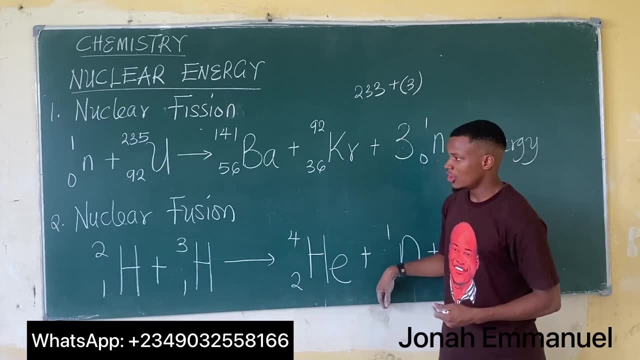 then it's a nuclear fission reaction. If the element with the larger atomic number and mass number is at the right hand side, or the product part or the product side of the reaction, then it becomes a nuclear fission reaction. So this is how you can. 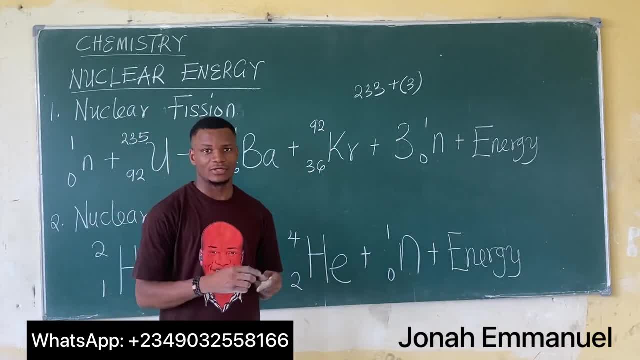 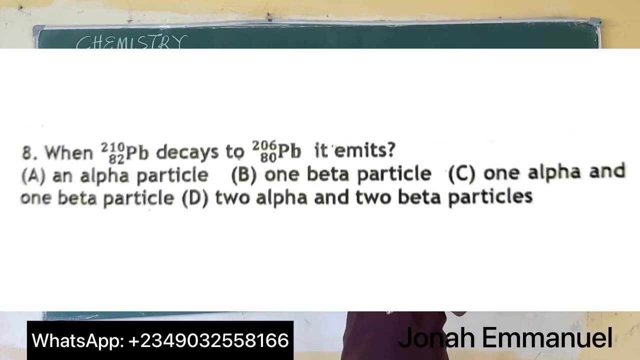 easily differentiate between a nuclear fission and a nuclear fission reaction. So we'll take some jump-pass questions and we'll start from here. So let's take the first question. It says: when Pb does lead, when lead-210 decays. 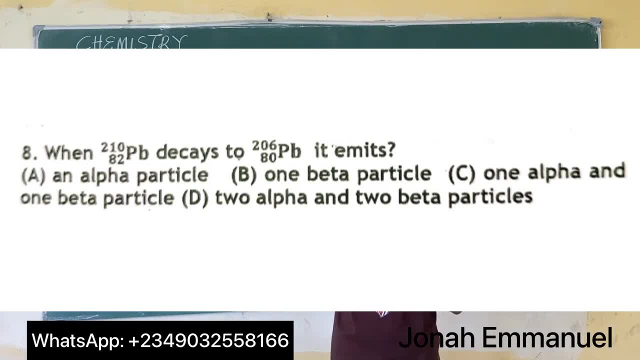 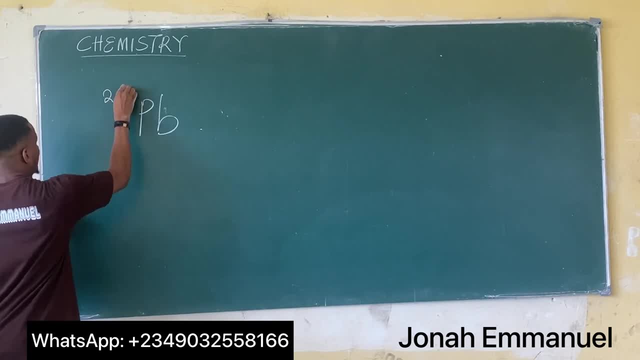 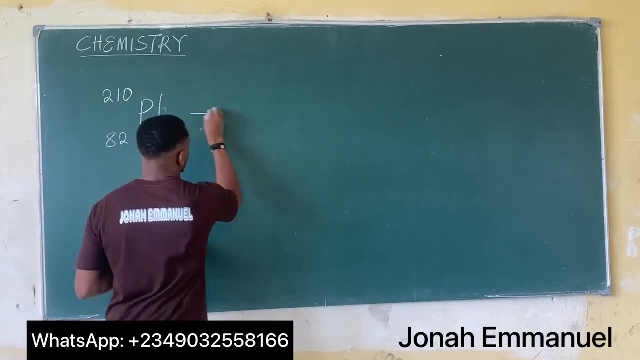 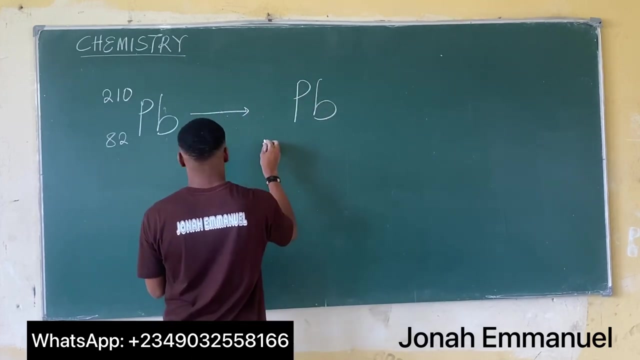 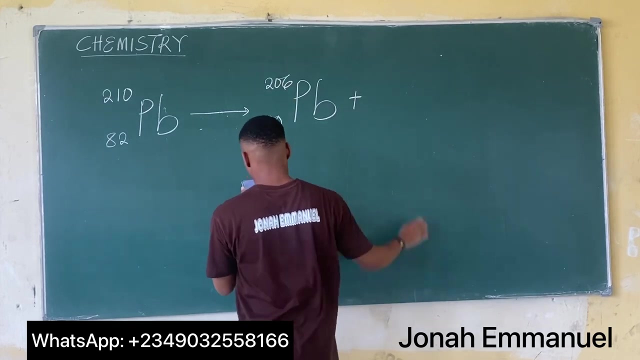 to form lead-206, it emits dash. So the concept is simple. I'm having lead-Pb-210 and, of course, 86, 82. It says this decays to form lead-8206.. It says it emits dash. 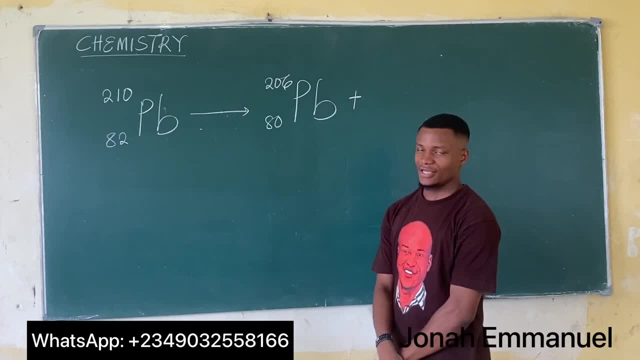 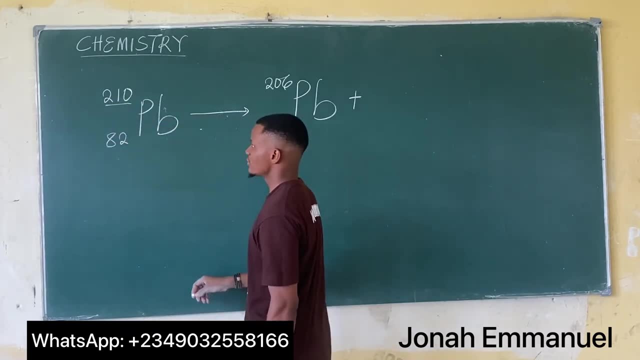 When it comes to emission, we know about alpha decay and beta decay. If I look at this, the difference here is that my mass number it had been reduced from 210 to 206.. That means this one here was got by subtracting 4 from here. 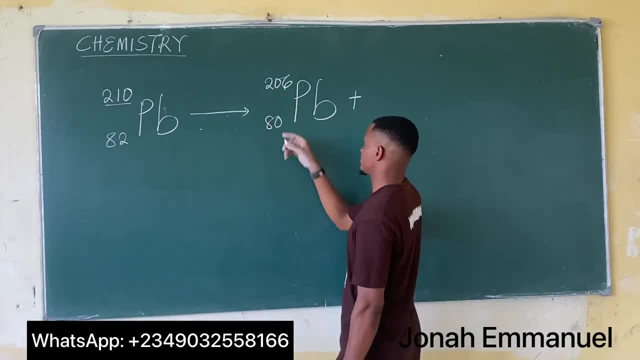 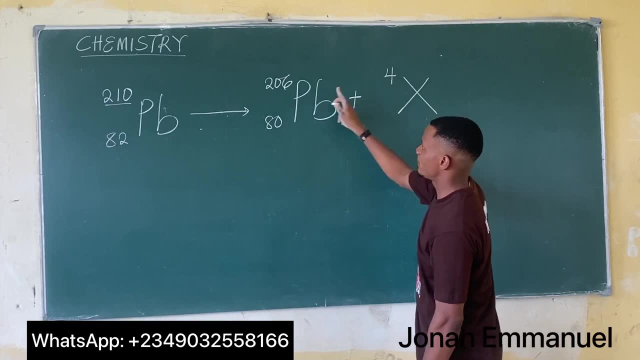 So 210 minus 4 gives us 206. So it has to be a particle such that here has to be 4, because 4 plus 206 gives you 210.. Also, I'm having 80 here, I'm having 82.. 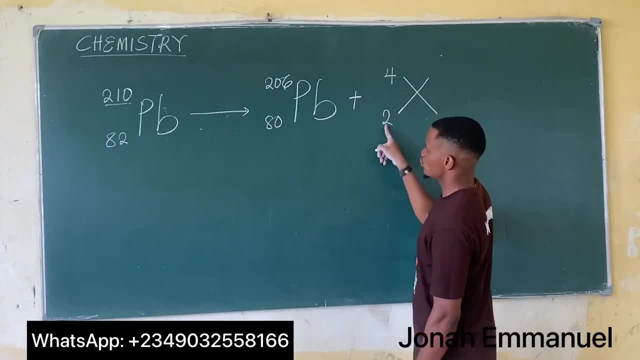 So here has to be 2, such that 2 plus 80 gives you 82., So that this becomes a balanced equation. And we know that the particle lines 4 and 2 is helium, So I'm having helium here instead, All right. 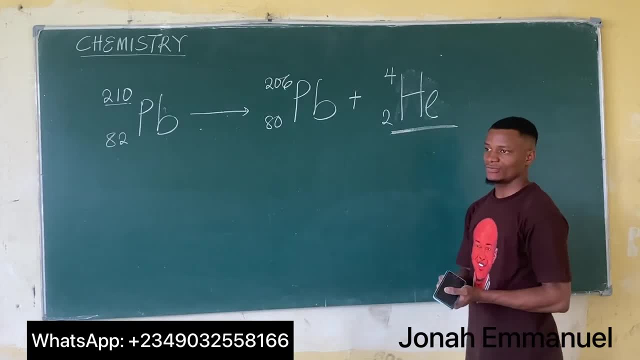 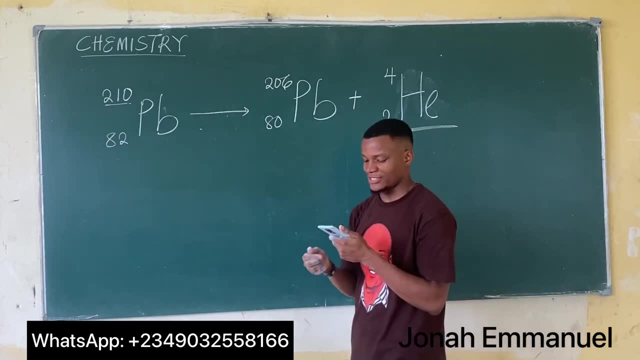 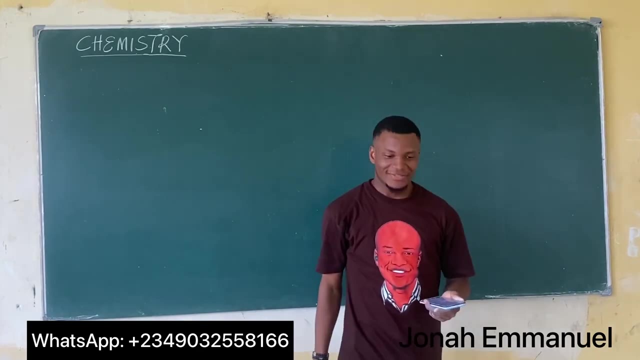 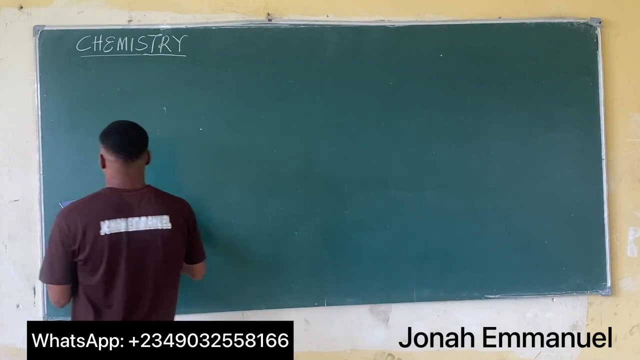 So the answer has to be one alpha particle, because we said helium or alpha particles are helium, All right. So it has to be one alpha particle. The answer there is option A, an alpha particle, All right. This question says the radioisotope uranium. 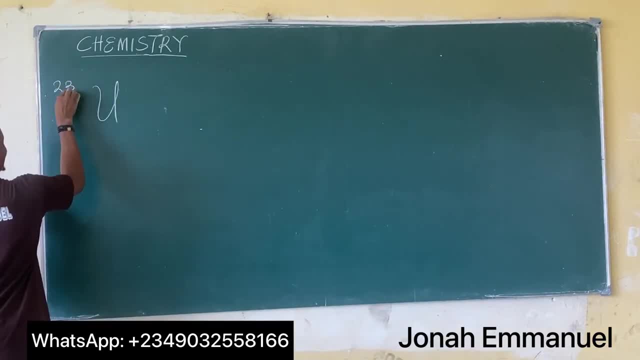 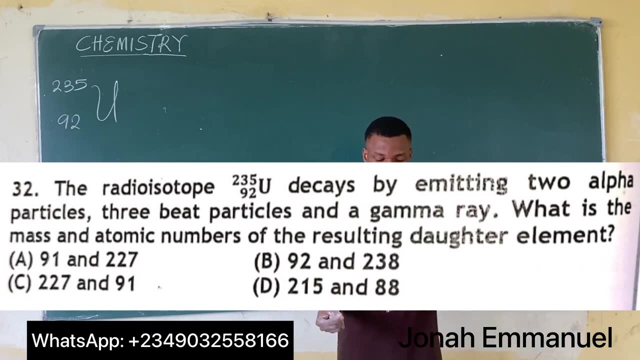 uranium-235 having atomic combined magnitude 2 decays by emitting two alpha particles- three that should be beta, not bit- three beta particles and a gamma ray. What is the mass and atomic number of the resulting delta elements? All right, Let's get this done. 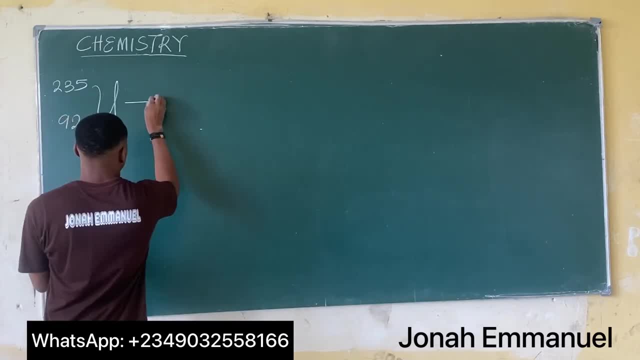 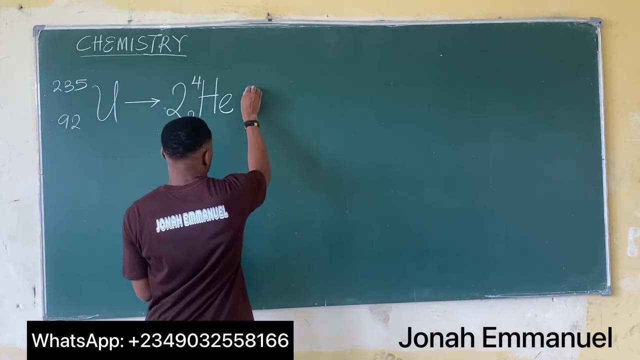 I'm having uranium-235.. We said it's undergoing a decay. okay, so decomposition reaction. They said two alpha particles, So two alpha particles are helium, HD2 and 4.. And also three beta particles, So three beta particles are electrons. 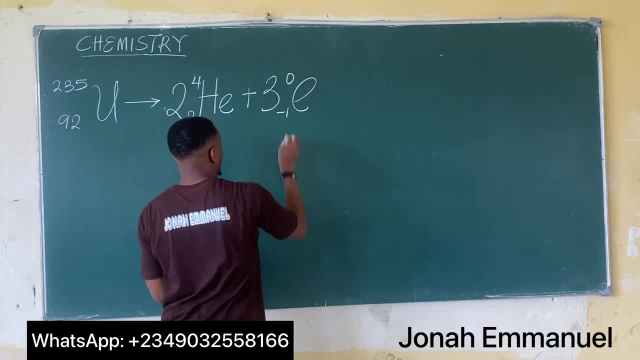 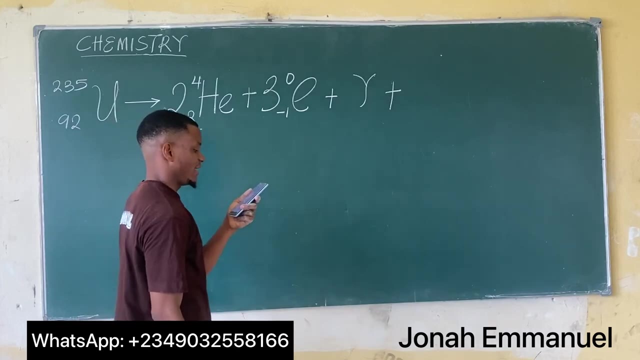 So electron minus one and zero plus, and they said a gamma ray. Gamma is just this, There's no repetition. They said plus What is the delta element? or what is the atomic number and mass number? Okay, It says mass number and atomic number. 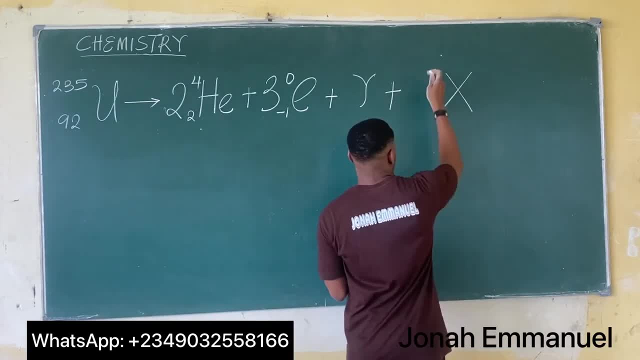 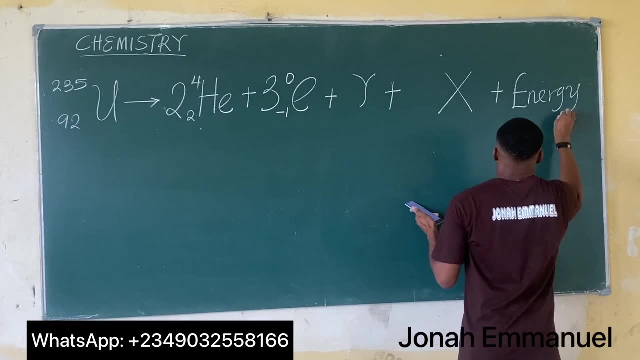 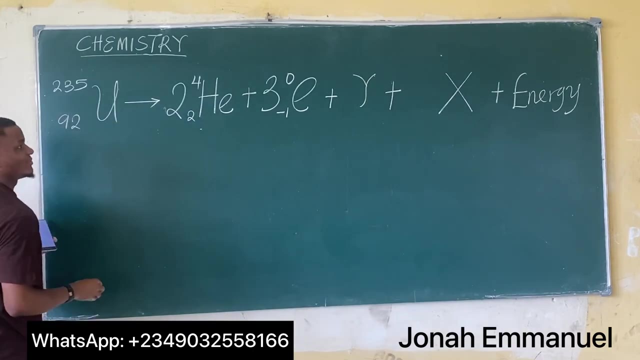 or the delta element. So delta element here, Mass number here, Atomic number here, Obviously, plus Very important Nuclear energy. So let's get the phases here. So how do I get this? So maybe for this let's look at mass number first. 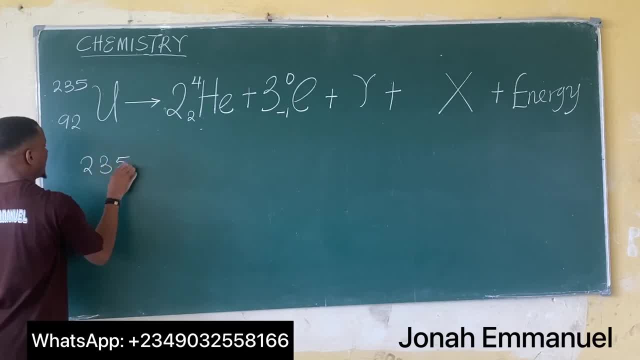 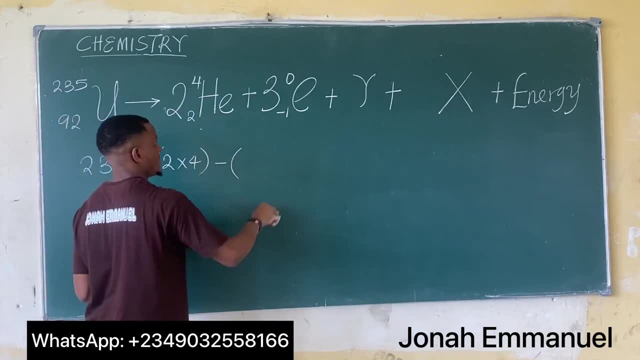 Here becomes 235.. So 235 minus That becomes two times four. So two times four minus That becomes three times zero. That's three times zero. This one does not really affect it, So I'm having. this is equal to. 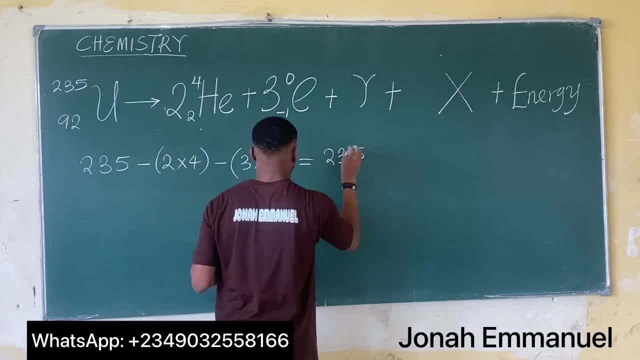 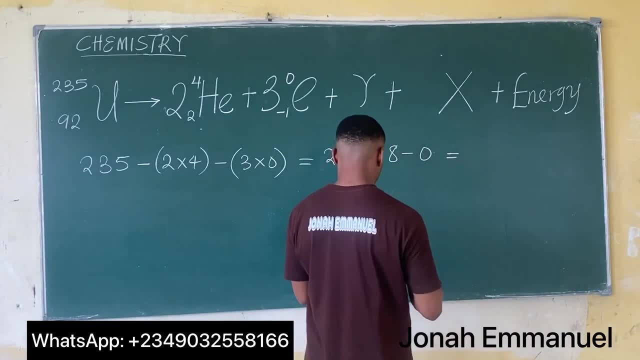 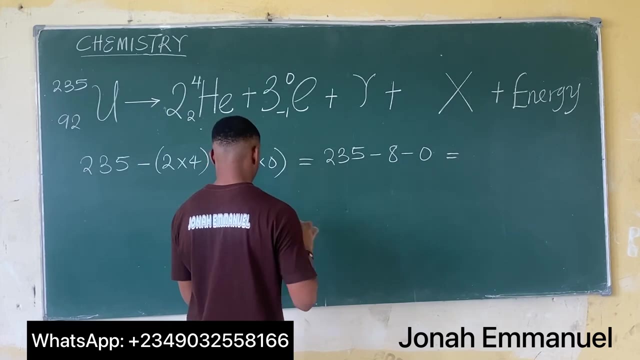 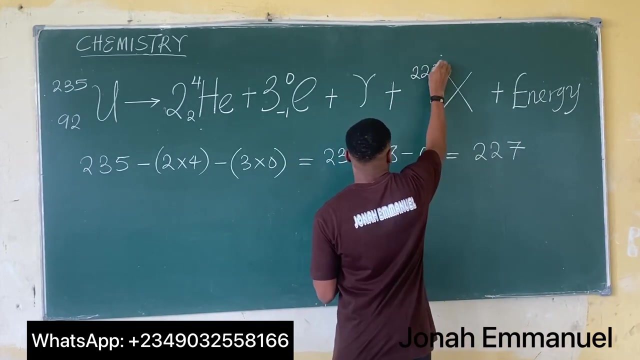 I'm having 235 minus eight minus zero, And that's equal to. I'm having 235 minus eight minus zero And just about 227.. That means the mass number again is 227.. I'm done with this. Let's get atomic number. 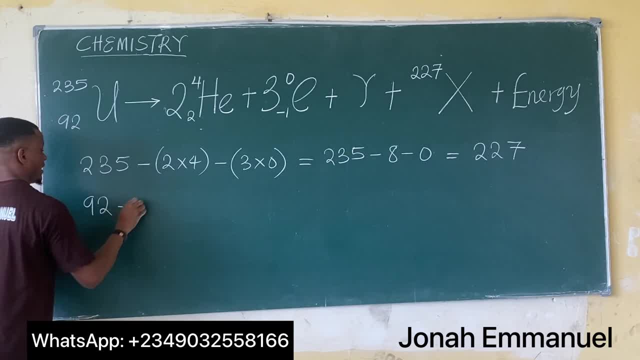 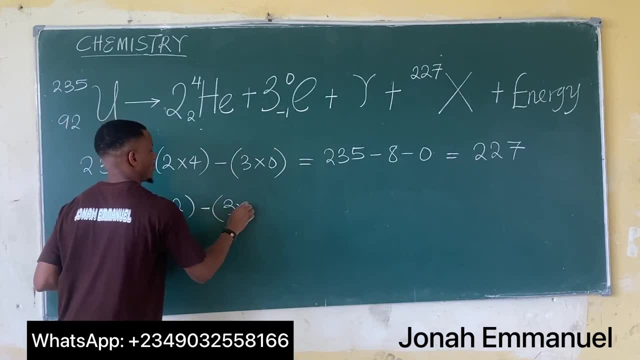 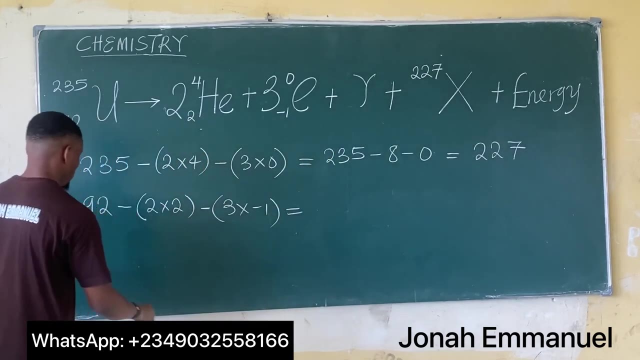 This becomes 92.. Minus two times two, Minus three times minus one Minus. So it has an effect. So let's go. It's equal to. So I'm having 92 here, So it gives me 92.. 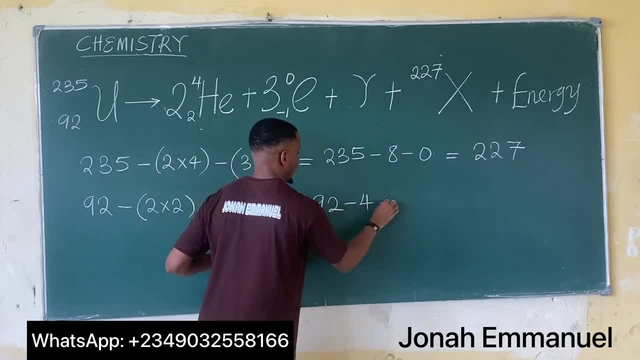 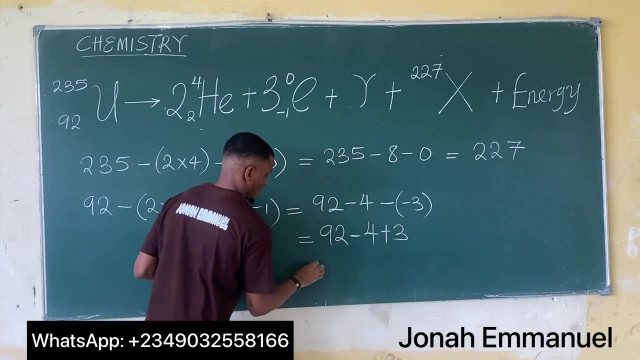 Minus two times two is four, So minus four. Minus Three times minus one is minus three, So I'm having minus three And this is now equal to 92 minus four. Minus minus is plus three. This is equal to. 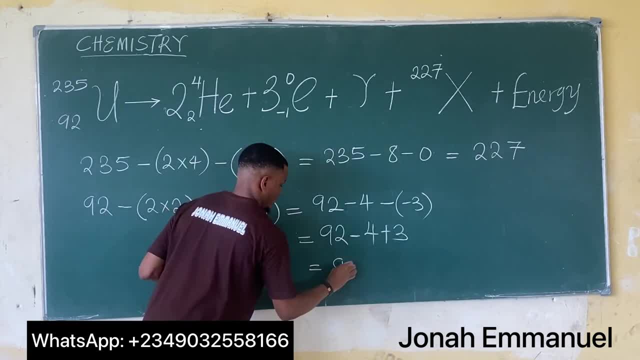 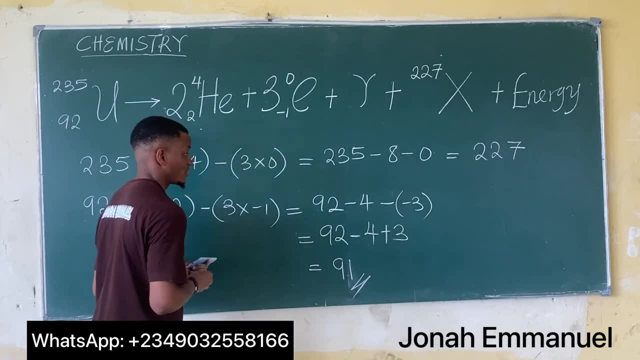 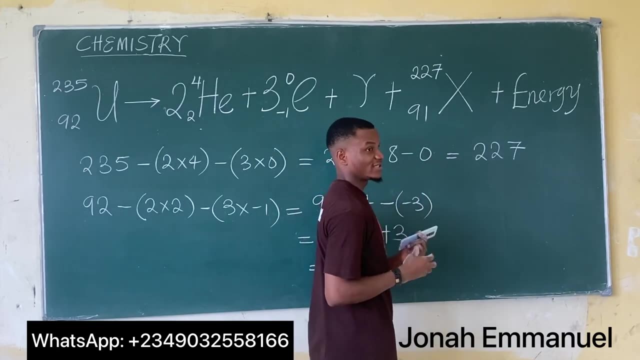 This will give you minus one, And here that should give you 91. That should give you 91.. So 92 minus four plus three gives 91. So I'm having here as 91. It means that the dot element is an element such that the atomic number is 91.. 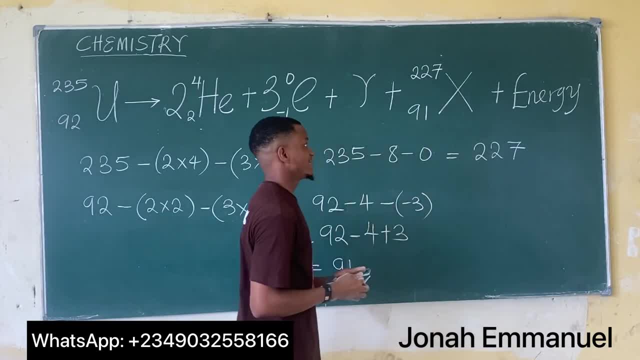 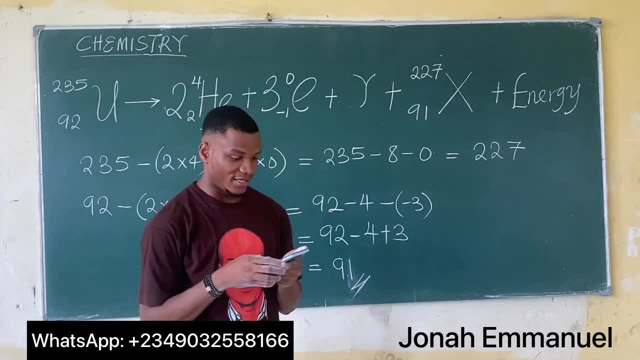 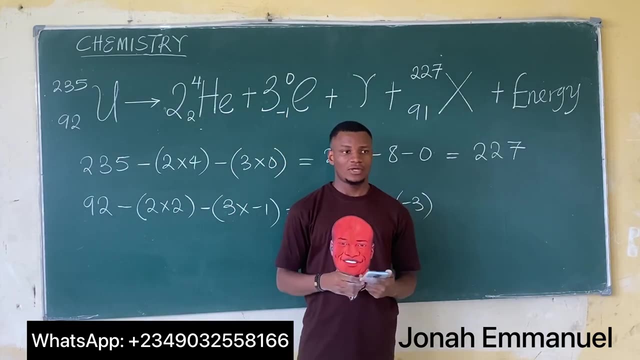 And the mass number is 227. So that is the dot element. So hence the answer is 227 for mass number and 91 for atomic number, And that is option C, 227 and 91.. By the way, the element which atomic number 91 is called. 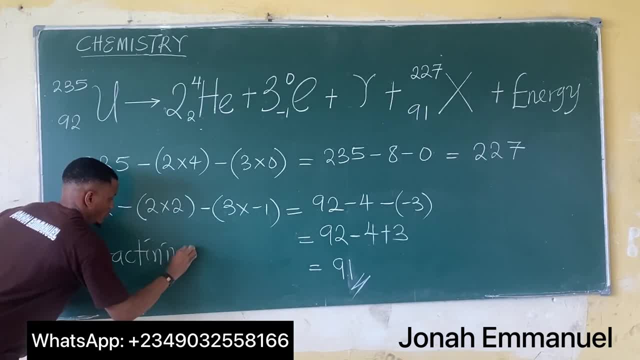 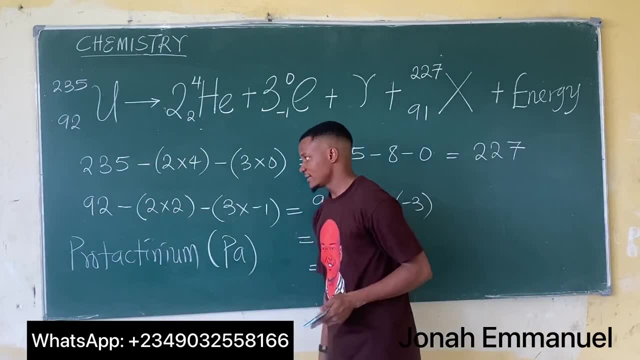 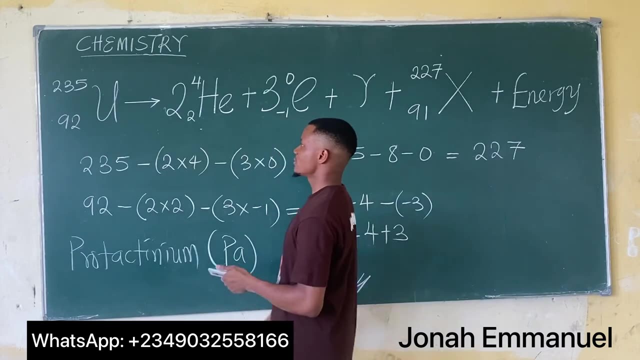 Protactinium. Protactinium is PA. It has a symbol. Alright, That's PA. This is an element which has atomic number 91. So you can see, uranium 235 undergoes with the activity K To produce two particles of alpha or two alpha particles. 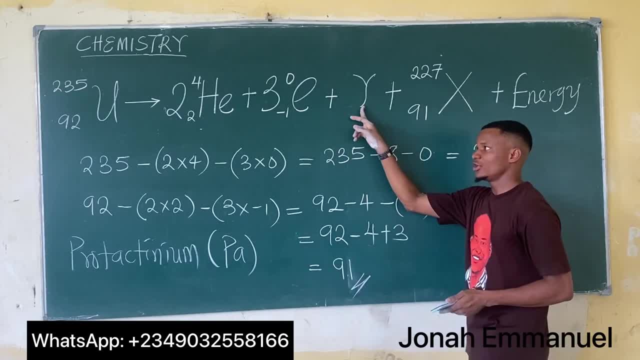 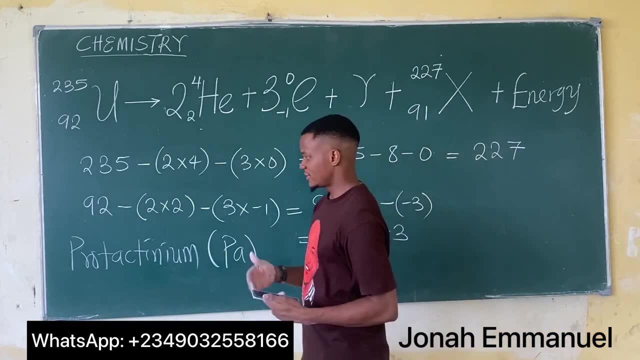 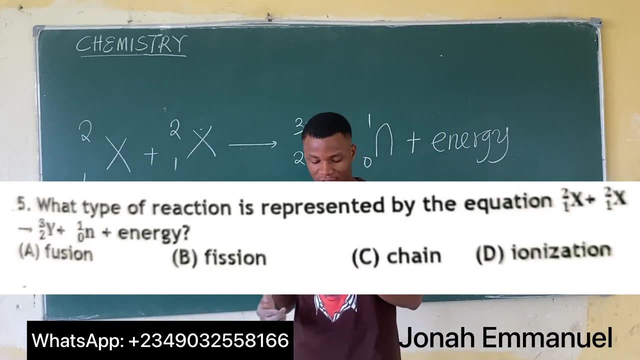 Three beta particles And a gamma ray to produce protactinium 227.. Alright, So this is how we solve this particular question. Alright, So this question says What type of reaction is represented by the equation of this. Alright, You have fusion. 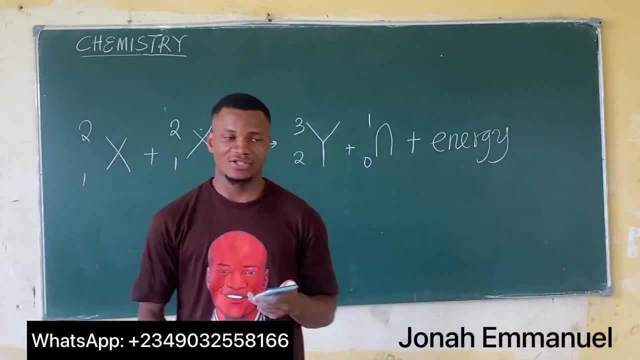 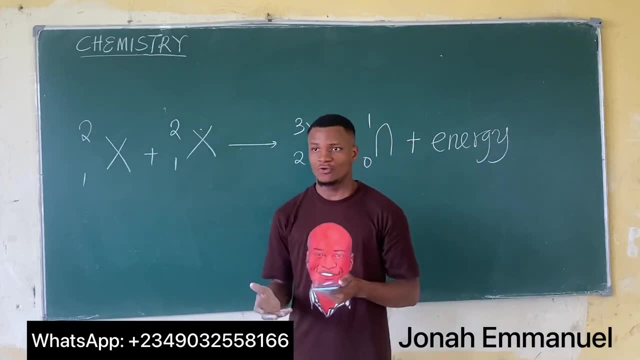 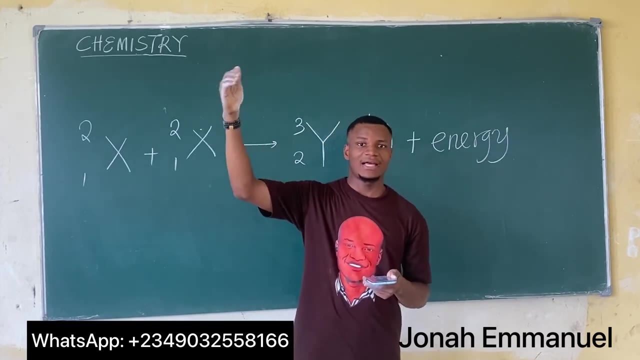 You have fission, You have change, You have ionization. So what's the answer there? Now? we've said before It's easy to differentiate between nuclear fission and nuclear fusion. We said for fission You have the particle or the element with the greater atomic number and mass number. 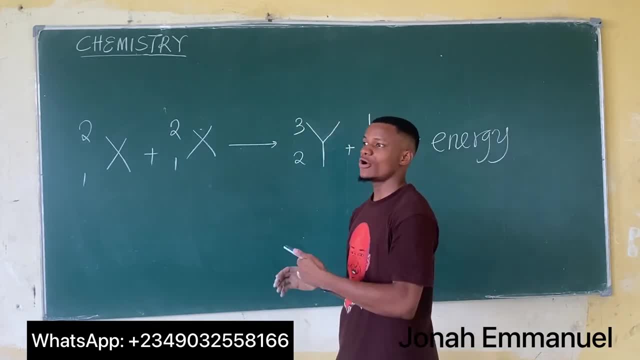 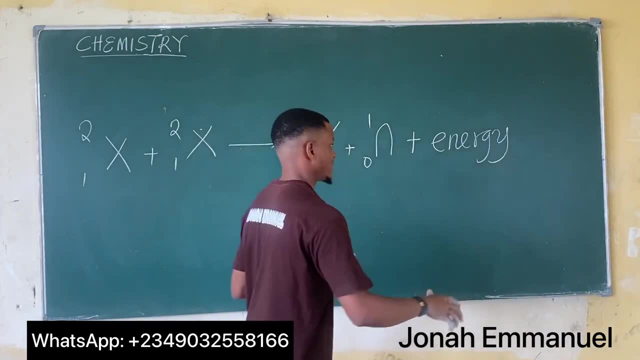 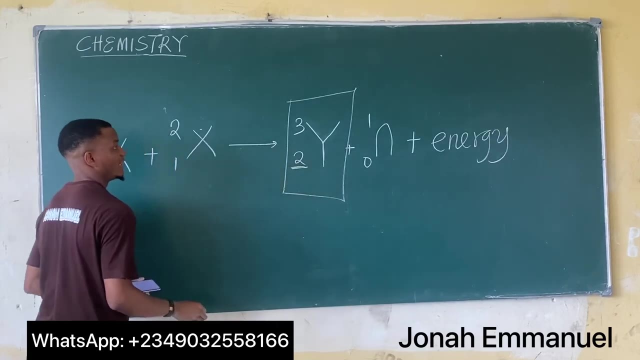 For fission, You have it on your left hand side. Why, for fusion, You have that element on your right hand side. If I look at this equation here, This is the element That has the greater atomic number And the greater mass number. 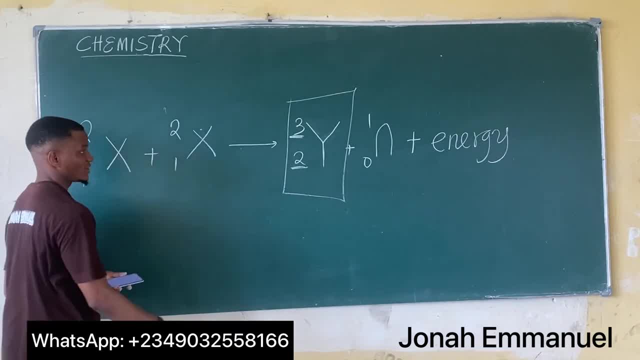 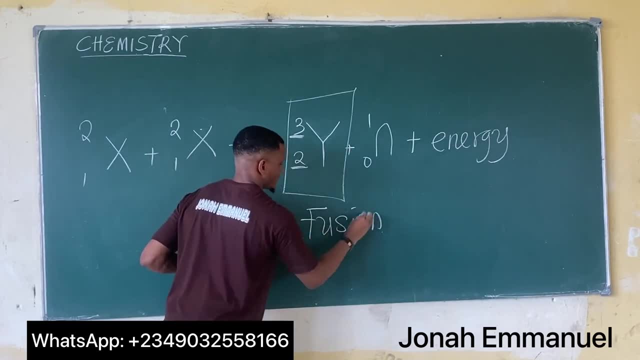 As compared to any of these here. So since this element is found on the right hand side, This becomes a nuclear fusion reaction. So the answer is fusion, Because the element with the greater atomic number and mass number Is on the right hand side of the equation. 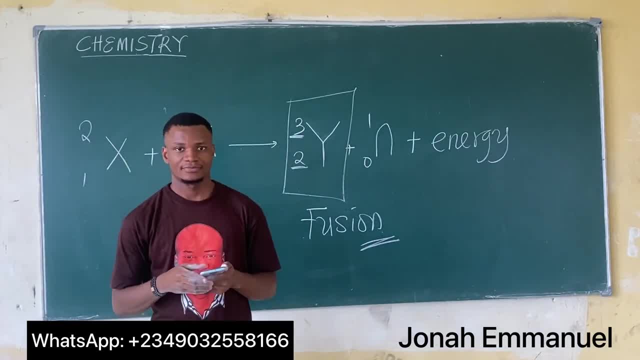 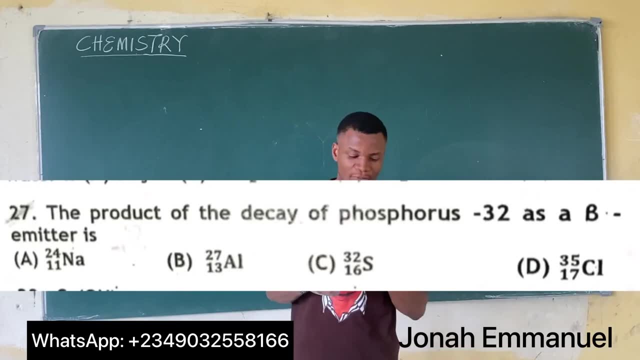 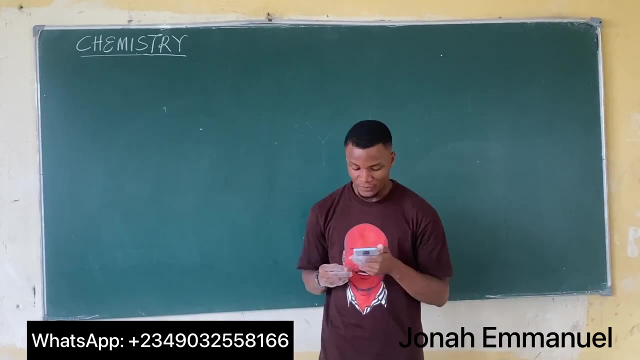 So that becomes option A Fusion, Alright. Let's look at one last question on reactivity. Now, this question says: The product of the decay of phosphorus 32.. As a beta emitter is dash Alright, So let's get this done. 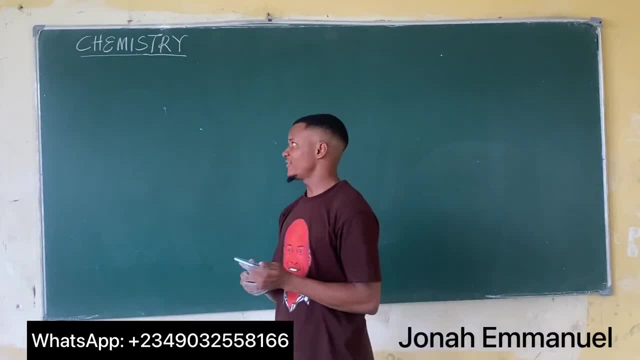 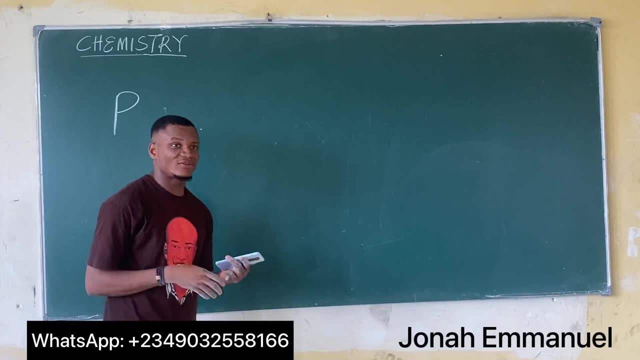 Okay, So let's get this done, please. So observe that The given element here Is phosphorus. Now, if I want to say Phosphorus 32. It means that the mass number is 32.. That's 32 there. 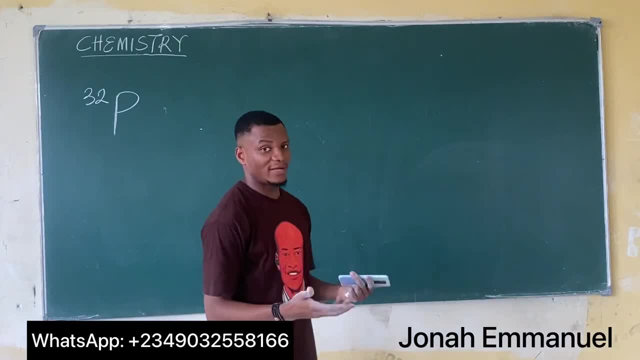 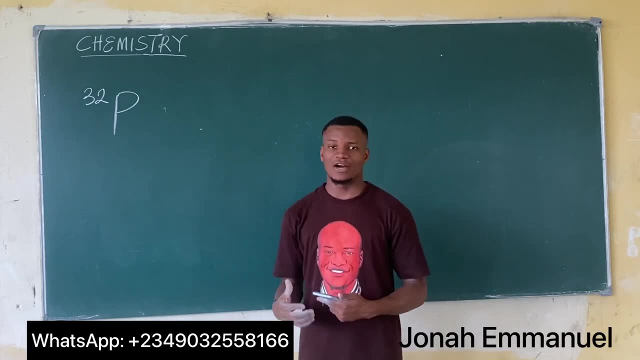 Now observe: You were not given the atomic number Because you are assuming that you should know. Alright, You are assuming that you should know The atomic number of phosphorus, Which, of course, is atomic number 15.. So I have 15 there. 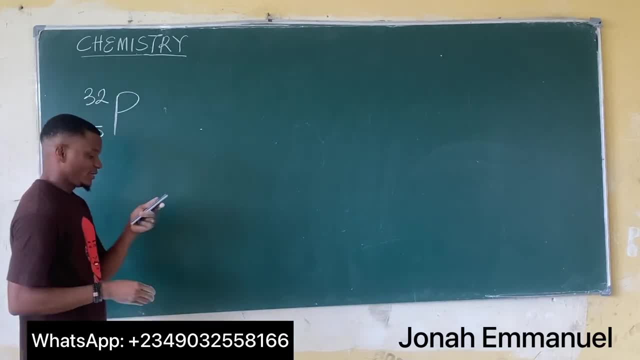 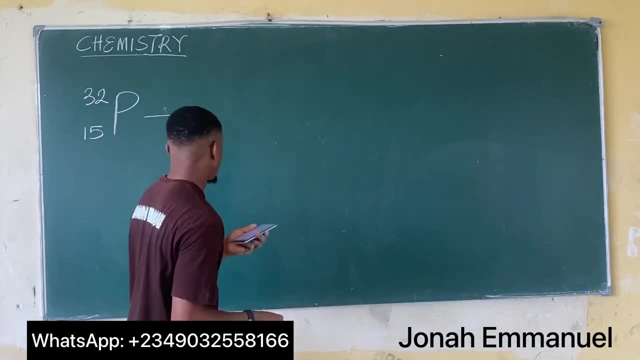 As the atomic number, They said It's undergoing a decay. So this Of A beta emitter, Okay, It becomes Beta emitter, That's electron Minus one. And dash, They said A beta emitter, That's just one. 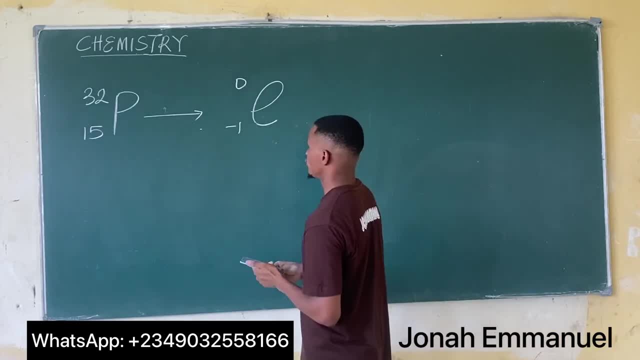 Alright. So what is the Product? So plus All I have. We said For beta decay That the mass number Is the same thing, So 32.. Why For the atomic number? We said It will increase by one. 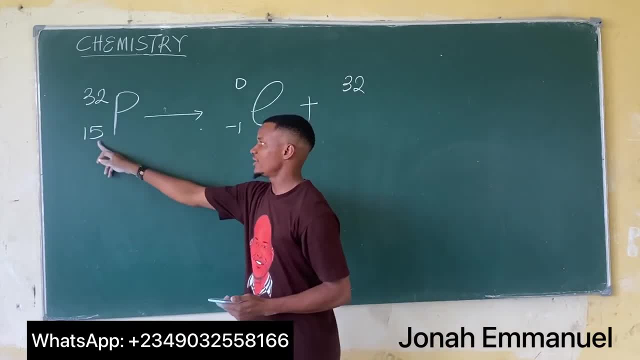 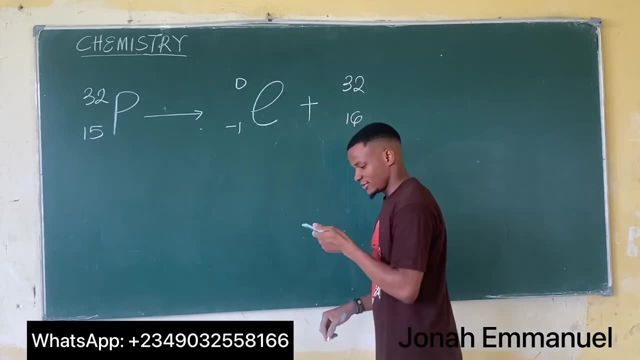 Alright, It becomes 15.. Minus, Minus one, That becomes 15 plus one, That is 16.. Alright, So I'm having 32, 16. That, of course, Is Soft form. I'm having 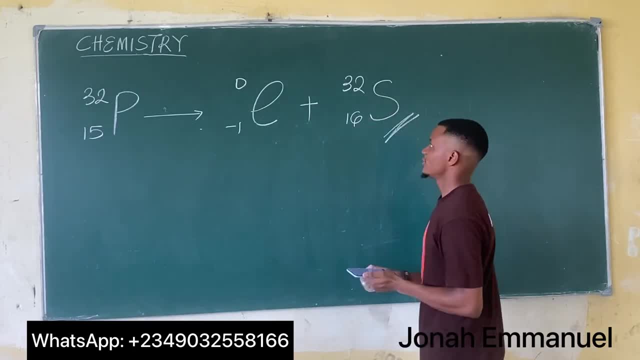 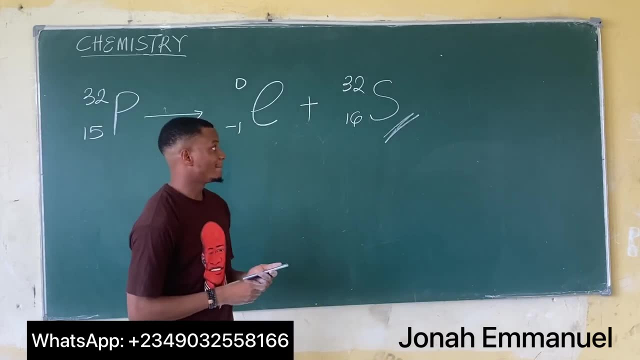 Soft form As the answer. So Soft form 32. With atomic number 16. Becomes The answer: Alright. So that's how you get Um This Question. That's how you answer this question. 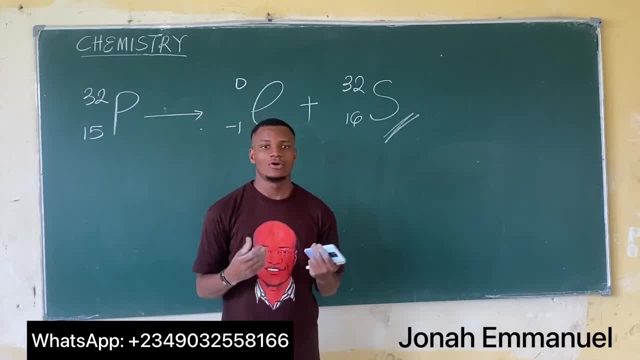 Alright, So that's the last Um Thing For This, Our class On Reactivity, But before we go, I'll give you One more Um, You have this, You have this reaction: Sodium 23..